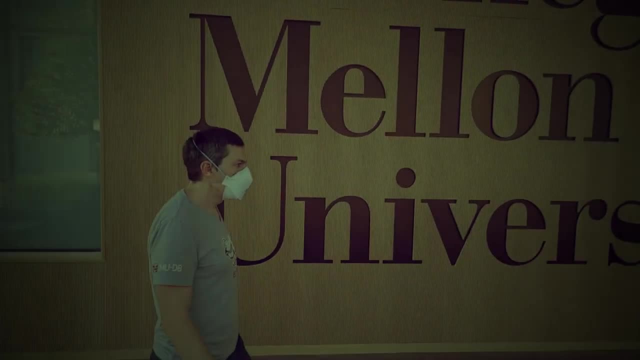 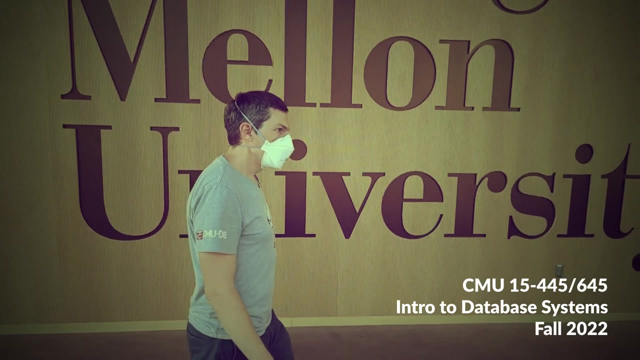 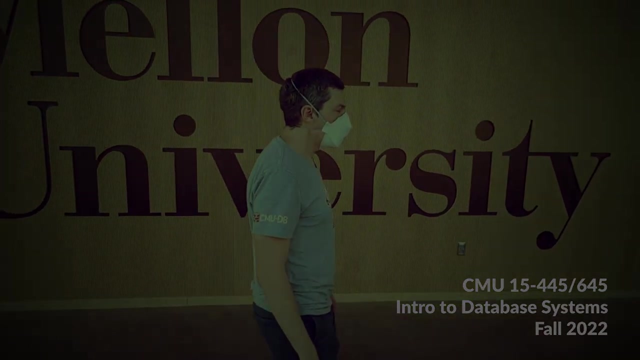 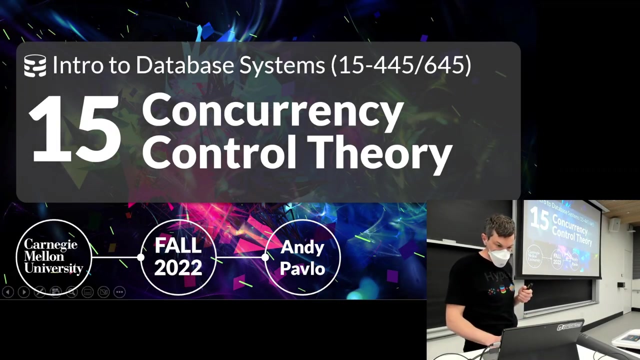 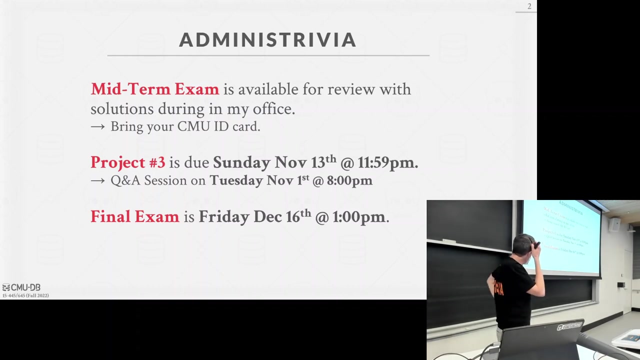 All right. so he's dealing with his lawyer. That's his problem. Let's jump into this for you guys. So again, midterm exam will be available in my office for review during my office hours tomorrow. Please bring your CME ID. Project 3 went out this week on Tuesday and that'll be due. 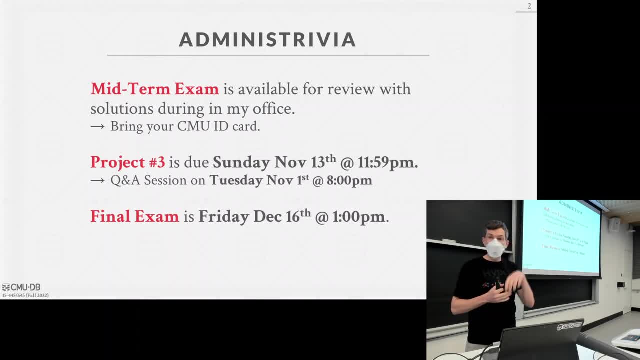 November 13th, which is a Sunday. I'll announce on Piazza. but we'll have the Q&A session next Tuesday at 8 pm over Zoom, And again, the slides and recording will be available afterwards. And then they've announced the final exam. It's Friday, December 16th at 1 pm. Please do not book. 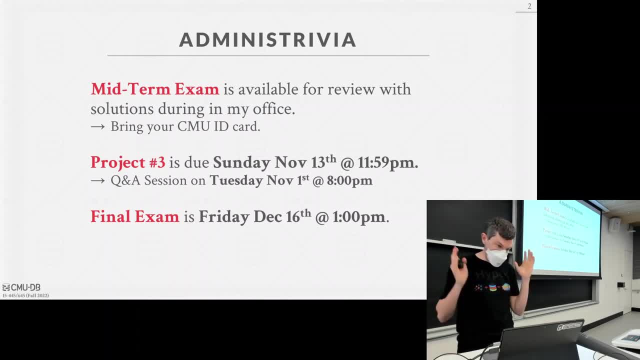 a flight prior to this. right, This will be in person. Okay, yes, Is the final exam cover like the second half or just the second half? The question is: does the final exam cover like overall, everything or just the second half? 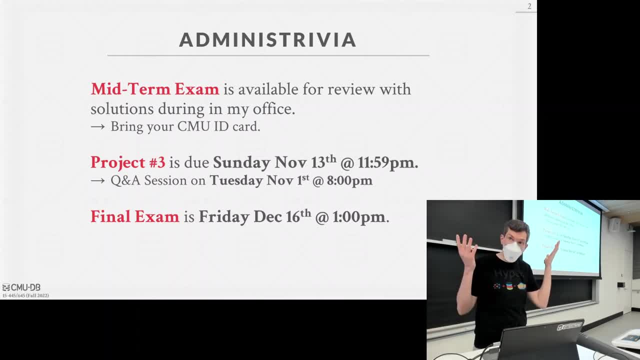 It will be focused on the second half. but, like again, if you forget SQL and you can't do SQL, that's your problem. So would the length be a three-hour exam or would it just be a five-hour exam? 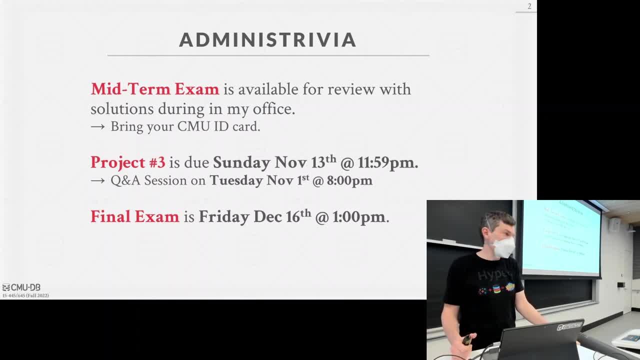 It'll be like. it'll be like it'll be like the midterm. Yeah, yeah, yes, No, but like just to like follow up on that, like you'll maybe ask like: 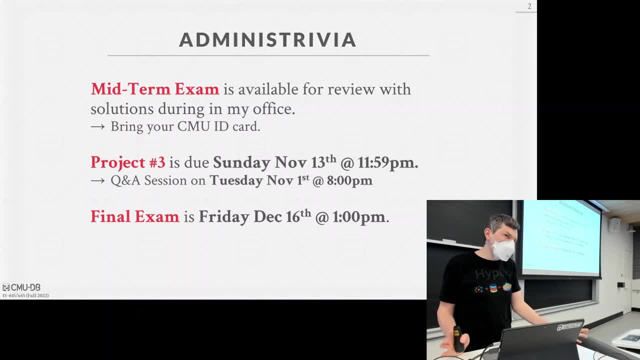 more like obscure stuff from like the first half. I wouldn't call anything I'm doing in this class obscure, but uh, no, it'll, it'll be. it'll be focused on the um, it'll be focused on the, on the, the material. 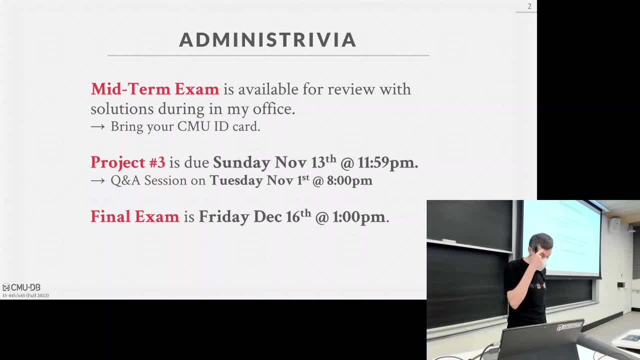 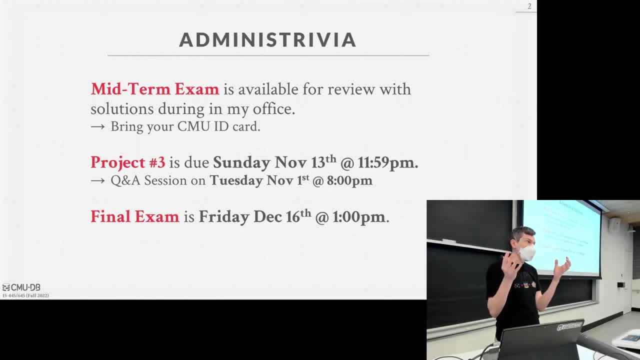 set up right. It's when I say like it'll cover everything again. if you, if you forget SQL, if you can have a buffer manager that works, you'll have problems. So don't do that. Yes. 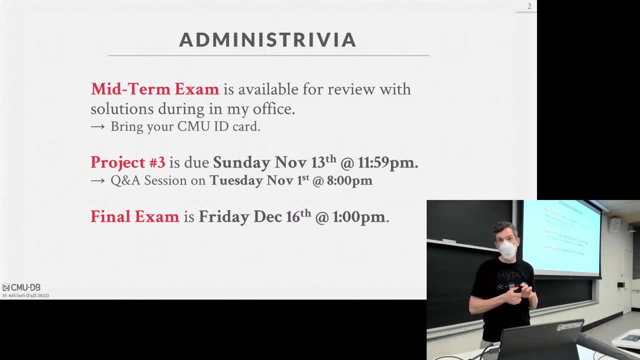 So is that like um the midterm? So in terms of that, is it, is this a three-hour slot? So are you given the three hours, or is it one and a half hours? I don't know how other, I don't know how other classes do it. It'll be a, you know it'll be. 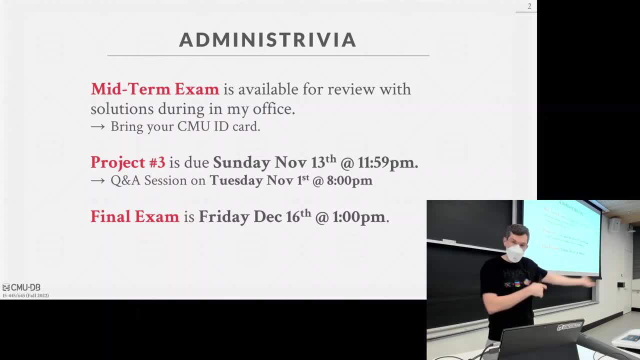 the same length and complexity of like the midterm. If you want to save the whole entire three hours, you go ahead and do it. some people do, we'll get coffee and donuts and for people, whatever. what do we want? okay, he said no, okay. 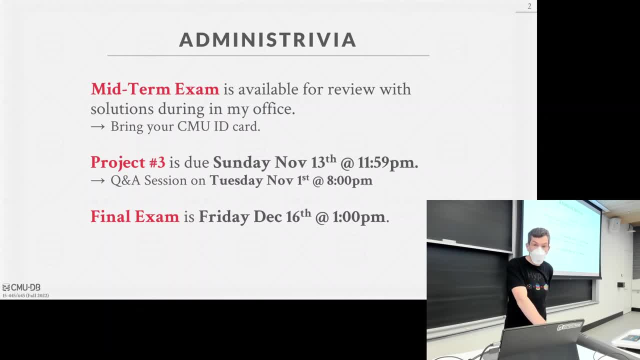 no, i don't get fired. no, i think, uh, i just don't know the answer to that. uh, okay, i can't get fired. right, i have a, i have a child. i gotta pay child support, like i can't. that's what he's gotta deal with. um, all right, so okay. 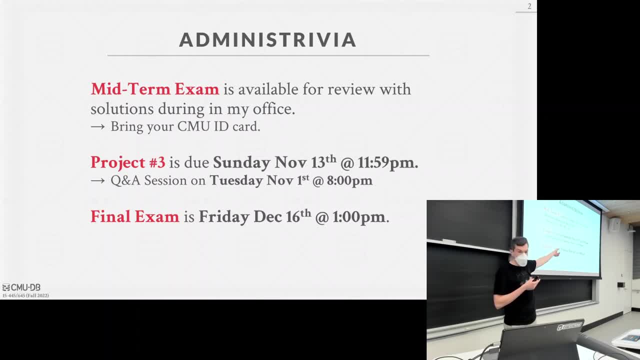 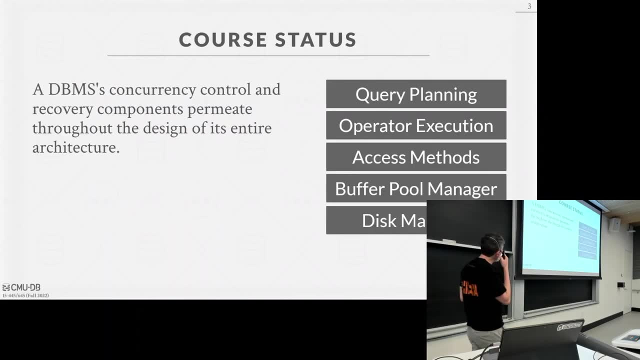 we'll have more, more information. i'm just saying, hey, we have a date, we have a time, we have a location. please don't book a flight before this, okay, all right. so, uh, at this point now in the semester, we've we've reached the summit, we've reached the top right, we started off. man the. 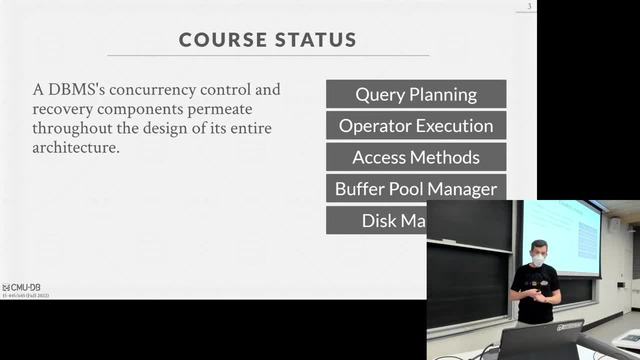 disk manager and we worked our way up to these different layers. and now we, you know, now we know how to take a sql query, you know, and convert it to a query plan, execute it, let it read some data, write some data at the disk, and so forth. right, so so. 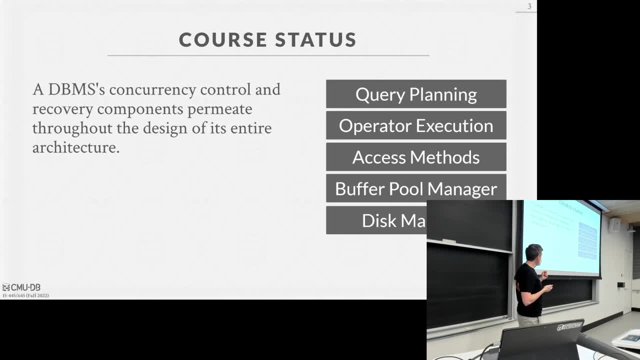 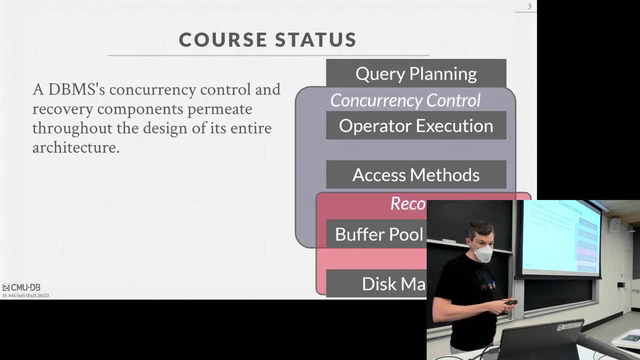 now what we're going to talk about going forward for the next two or three weeks is sort of coming back down and looking at a bunch of other parts of the system now in the context of concurrency, control and recovery and the reason why we covered this after we've sort of gone. 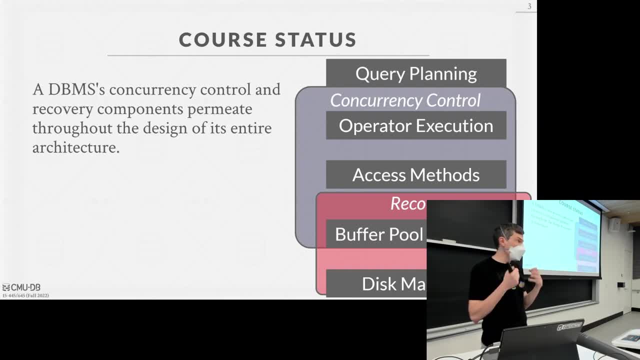 through all the layers is that this concept of concurrency, control and and the the protection mechanisms we would have for recovery and other things. these are going to be all intertwined with all the different parts of the system, and so it's for it just sort of makes it easier to go through. 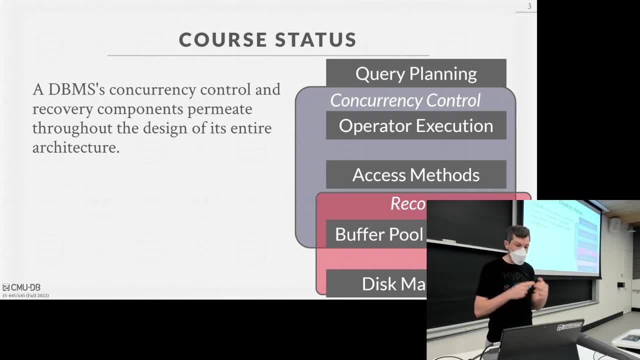 these things without worrying about these extra stuff we're talking about now. uh, because now you understand the basic concept of, like, you know what a powerful manager does, so now we can say: okay, how do we make it uh work, and you know, and make sure that the changes we write to disk are recoverable. 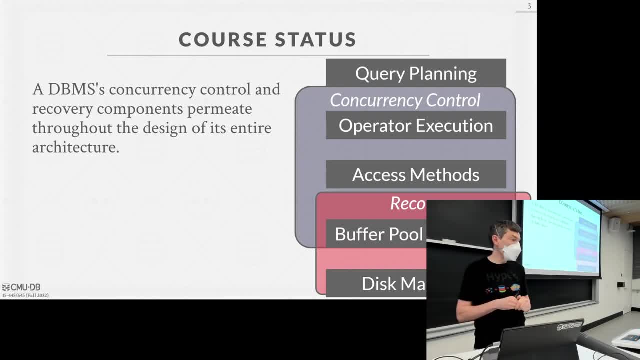 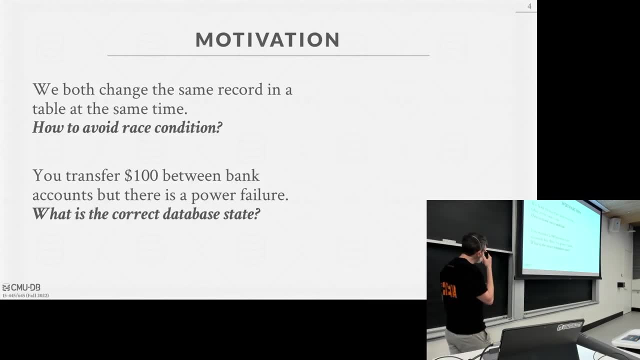 uh, or durable, and how to make sure that transactions can run safely, uh, protect, protecting themselves from each other. okay, all right. so to get this motivated, on talking about concurrency troll, i want to come up sort of two basic scenarios here, two sort of obvious things. right, and so say we? 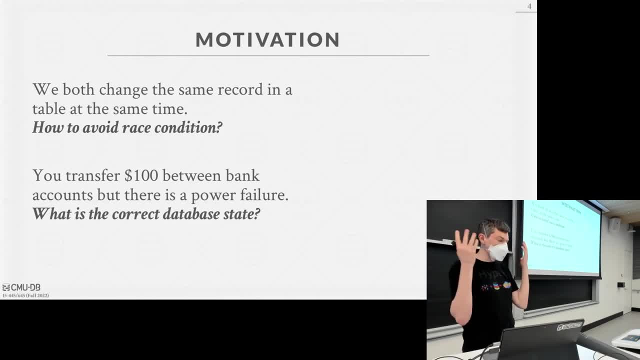 have an application that's recording some your financial status, your bank account, right. so let's say we have a case where we have two threads or two, two, two application uh programs running the same time and they issue queries at the exact same time. that will update the same record in the same 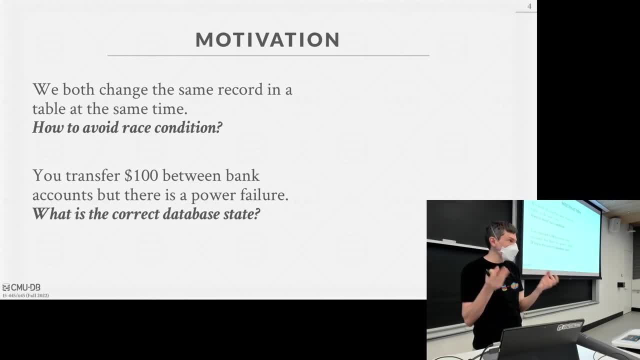 table right. so how are we going to make sure that we avoid a race condition to not have, you know, some weird torn rights or some uncorrupted database state? let's say there's another scenario where we i'm taking a hundred dollars out of my account, i'm putting it to another account, but in between 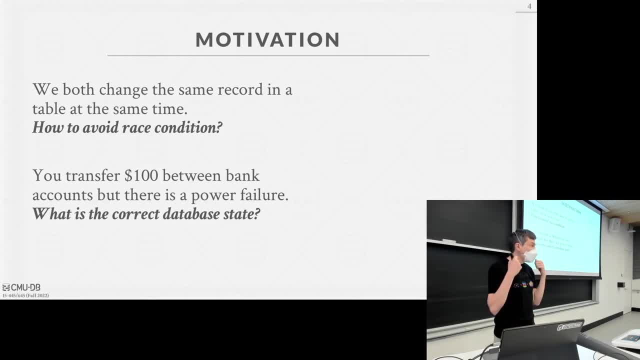 the time i take the hundred dollars out of my account before i put in the other account. there's now a power failure, the the. you know the building is struck by lightning or something. the machine loses power. uh, and this, the name system crashes when we come back what should be the correct state. 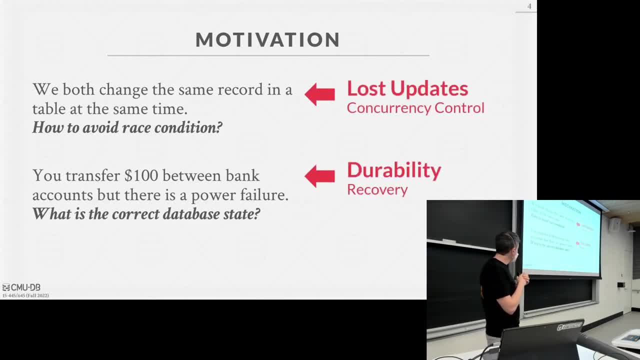 right, so the the first example is what's called a loss update, right, how are we going to deal with two threads trying or two- i don't say threads or two- two queries trying to right to the same thing at the same time? uh, and it doesn't have to be a record that can. 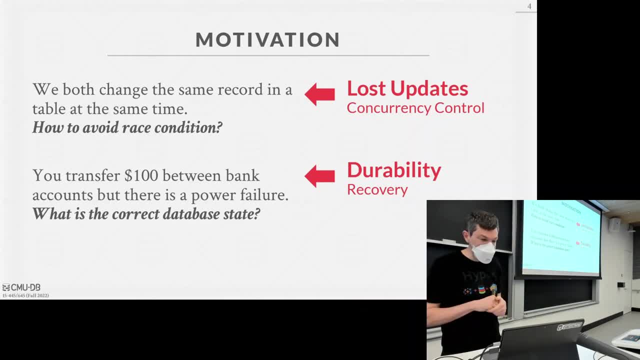 write to the same table at the same time, even the same database. we can have different levels of granularity, uh, but we're going to protect the, the system is going to protect itself from these problems using concurrency control, which we'll talk about for the next uh, three or four. 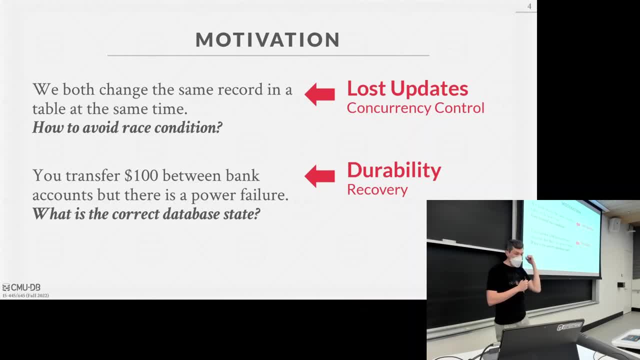 classes. and then the second problem here of how do we make sure that we don't lose anything. uh, when there's a failure, that's going to be in the context of recovery mechanisms, which we'll cover after concurrent control. again, these things are intertwined as we'll see, as we're 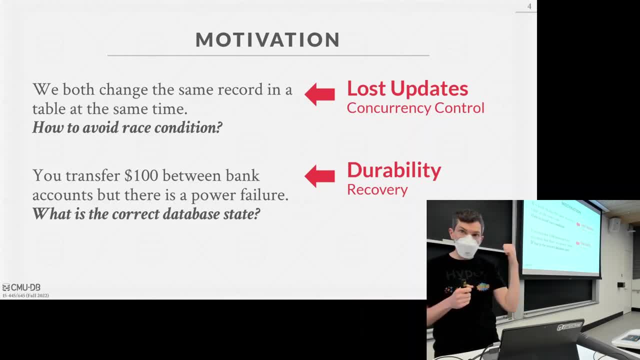 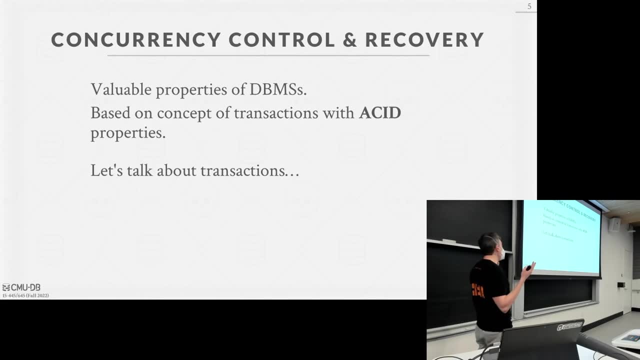 throughout today, but i'm going to really focus on the the loss update, the first problem. uh, for the next two lectures or three lectures, all right. so it's sort of obvious why you need these things, or why you want these protection mechanisms. right, this is what the advantage. 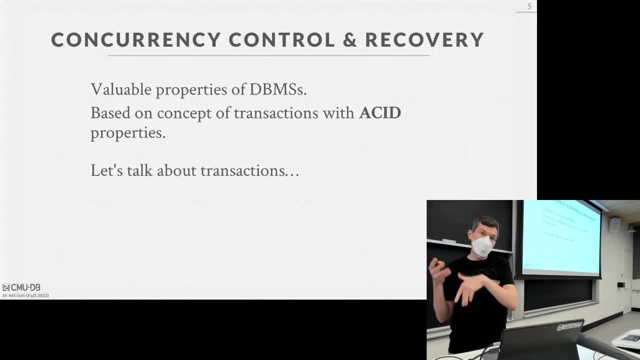 you're going to get using a database management system over you trying to go. you know, go off the rails and write your own, you know data manager right in your application, right? i think if you're a new startup, you're trying to get your, your application out the door and so people start. 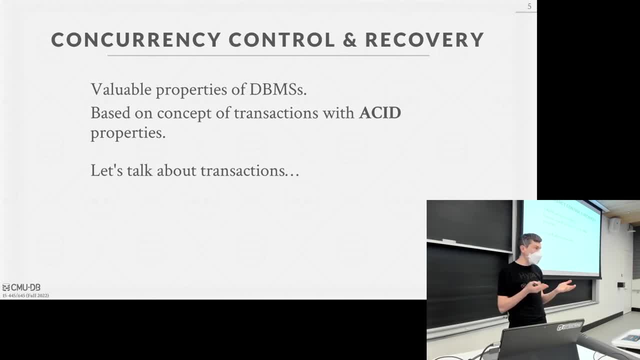 using it so you make money. you don't want your developers spending time writing all this concurrency control stuff and recovery mechanism stuff like the. the fact your application doesn't lose data when you crash is not a differentiating factor from your application versus your competitors, so why are you going to spend your time writing this stuff? you're going to let the database system 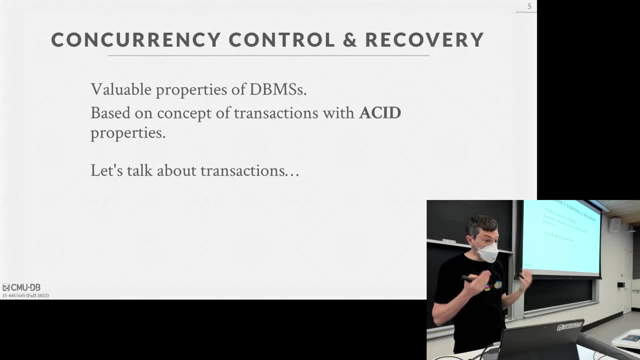 do this for you, all right, and they're obviously going to do a much better, better job than you possibly could. so the core concept that we're going to have to have these protection mechanisms, that reason about what does it mean for the system actually? correctly, it'll be in the context of this. 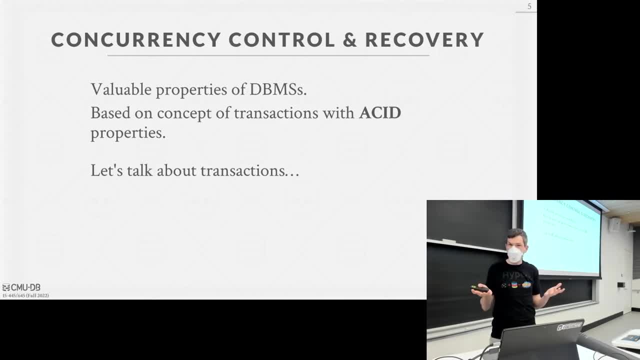 acronym called acid. quick show hands. who here has heard acid before? all right, actually not bad, good, excellent, good. so we'll go through each of these uh one by one and we'll see. uh, it's actually more than previous years, so that's very good. um, we'll go through that. you know the. 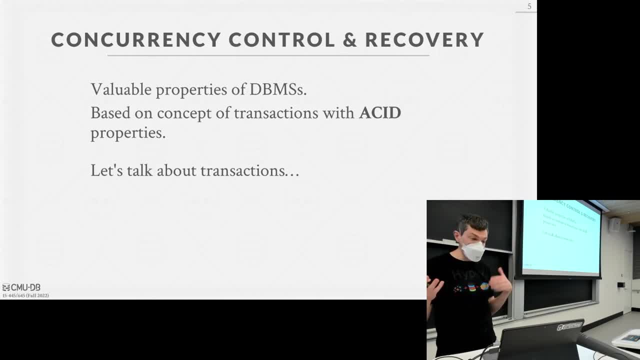 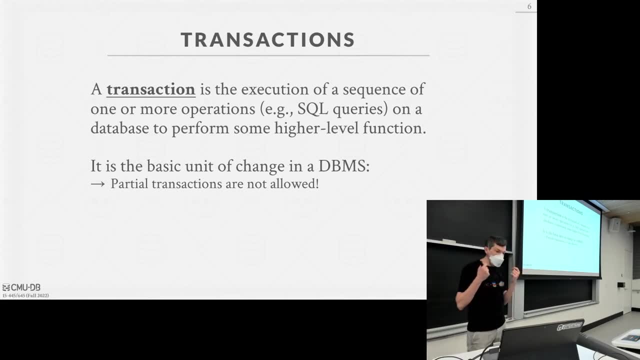 acid what they all mean and talk about how the system would implement the mechanism to protect them. but first we need to find what a transaction is. so the transaction is going to be a, a, an execution of a one or more operations. uh, in our case there will be sql queries, but we'll 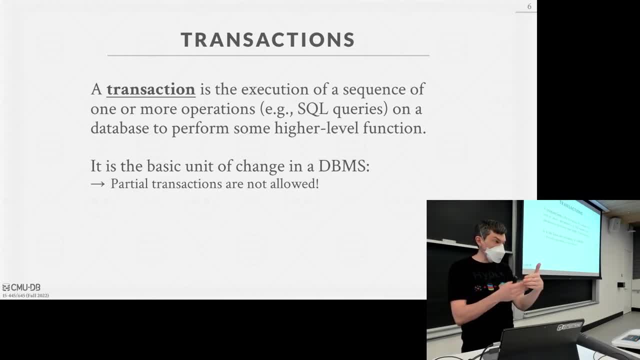 see how today it's going to be from the database system's perspective. it's going to see just read and write operations, but it's going to be these, these, these operations going to execute, to perform some higher level task or function in our application. so my example of like taking 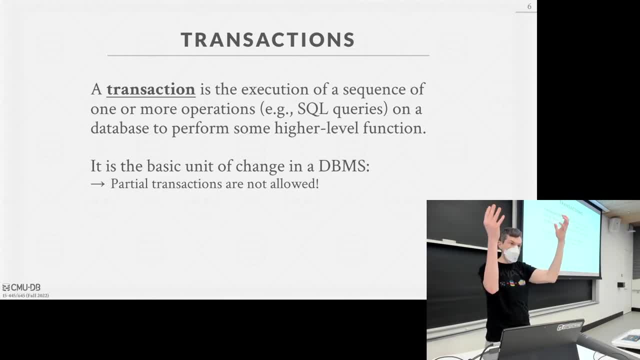 money out of my account and putting it to my bookies account right. those the the first step of taking the money out and then putting into the other account that those two together are- are a transaction right. it's. it's the thing that the, the application, is trying to do to. 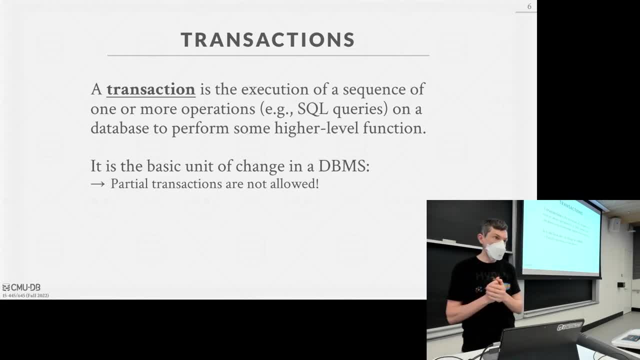 achieve some state change in our database that it reflects some aspect of the real world or something that occurred in the real world. so the transaction is going to be a basic unit of change in our database system and the key idea here is that we just we're not going to be allowed to have 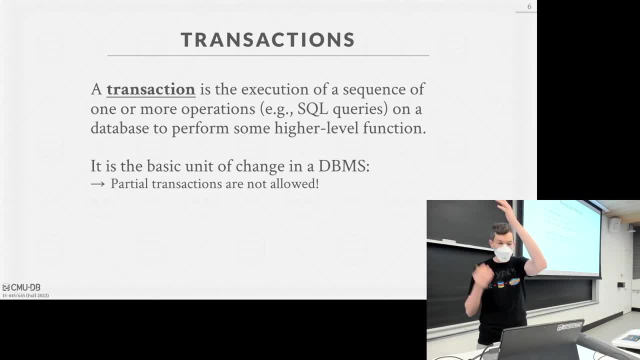 partial transactions. so i can't do. if i want to do, take money on my account, that's a right. take them and put the money in this account, that's another right. i might just go ahead and collect it all the way because some array changes because of uh running, but but then you know if the ako and and phлоx are utility eat. they're all monkeys and so i figured i didn't think it was like it and that's the reason that i saw if you, if you can actually implement this, it's in my business. i understand that you've got to. 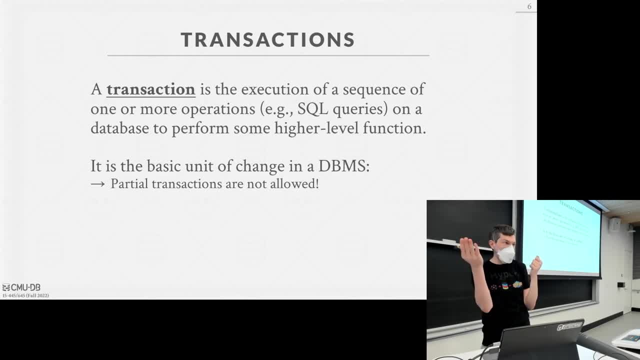 my transaction can't do only one of them, right? I can't take the money out and then not up to the other. I can't up the other without taking the money out, right? We'll simply say if that, if I can't do all of them, 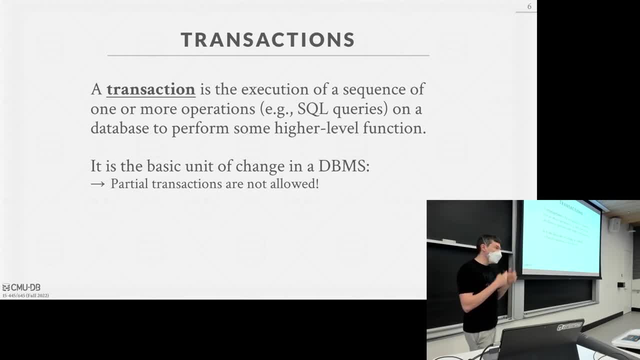 then I'm going to do none of them. Now you say: oh well, what about if I have a one operation, you know? I mean, if it's doing one operation without, that's by itself, well, that's a one operation transaction. 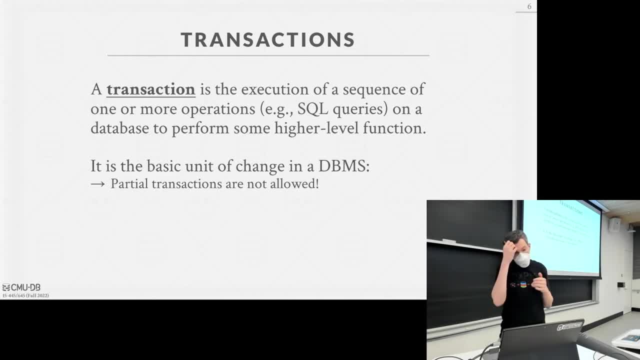 That's still a transaction And there'll be some other interesting things that'll come out of that, Because you know, you can obviously have a single SQL query and a transaction by itself, but it can update multiple records right. So again going back to my example here, 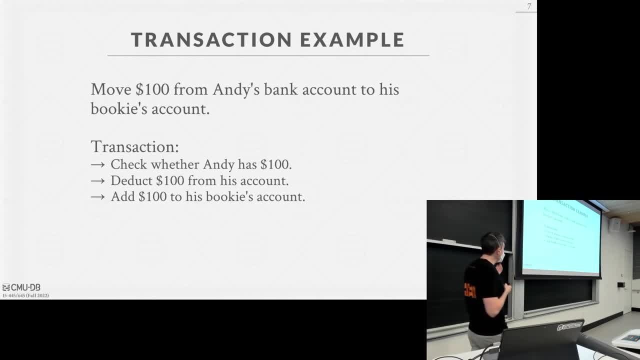 I'm taking the money out of my account, putting it in my bookie's account. The transaction we would define is would be these three steps. Obviously, we do a lookup, a read into my bank account to see whether I have $100, probably don't. 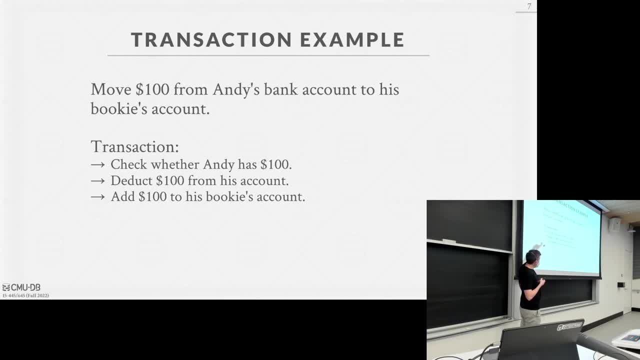 And then we'll deduct the $100 from my account and then we'll add it to the bookie's account. Now you can imagine other checks being done in here. like you know, is my account closed or open? Is the bookie account? 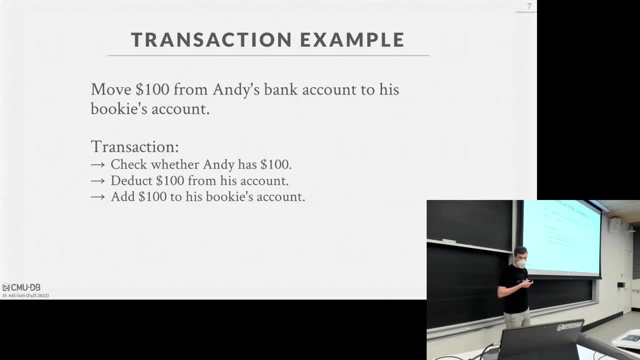 Like: is it flagged for fraud or something like that. There's a bunch of extra stuff you actually would do here, but for our purposes it's three steps, And so the right operation is the deduction and then the addition. These have to occur together. 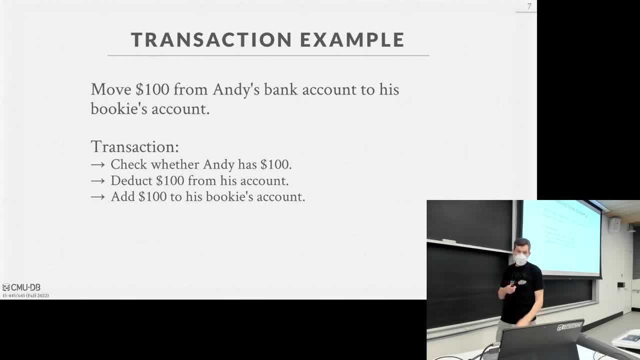 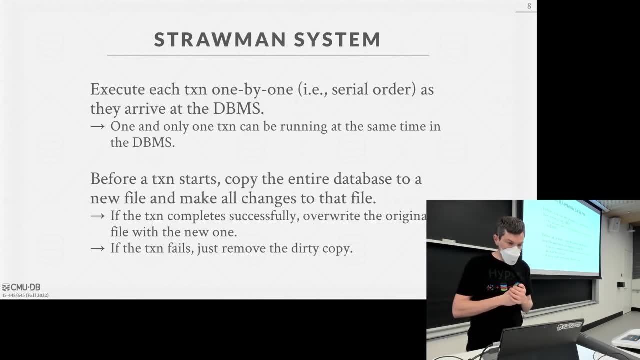 or none of this is going to occur. Okay, So let's look at a straw man system, how we could actually implement, you know, a database system to support this. And so let's say, now we make a single-threaded database system. 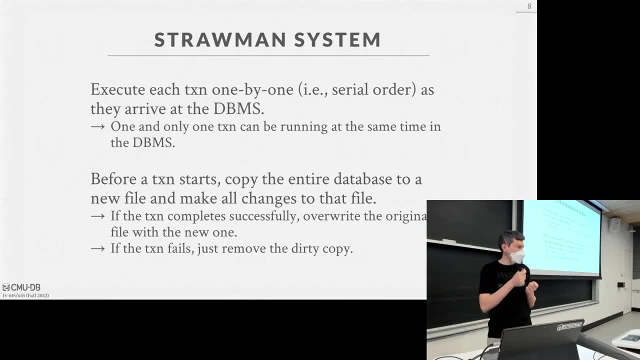 that's going to only execute a single-threaded database system And then we're going to have transactions one after another in serial order. So that means that, like if I have, like, multiple applications trying to submit a bunch of transaction requests. 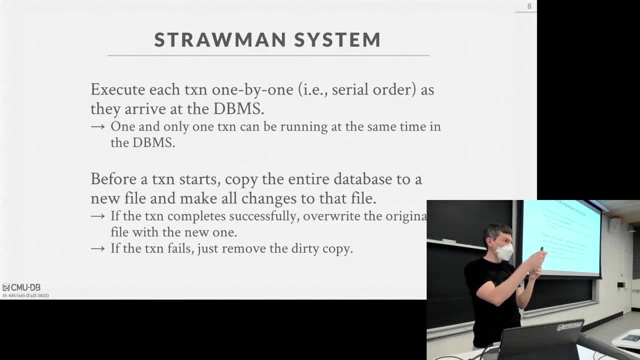 at the same time. they're going to put into a single queue and be one thread, popping those transactions off the queue, executing them one after another, Right, And the only one transaction will be running at a time. So now, when we pop up a new transaction off this queue, 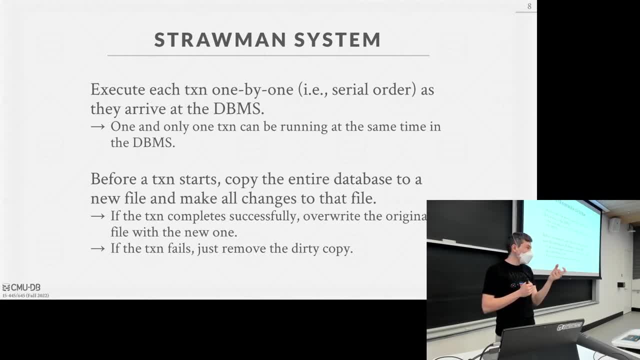 and we start executing it. the first thing the database system is going to do is copy the database file to a new file. Right, Just do the copy command. Nothing special there. And then, when the transaction starts running and makes changes to the database, 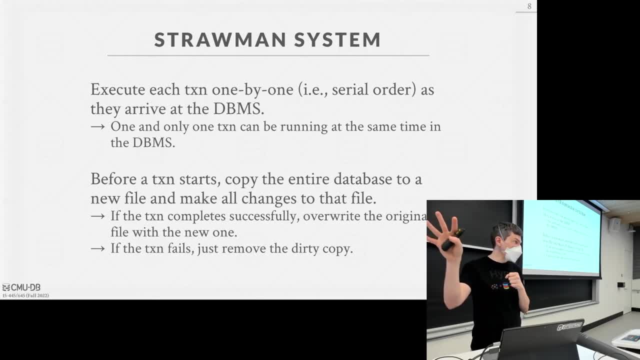 we're going to write all those changes to this new file. Then if we are able to commit, the transaction says I want to go ahead and commit and there's no other mistakes or failures. then we'll just flip a pointer somewhere that says: 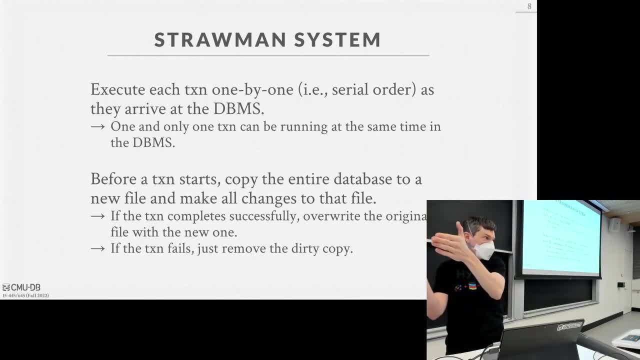 if you want the latest version of the database, it's this new file that we wrote to Right. Would this work? Would this work? Would this solve? Well, he's shaking his head. yes, Right, Would this avoid the partial transaction problems? 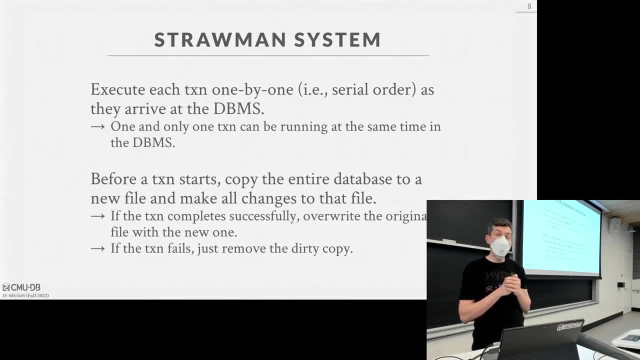 His statement is: can we assume the override is atomic Override of what The pointer Right? so again, maybe I should draw a diagram. There's one file that says here's the file name of the latest version, And then, when my transaction starts, 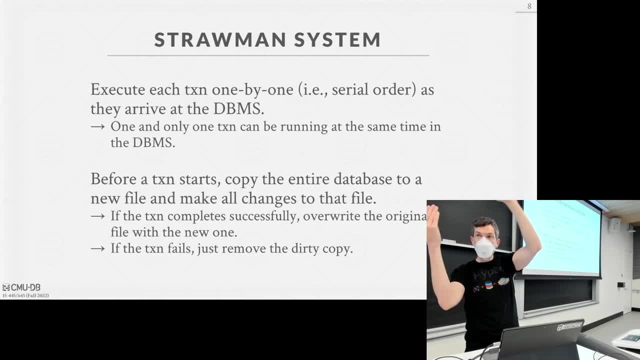 I copy the database like heap file and make a new one on disk, make all my changes and then I make the changes there, Flush those out to disk. Then when I go to commit the transaction then I update that one pointer file and say here's the new file location. 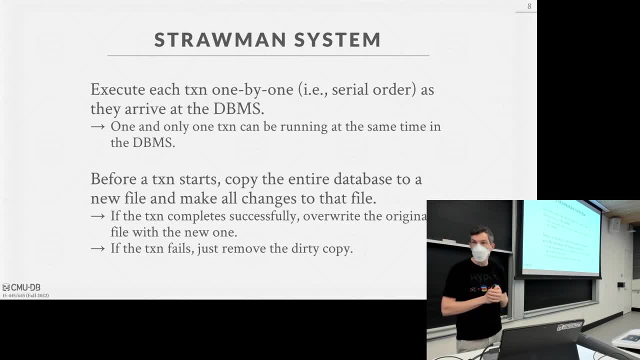 So you can assume that updating that pointer file is atomic. He says he thinks it works. Is this a good idea or a bad idea? Yes, You said you know it's a bad idea. Why? A? it's the same building. 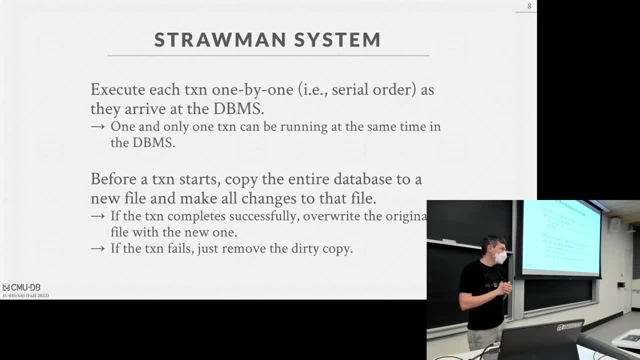 Because if it means zero concurrency and it means that for one connection to occur, all the ones that, And if any of them had anything go wrong, they have to have this very extensive process of not only copying everything but do lots of stuff. 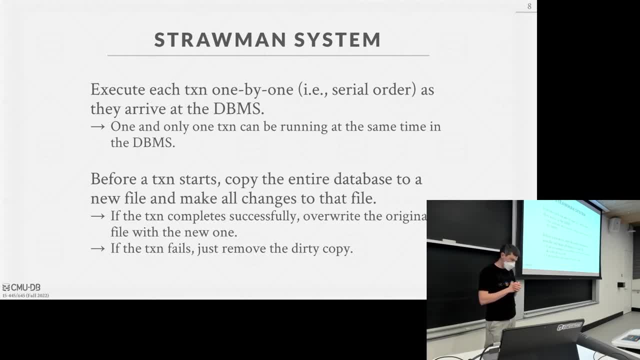 You have to either do a lot of updates at the end or once at the end all the updates kind of get mangled in. But Why would they get mangled in? Well, you have all these dirty copies. What if, halfway through the process of updating, 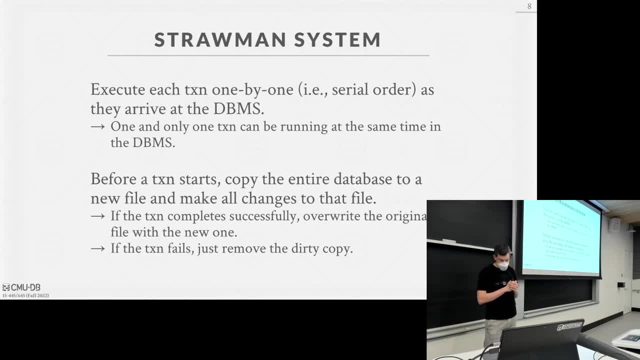 replacing the clean ones with the dirty ones when it's halfway in. that's not going to be your update. That's not really a good idea. There's a lot of other things that you can do. So you're saying that. you're saying: 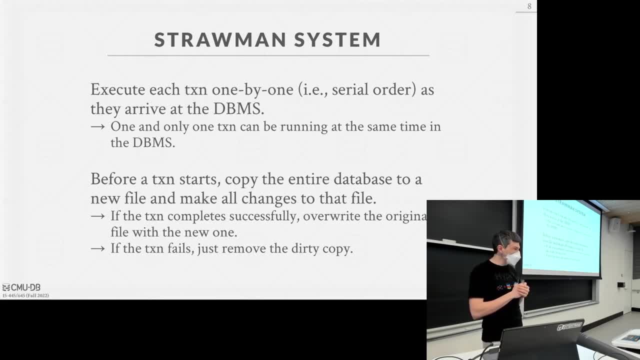 that you're going to have to do a lot of updates because the updates are going to be up to date. Yeah, So you're saying that you're going to have to do a lot of updates while you have all these dirty copies? What if, halfway through the process of updating, replacing the clean ones with the dirty ones when it's halfway in. that's not going to be your update. That's not really a good idea. You can just delete the file. Who cares? That's easy. Yes, In principle, OS can do something like shadow copying. 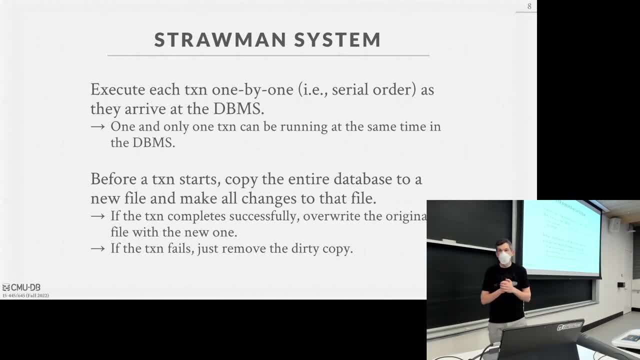 Like, even though you say you want to modify this 50 gigabyte file, maybe only one kilobyte like it will do the exact same thing and then it wouldn't like impact you. You're describing MMAP. 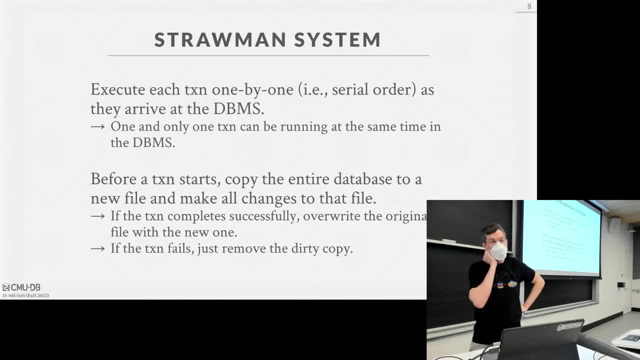 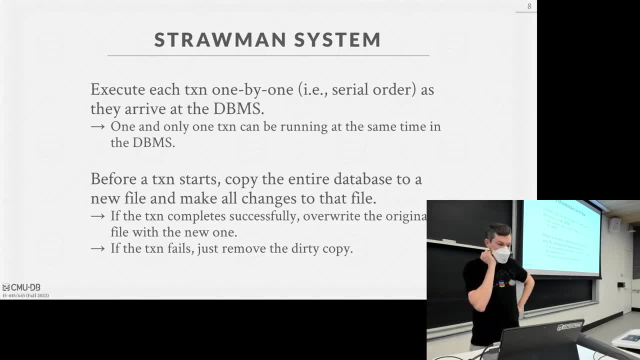 I mean there's no concurrency because you do everything sequentially, Yes, And then every time you actually make a transaction it will copy the entire database file. So he basically said there's no concurrency because the transactions are executing in serial order, one after another. 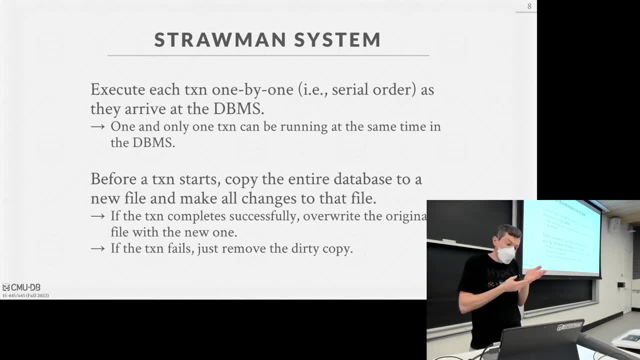 and then every time you want to start a new transaction, you've got to copy this entire file. If it's a four-kilobyte page, The database is only four kilobytes. who cares If it's four petabytes? 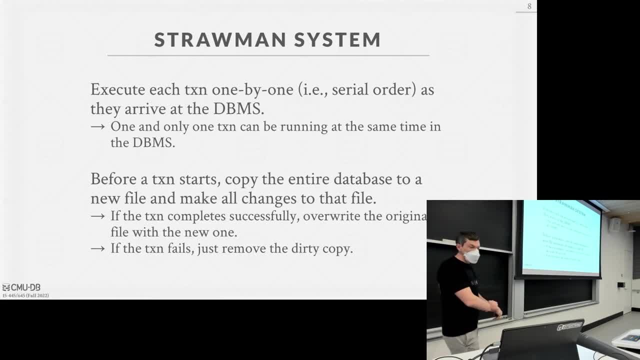 then yeah, you care, So, So this. so there's sort of two ways to think about this. Is it correct and is it fast? This is correct. If you do this, you can guarantee that your transactions will execute in a correct order. 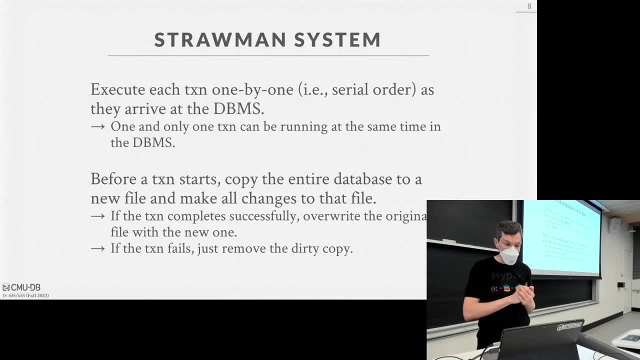 and produce a correct database state And I'll define what correctness is in a second. But as you guys pointed out, it's going to be slow Now if you think about the problem you have with checkpoint two, you had to rate a concurrent B plus tree right. If you make it single threaded you don't have to do any of that right, And there are some systems like Redis and BoltDB that actually do that. But in general we're going to. most systems are going to have concurrent threads. 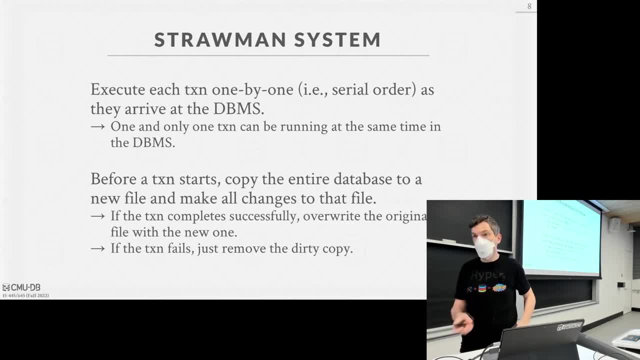 and concurrent transactions. so you do need that concurrency control. Yes, But isn't Redis mode to be quite fast? So what's the? I don't quite get it. Your statement is: is Redis mode to be quite fast? Why Is that what you're asking? 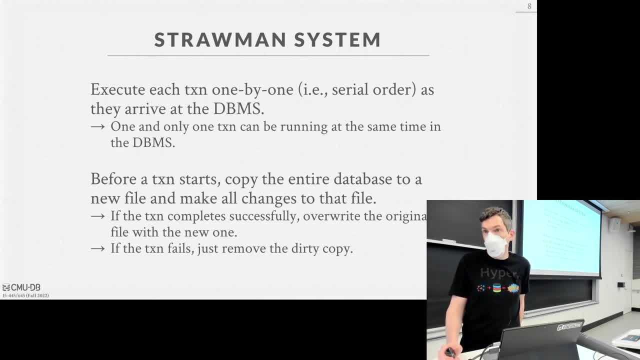 Because it's single threaded and in memory, right, So like if your database fits entirely in memory, fantastic, great. If you can execute all of the operations you need to do with a single thread, then yeah, great, Yes, So why can't we execute the entire database file? 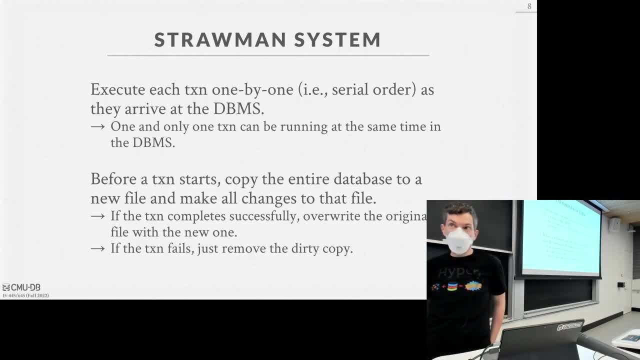 Yeah. so his statement is- and we're getting this- like: why can't we just do this instead of copying the entire database file? what if we copy pages? That's shadow paging. We'll get to that in a second, yeah. 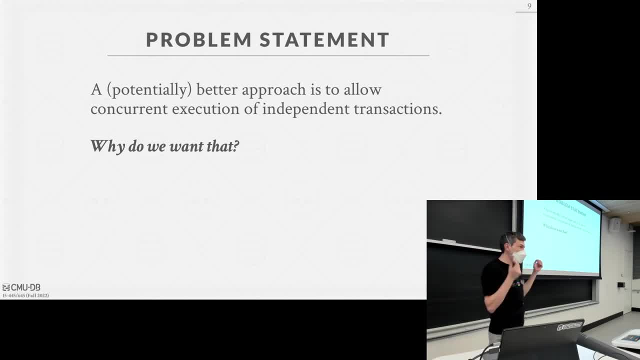 Okay, so this will work, but it's going to be slow And in a modern system, we're actually going to want to have concurrent transactions, right, Because, just like we had when we talked about parallel execution, we want to take better transactions. 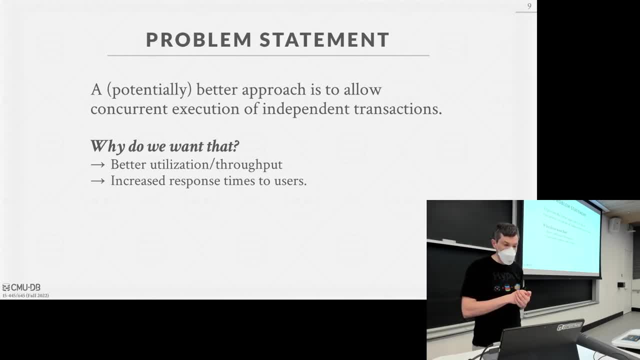 We want to take better advantage of the hardware that we have, allow multiple threads run at the same time And, in any case, that we have a transaction that tries to read something that's not in memory. right, there's a miss in our buffer pool. 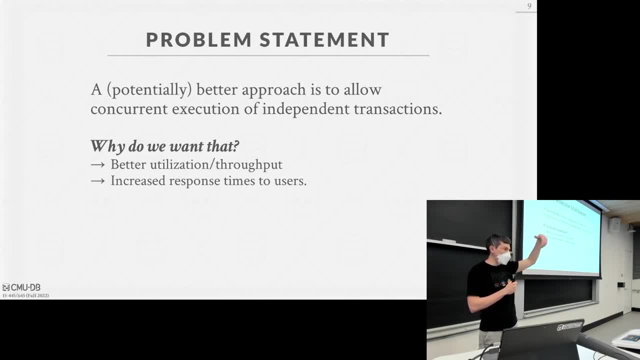 and we've got to go out to disk and get it. well, we can let that transaction wait, install while the system fetches that disk or fetches the pages from disk, but then we can let other transactions keep running right. 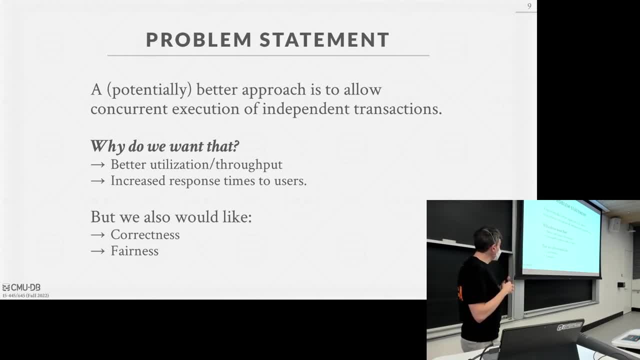 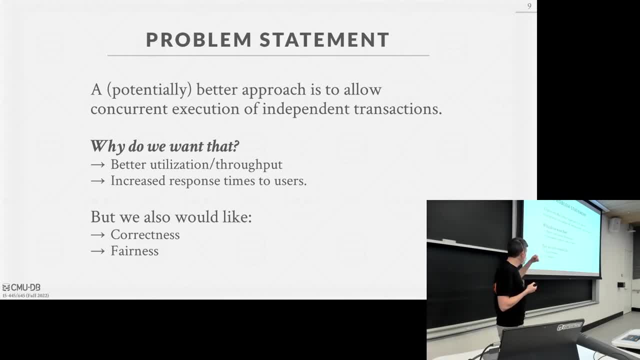 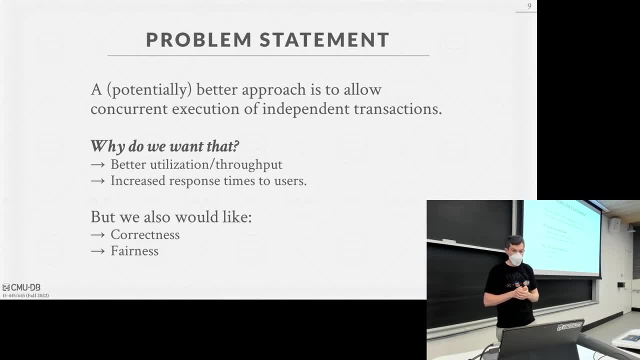 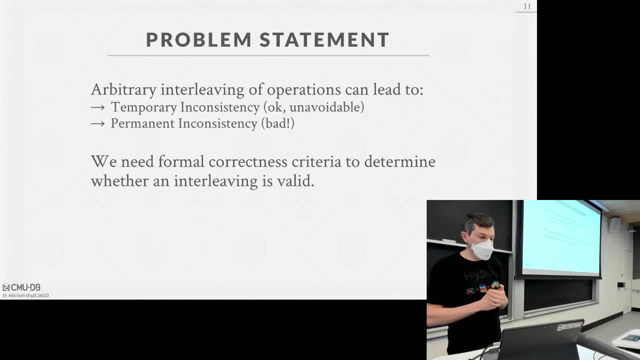 about fairness, right? We don't want transactions to get starved, you know, because they keep getting preempted by some other transaction. So the challenge we're going to face is that when we start interleaving these operations in our transactions, it's going to put the database in an inconsistent or invalid state. 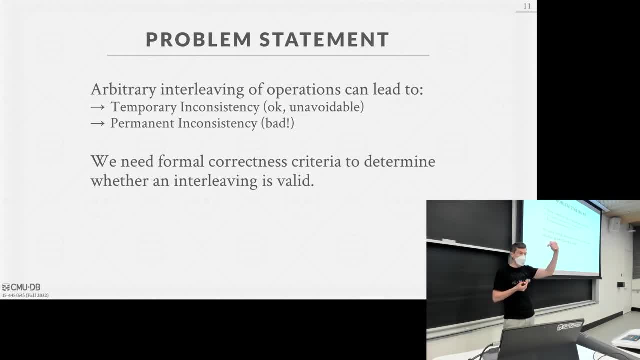 Okay, right. so my example of taking money out of my account, putting to my bookies account: right, there'll be a moment where i'll take the money out of my account and at that point in time that money doesn't exist anywhere because i haven't put it in. you know, updated the other. 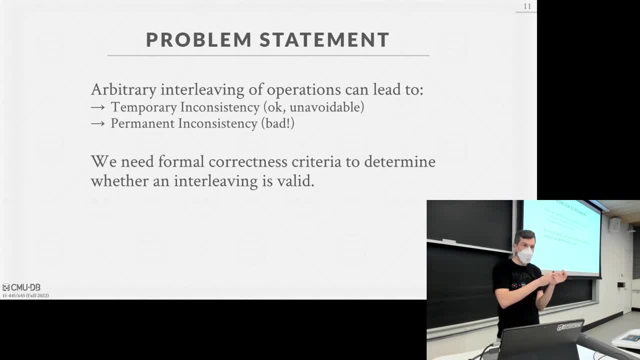 the other account with the new, new value. right, so that's unavoidable. right, think of the low level execution of the system. right, there's no magic, you know. instruction that we can go update two different pages atomically at exactly the same time. right, so these temporary inconsistencies? 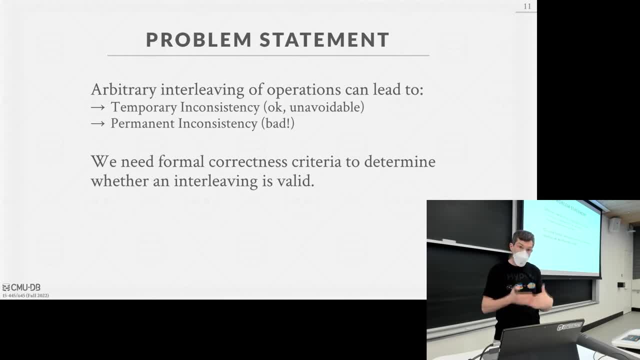 are going to be unavoidable, but it's okay, because we're not going to expose that inconsistent state to the outside world again. i'll explain what all this is it means in a second. what we want to avoid is the permanent inconsistency, meaning like if i take the money in my account, the system crashes. 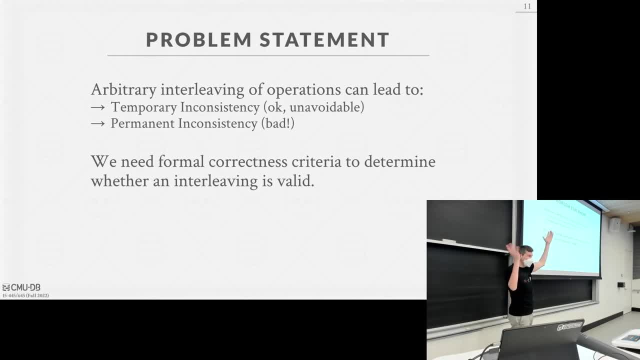 and i don't put the money back in my account. now the you know, the bank has magically lost a hundred dollars and that would be the end of the system, right? so that's a good example of that. so these these the protection mechanism we need to have to make sure everything is going okay. 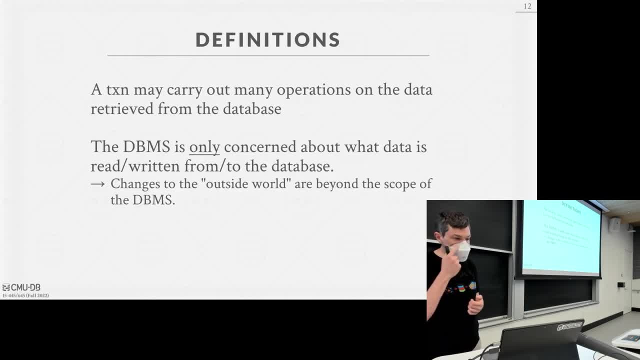 so to define what it means to be, uh, correct, we need to define actually what a database is, and this will be a simplifying instruction, or simplification of how a real database works, that we'll go through for this class, because i'm making it easier to understand these concepts as 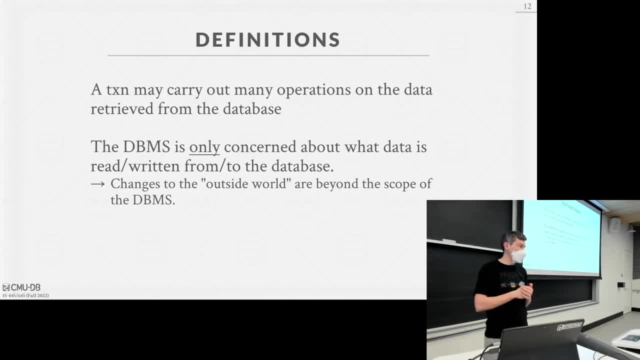 we go along and then on tuesday next week, when we talk about two-phase locking, we'll talk about how to do this in the context of a real system. so the, the transaction, is going to be able to carry out as many operations at once on the data. 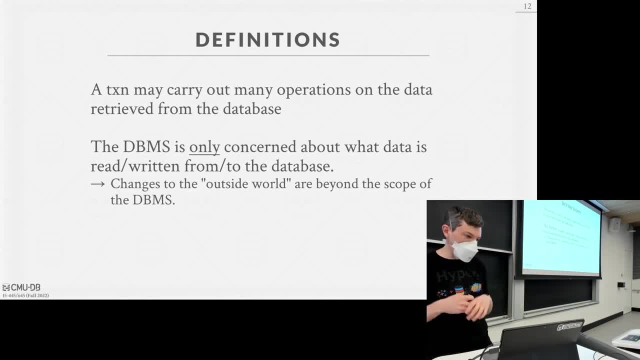 or the database, uh, and it can read and write whatever, whatever it wants. i'm not going to define what actually is a, an object in the database, uh, we'll just call it. you know, use, use variables, abcd. uh. in practice it's usually going to be a tuple, but you could apply these. 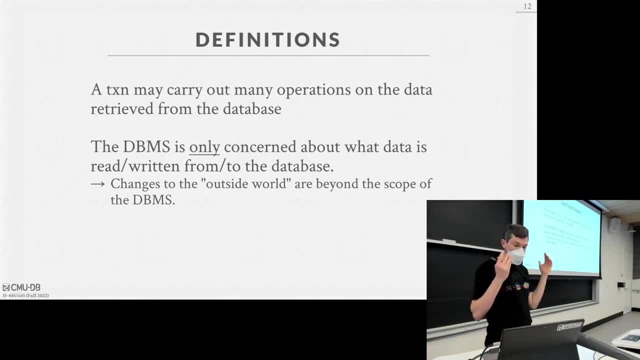 same techniques for for for pages, for tables, for for for databases. and the other thing, important thing to understand is that we can only use the same techniques for for for pages, for tables, for for pages, for for for for pages or for page, for pages only. uh, the tables has only been able to. 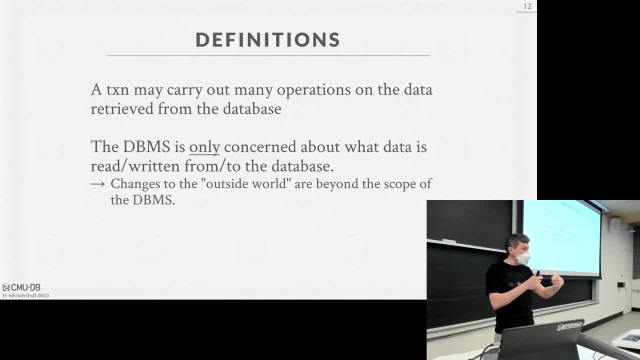 control things that are within its purview, uh, or meaning of the data that is actually being stored inside the database. so that means if the application does something that leaves the orbit of the database system, we have no control over that and therefore we can't- we can't reverse that. 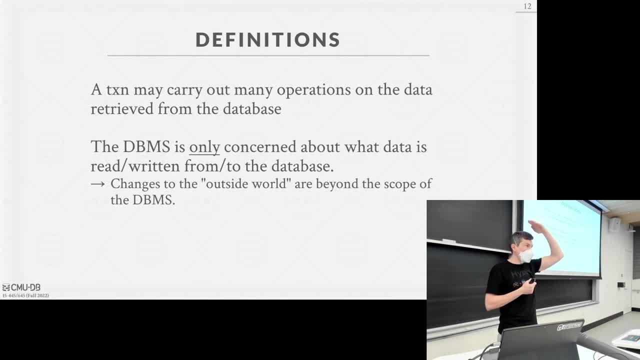 and roll things back, meaning like if i, uh, if i take the money out of my account, put it in my bookies account, and then the application sends an email confirmation to say: hey, andy, you know we did. but then the transaction aborts and rolls back that change. 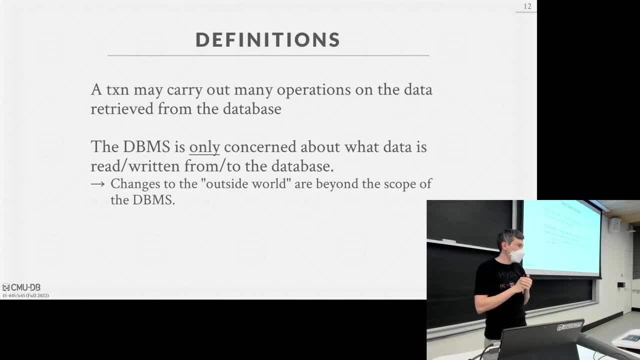 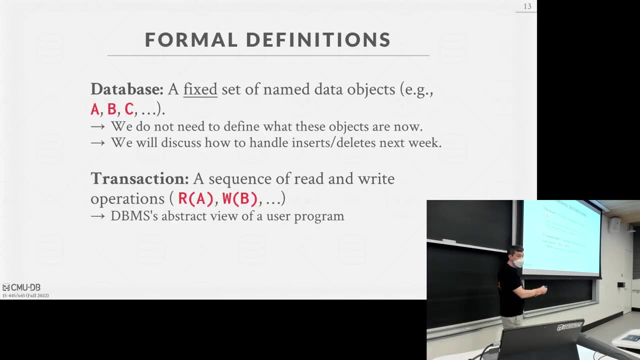 the database system can't magically retract that email. so there are external things that the application may do in the context of a transaction, but because the database system is not the one doing it, it has no control. alright, so we're going to find a database for this class to be a fixed. 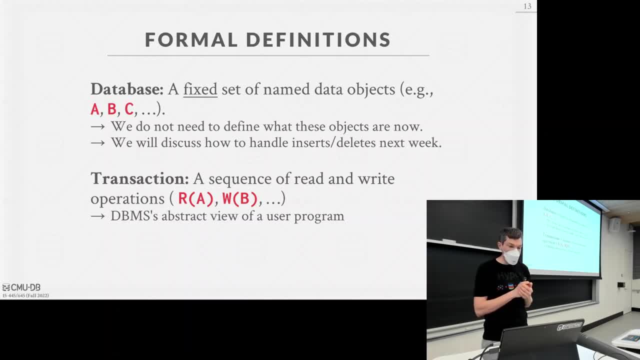 set of named objects. as I said just ABCD. we don't need to define what those objects are now. all the techniques we'll talk about today and actually pretty much all the techniques we'll talk about going forward, it doesn't matter what the granularity is. and the other key thing to point out is that 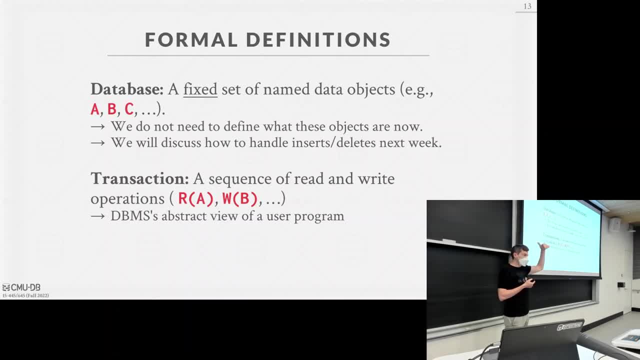 I'm saying the database is fixed, meaning we're not going to support inserts and deletes. we can only do reads and writes on database objects that already exist. again we'll see how we handle that inserts and deletes, next class and then for our transaction we're just going to say it's a sequence. 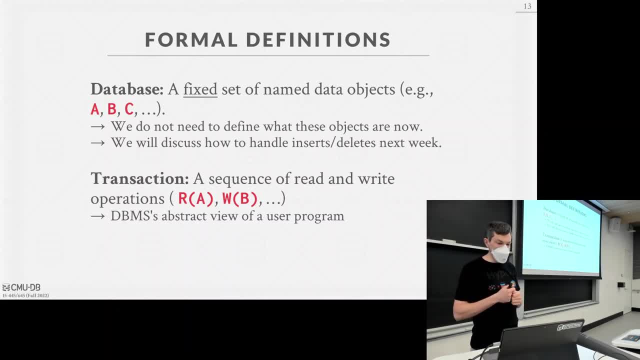 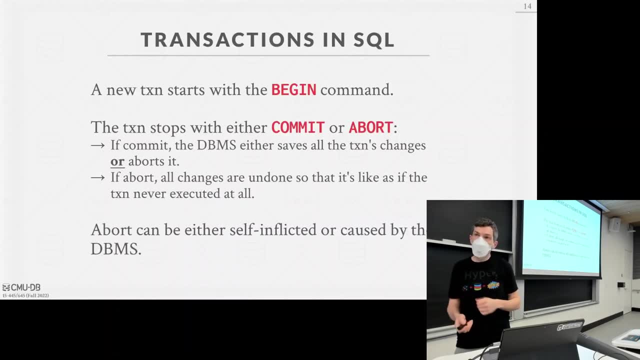 of read and write operations: read A, write B and so forth. we don't see. for our purposes here we're not going to actually see SQL queries, sorry. so in this case, write is like an update, right? yes, in this statement, write is an update. yes, write is a web page rather than. 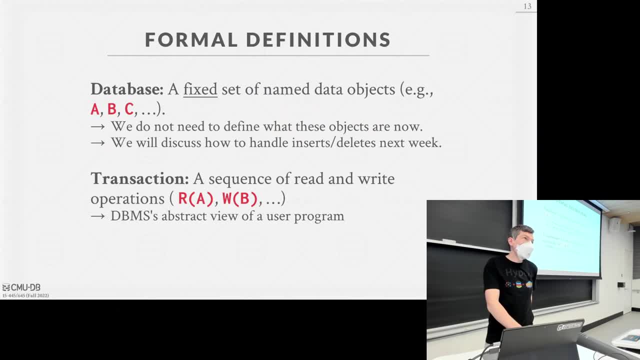 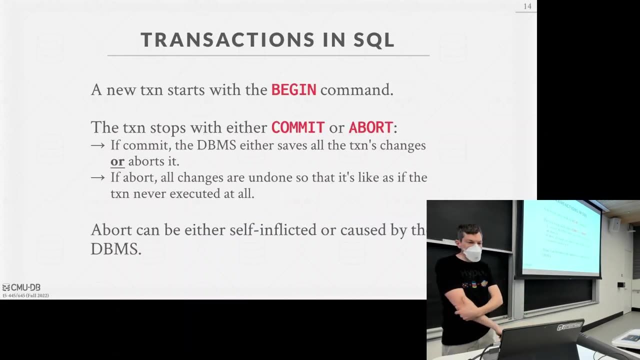 a pen again. yeah, like think of it's overwriting whatever the value was there before. right say B equals Andy. I overwrite it with B equals Charlie, right. so in SQL again, we'll talk too much about this, but you'll see it in the schedules that I show. 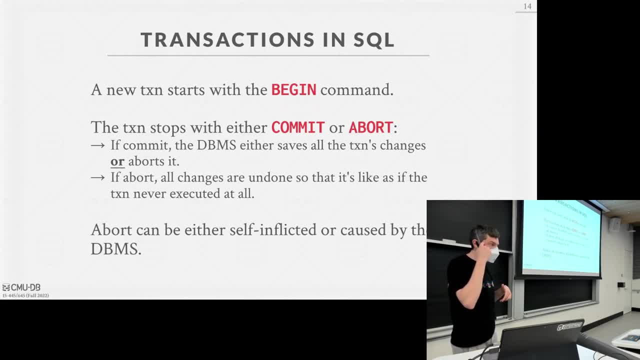 you start a new transaction every time you call begin. there is something called auto commit where basically anytime I have a SQL query it assumes that's the start and stop of a new transaction. but in general you explicitly start the transaction in SQL using begin and then you can either. 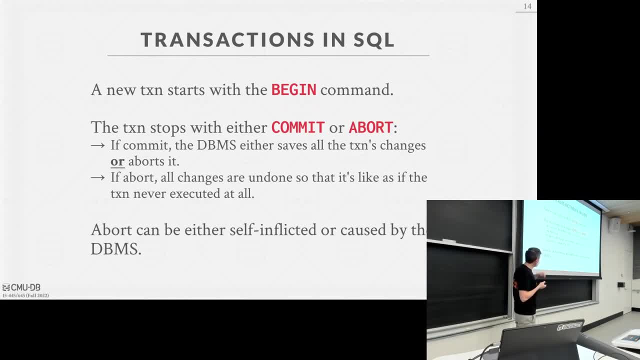 complete the transaction with either a commit or an abort. commit says: I want to save all the changes I made. abort says: rollback everything. I think the SQL standard also supports the rollback. instead of abort, you can say rollback. I think Postgres supports both abort and rollback. MySQL only supports one. 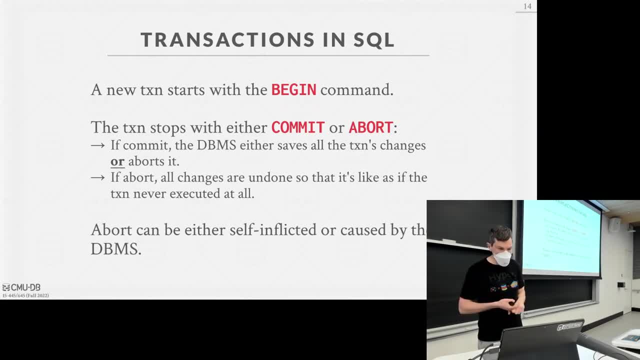 I can't keep track, but like I'll just use abort because there's fewer characters, fewer letters, right? so if I abort, then it's going to be as if the database never executed the transaction at all. now, one important thing to understand also, too, is that if the applicant says 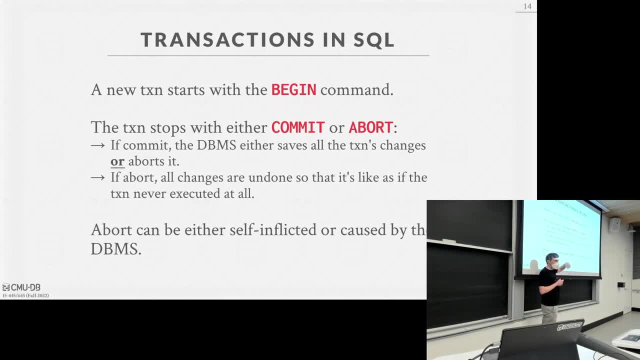 call is commit, there's no guarantee the database system is actually going to commit your transaction. so if I abort just because you want to commit doesn't mean it's going to let you. so it may be the case that you call commit, the database says uh-huh, no, you did something. 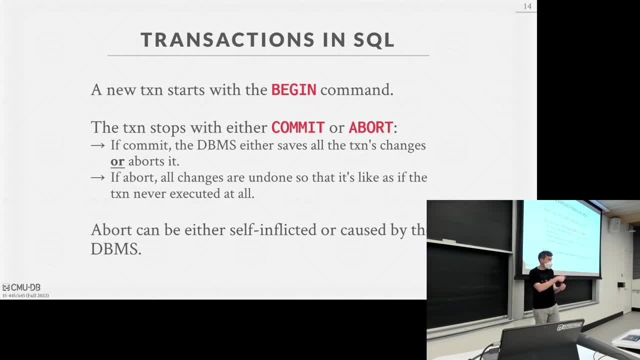 you're not allowed to do and you actually get an abort and you get an exception thrown back at you. it says we can't commit this transaction and it gives you usually might tell you why and there are partial rollbacks which we can talk about later, but in general you have to write your application. 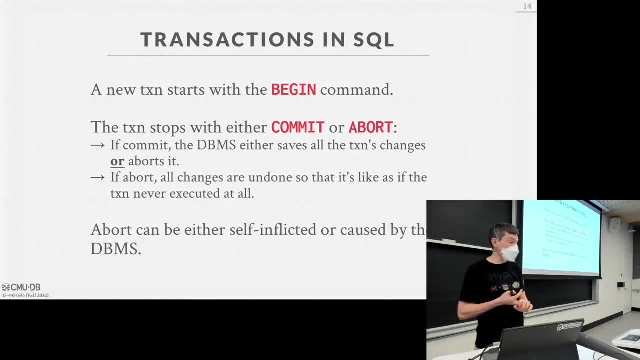 to when you call commit, handle the exception that says I wasn't allowed to right and the aborts could either be because you call abort or, like I said, the database system. you can't proceed and it kills you. yes, the question is, why would the database system? 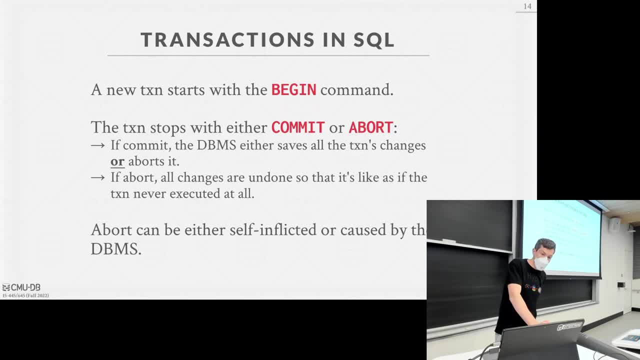 fail on the commit step and not on the early queries, because you could do what's called optimistic currency control, where you assume everything's okay, you let it do whatever the transaction do whatever it wants, and then only on commit you go then verify all right, so we 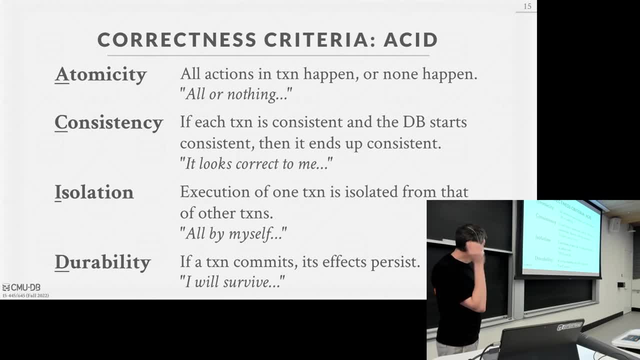 sound like everyone heard of asset before, so I'll go through this quickly and then we'll go through more details how this is actually implemented. right? so asset stands for atomicity, consistency, isolation and durability. so the first one, atomicity. basically it's the partial transaction thing. 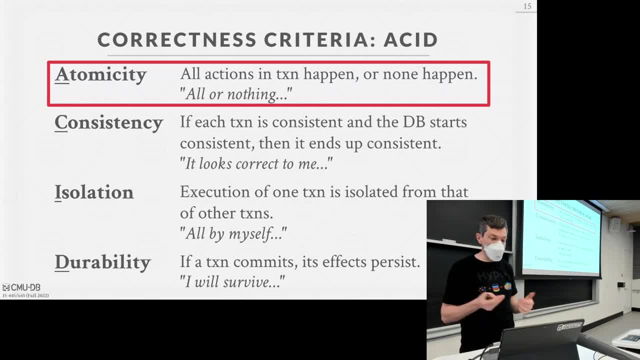 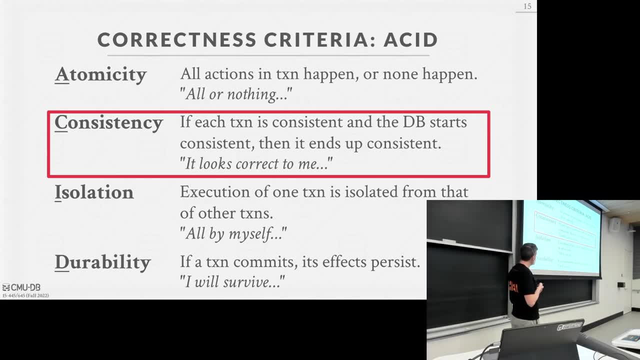 right: all the actions or operations or transactions have to occur or none of them happen. right- consistency: this one's a bit vague and we'll see why when we discuss it. it'll make more sense when we talk about distributed databases. but it basically says if the transaction is consistent. 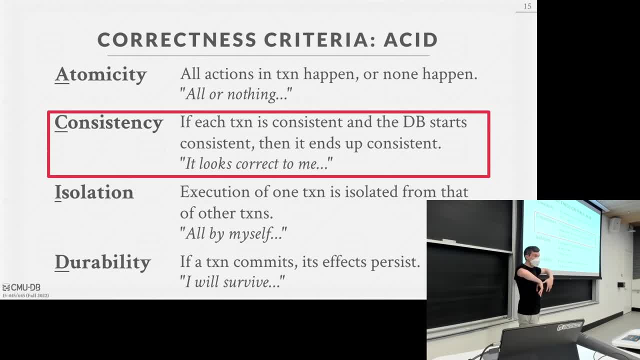 and the database starts off being consistent, then when we talk about the transaction, if you want to execute this transaction, it has to be consistent, right? that's pretty, that's pretty confusing. it basically means that, like if the database was correct and the transaction does correct things, then 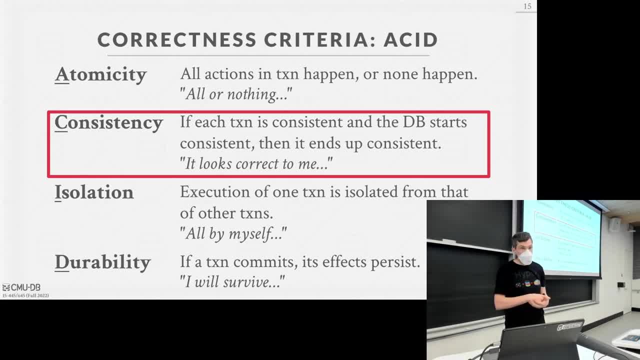 my database will be correct after I execute the transaction. now you're saying: what does it mean to be correct? it depends. so the true story is, like the supposedly the guy that invented this term, acid, he kind of admitted he shoehorned C in there to get. 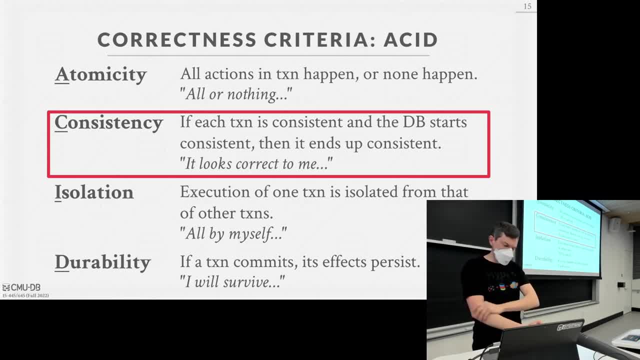 to make it be acid because he was trying to make it in front of his wife or something. it's some- I don't know if it's an urban myth or whatever, but like his wife didn't like sweets, so he called her an acid woman. so he named this after her. 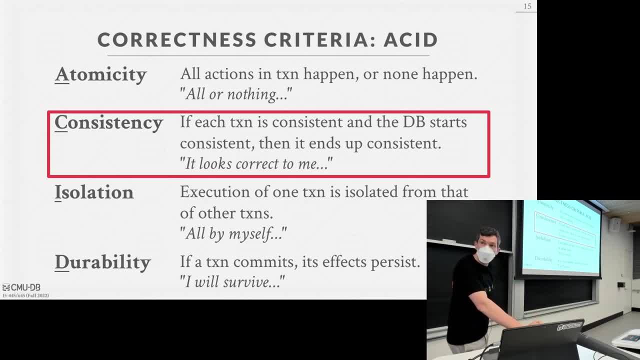 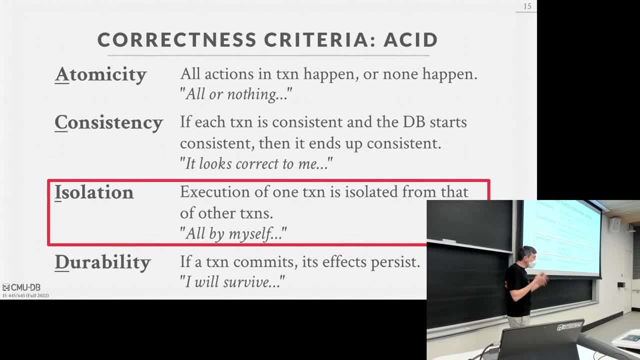 he was German. is that? huh, he's German, so who knows? all right isolation could be the we want to give the illusion that our transactions are executing in serial order, like one after another, even though they're not really. and then durability means that if the transaction commits, 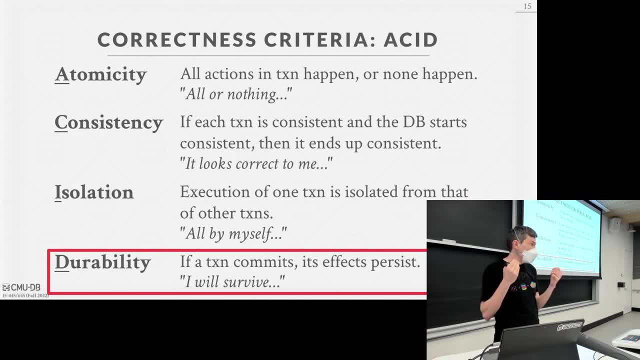 and we get the notification by the outside world that it commits, then the message is that no matter if the database system catches on fire or blows up or crashes, then we should be able to see our changes afterwards, that someone might come and overwrite those changes. we obviously have to support that. 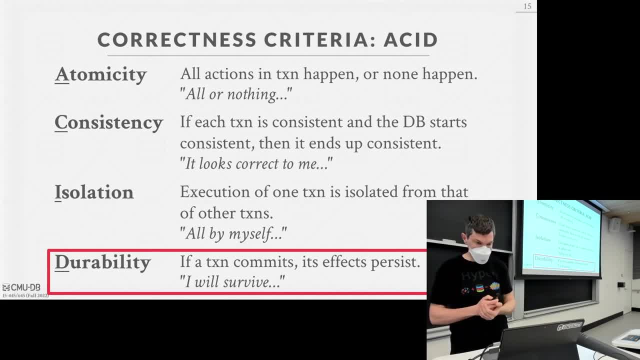 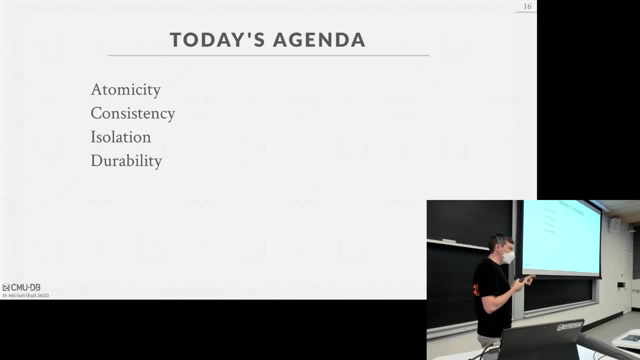 but assuming that's not the case, then our changes should be durable. all right, so we're gonna go through these one by one again. so today's class is the high level concepts and understanding what this all means and how we'd actually potentially implement it, and then 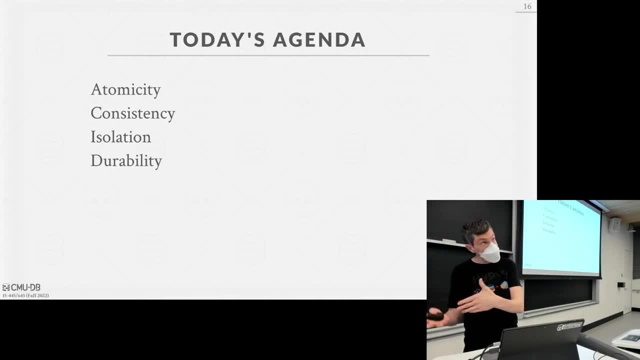 and we're not gonna go into actually specific algorithms and actually implement this. we will cover that starting next week. I just wanna make sure you guys understand what's actually going on, why these things matter and what are the sort of correctness guarantees we need to provide. we're mostly focused on isolation. 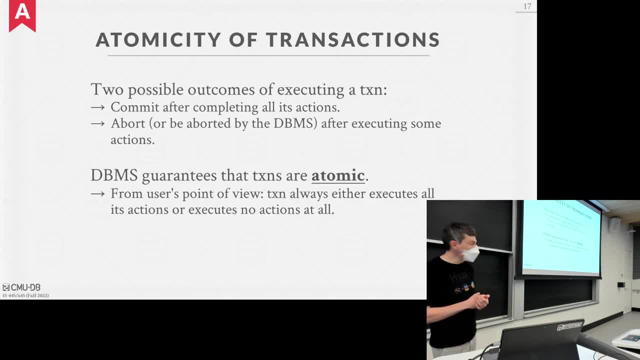 because that's the trickiest one here. all right. so, as we've already said, atomicity- okay, it's no partial transactions. you're basically guaranteeing that all the operations that are in a transaction will happen atomically all at once. right and again, it doesn't mean that it's gonna. 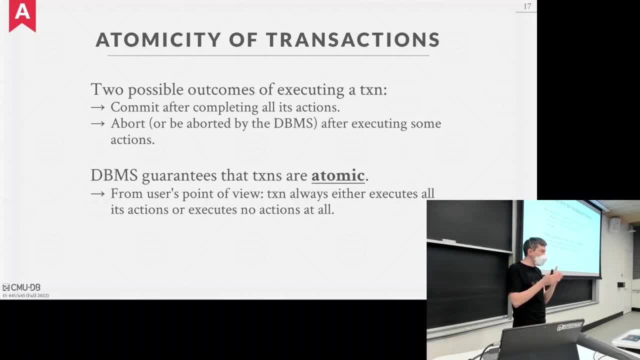 you can't execute these truly atomically in some point in time, but from the outside world it'll appear that's the case, right, so that if we go and commit, then all our changes get applied. if we abort, then everything gets rolled back. so these are the two examples. 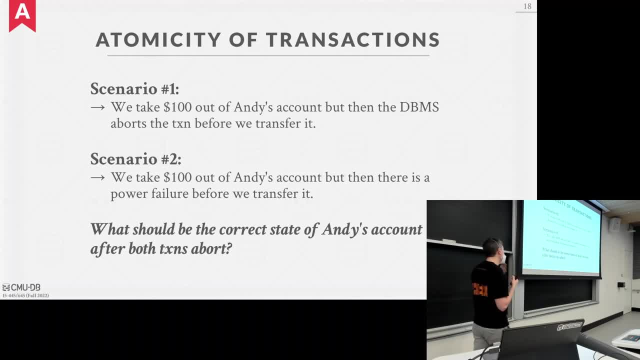 that we talked about before, well, the taking the money out of account, putting my bookies account. but it's two different scenarios of this. so if we take $100 out of my account but then the data system aborts our transaction before we apply it to the other account, 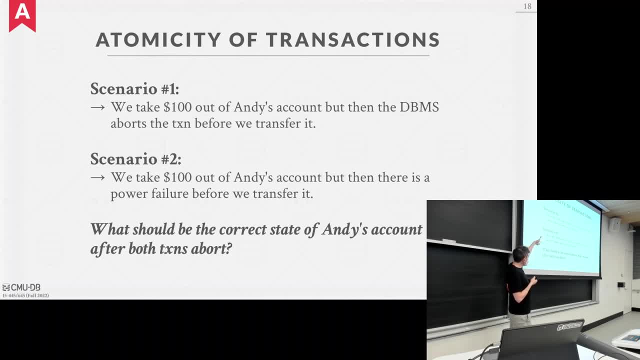 we need to make sure we roll that one back, and then if we take the $100 out of my account, but then there's a crash and a failure again, it's basically the same thing. we need to make sure that this doesn't happen. so the correct state of the database. 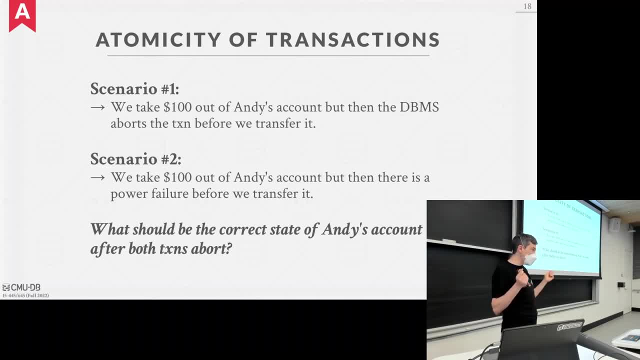 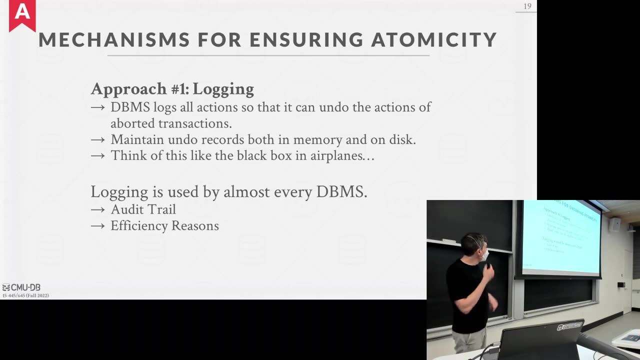 in both these scenarios will be as if my transaction didn't execute at all and the data system is going to use concurrent protocol and it's and the recovery scheme to ensure that this is the case. so there's two basic ways to support this. the first is through logging. 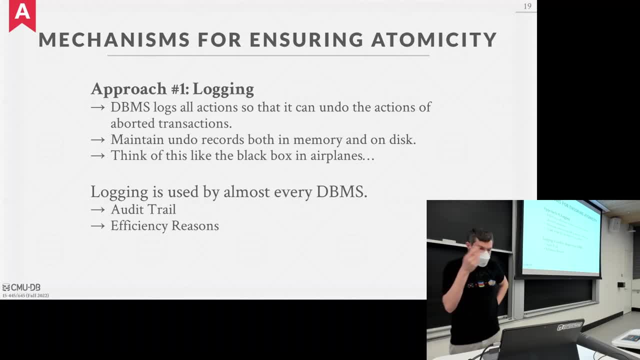 sometimes also called the right-hand log, or that log structure stuff that we talked about before- where, as the transactions are making changes in the database, we're going to write these log records that keep track of the change that was being made, and it'll have information on how to undo that change if necessary. 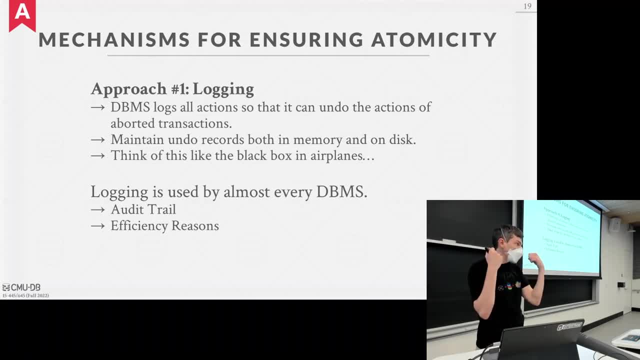 so now, if there's a crash, then I can go back and look at my log and say, okay, what was I doing at the time of a crash, before this thing got committed, and potentially reverse those changes in the case of the log structured storage that we talked about before. 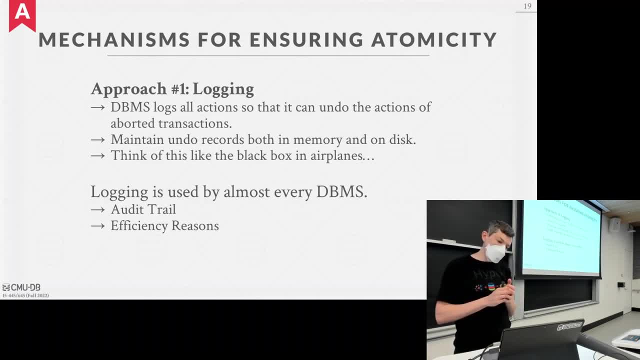 there really isn't that any recovery you potentially have to do, because the log itself tells you exactly what happened. so most systems are traditionally most systems would maintain a log separate from the database heap files. if you're using log structured storage, you don't need to. the log itself is everything you need to provide this. 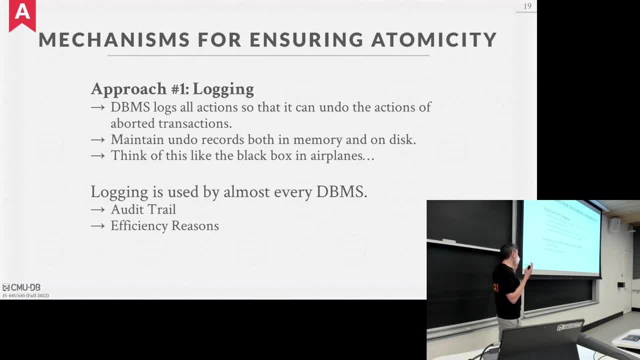 beyond just for durability reasons. logs are used in for a bunch of different reasons. it guarantees that you can have much sequential writes instead of random writes, and it often times too in. like enterprise systems. you need the log for auditing. there's, like you know, regulatory reasons you need to keep track of. I think in the US, 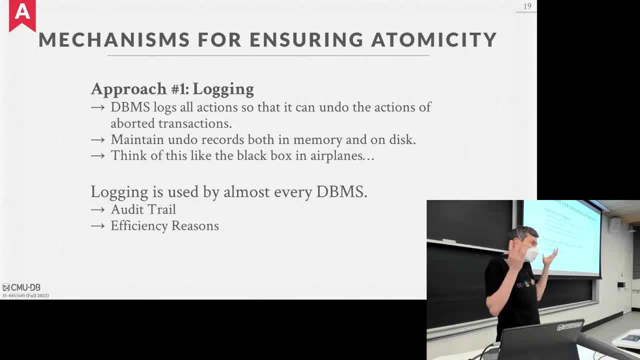 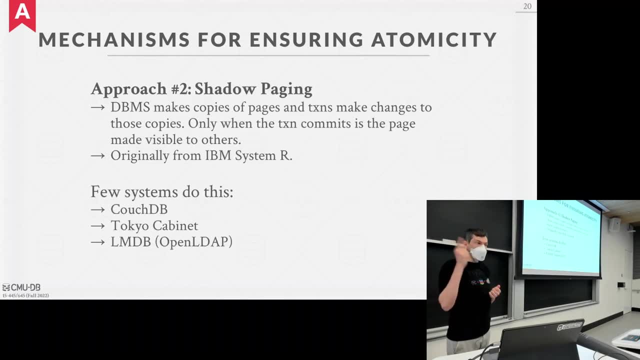 the last seven years of any financial transaction. so that's essentially the right-hand log. you could use that to figure out what actually happened. all right, the other approach is what he brought up and it's called shadow paging, and it's basically the same example that I talked about in the beginning of the straw man. 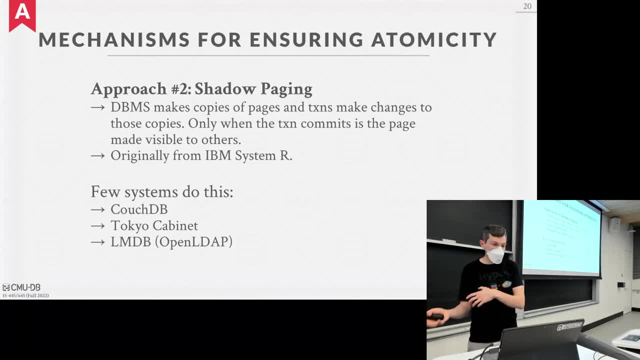 where, instead of actually copying the entire file, you'll copy the pages that the transaction modifies, keep track of some. there's some data structure keeps track of what those dirty pages are and then, when you commit, you just flip a pointer to say, okay, here's the latest version. 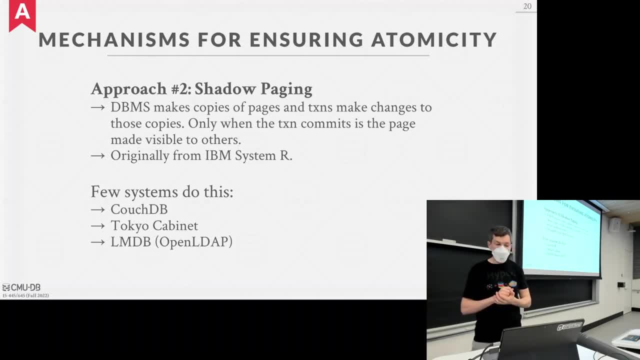 of that directory data structure with all my new updated pages. all right, so that's the other approach. so this technique is rare, the logging one is the most common. but this is actually what they implemented in the first relational database system at IBM right in system R, but they ended up banning it. because it would suffer from a lot of fragmentation. because now you're, if you do like you would sort of invalidate pages because they would get, they would get updated by a transaction. you have to update new pages and then you just sort of had this hodgepodge. 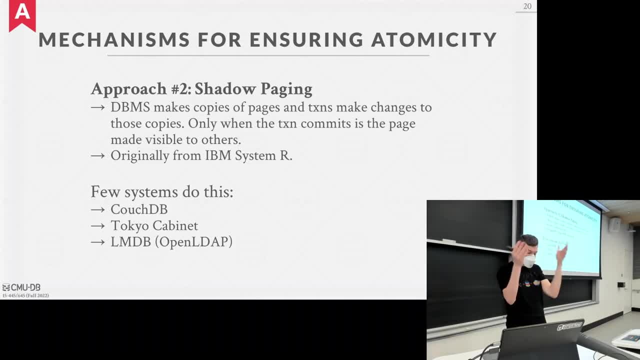 of of pages and what was the latest version of the database at any given time and you had fragmentation, you had to do garbage collection, it was very expensive and it was a lot of random reads, whereas if you use the write-ahead log from the last slide, you get sequential access. 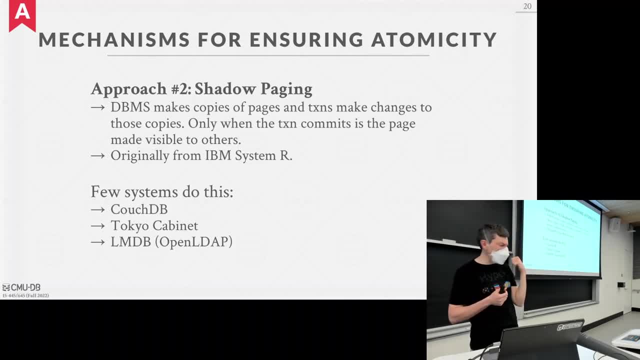 and that's better. so they abandoned this. and then they, when they built DB2 in the 1980s, they switched over to the logging approach. the three systems, the modern systems that actually I know that do do something like this, is CouchDB, Tokyo Cabinet. 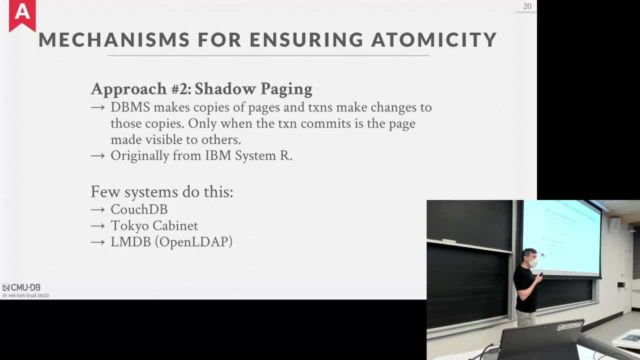 and then they did something like this in LMDB. LMDB is a embedded in-memory B-plus tree or index-organized database that uses MMAP, and this guy is very, very- how do I say this? he is very, very opinionated about how great MMAP is. 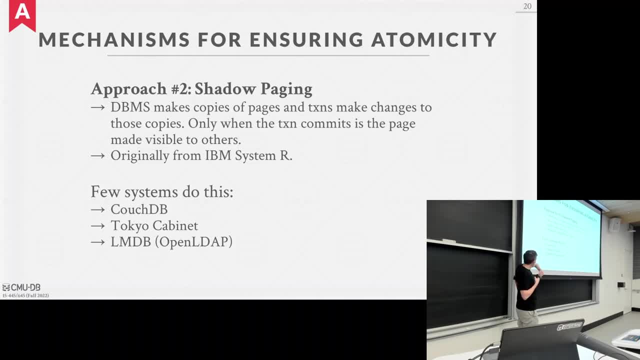 and he emails me about this. he's wrong. okay, CouchDB uses something similar and the Tokyo Cabinet was a embedded key value store that was sort of popular out of Japan a few years ago. I don't think a lot of people are still using it anymore, but again, this is rare. 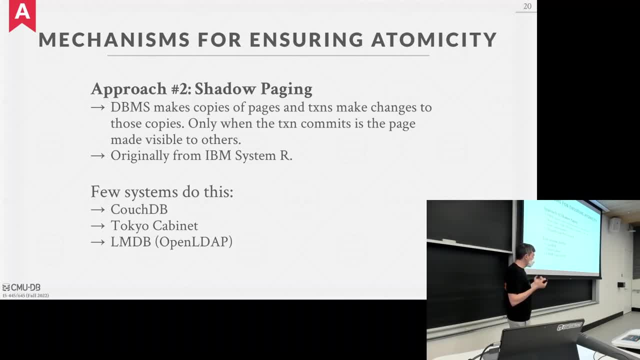 so the advantage of this approach- why would you want to do this? is that you actually get instantaneous recovery in the write-ahead log approach. when you crash, it's like the black box of an airplane. if the plane crashes, you've got to look in the black box. 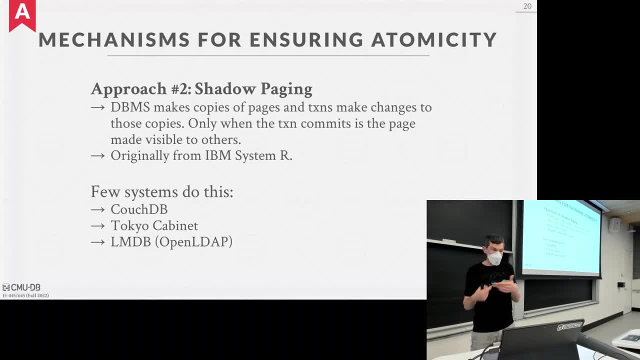 and figure out what actually happened. same thing with the database. when it crashes, you've got to look- the system has to look- in the write-ahead log to figure out what was going on at the time of the crash and put the database back to a correct state. 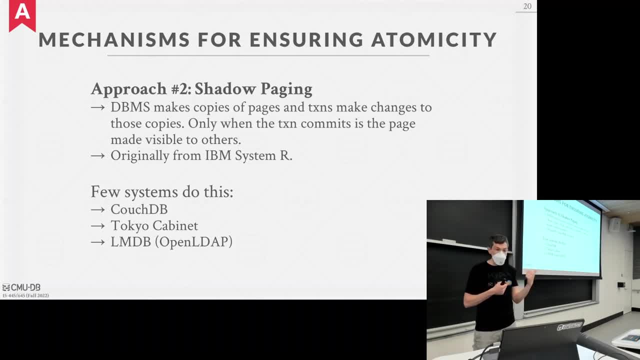 to remove any partial transactions in shadow paging. when you crash and come back, you don't do anything because that pointer is always going to point. the directory is always going to point to the latest version of the database- any transaction that was running at the time of the crash. 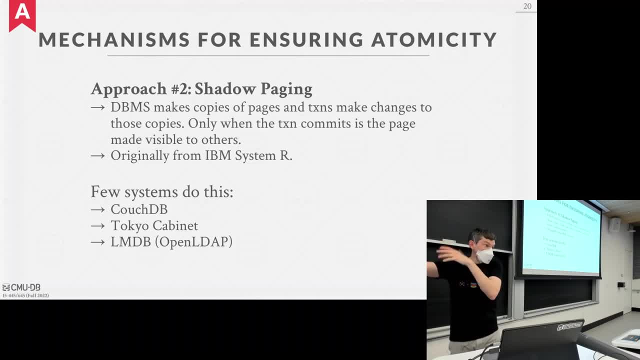 they were updating a bunch of you know like secondary copy, the shadow copy, so you just ignore that and garbage collect that when you come back up, right. so you know. it's not to say that this is a terrible idea. it does have particular advantages, but most systems should be. 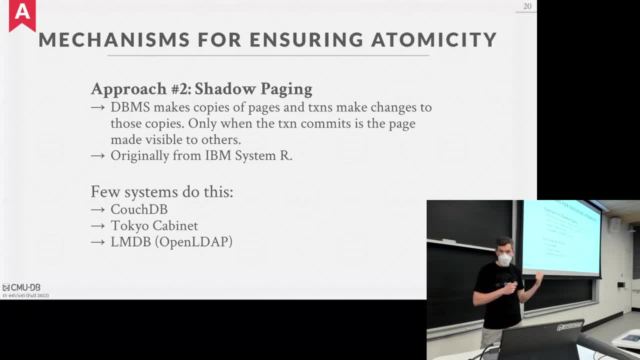 you just choose the write-ahead log approach. the logging approach because of performance reasons. yes, what happens if the crash is during the updating of the pointers? question is: what happens if there's a crash? is updating of the pointers? you assume that has to be atomic. 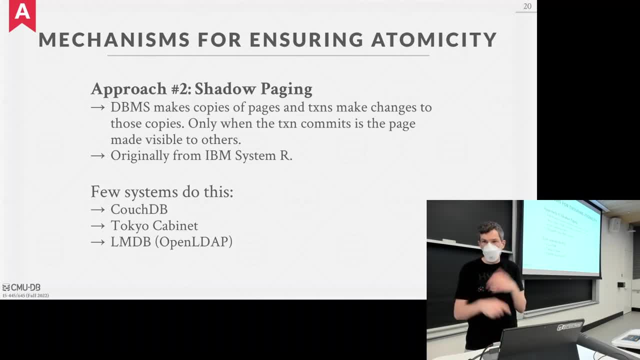 like that has to be atomic, but it's updating a pointer like you can do that atomically. the one system that is interesting that did do this as well- I don't know the name of it. it was the 1970s. it was this database built by 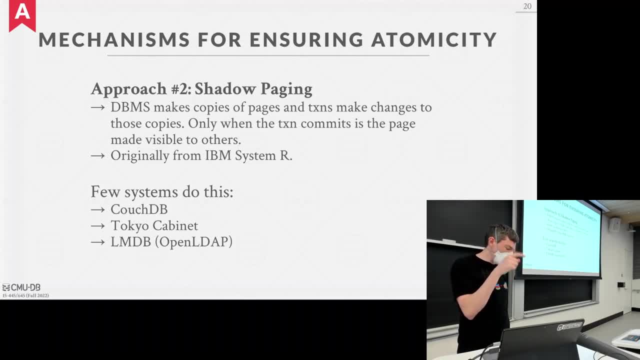 like the Puerto Rican telephone company, and Puerto Rico has problems now. but in the 1970s they had even more problems with the power. the power was always going off randomly. so they built a database system using shadow paging, because when the power went off randomly the system would crash. 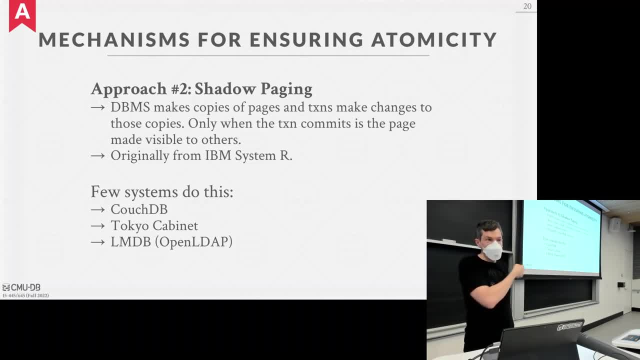 and because it happened so many times during the day, when the power came back on. you would have instantaneous recovery if you use shadow paging. yes, does this allow for concurrent access to certain pages? this question is: does this allow for concurrent access to certain pages you would have to use? 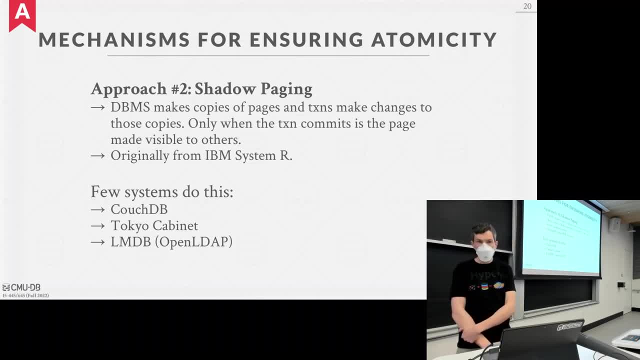 like the isolation mechanisms above that? yes, but you could. back in the day, though, it was like it was a unit processor, it had one core. yeah, yes, your question is, and she's correct. if you're using shadow paging, you don't make a copy of the entire database. 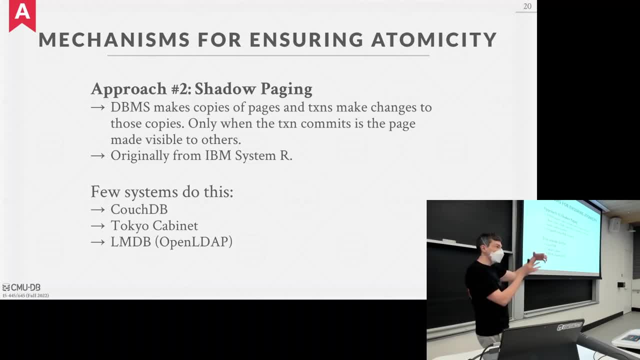 as I said before, you make a copy of individual pages? yes, but there's additional data structure to say here's the pages I've copied. yes, this question makes more sense for memory databases. I think right-hand logging is still better. the logging is still better. we can cover that later. 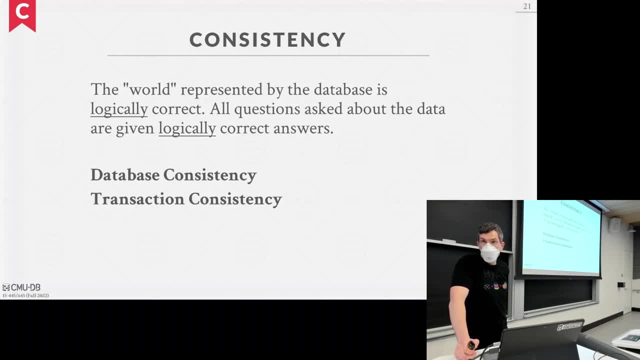 yes, but how many did you think? because I thought it was a small. let's take that offline. you should have a log. you logged a disk, yeah, okay, all right. so let's talk about consistency again. this one is kind of kind of vague, and it's so bear with me here. 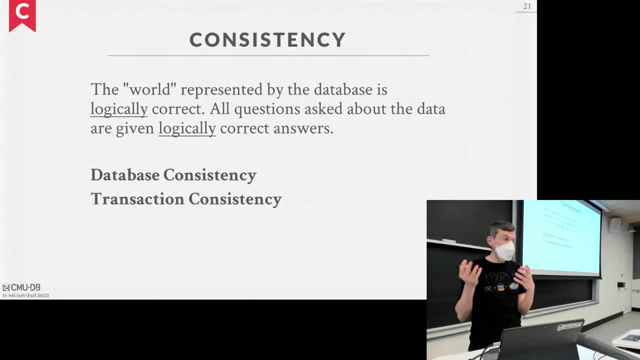 so the thing I understand is what the database is trying to do. the database is trying to model something in the real world, right, and so you think of: like I have a database on S3, what students take what classes, right, you're all here as students, you're enrolled in this class. 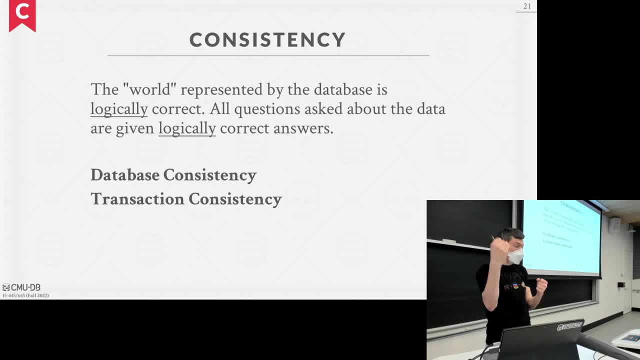 so somewhere there's there's a record that says student X is enrolled in 15.4.45.6.45, right, and then if you're enrolled in the class, you obviously want a row there. if you drop the class, then that gets marked as dropped. 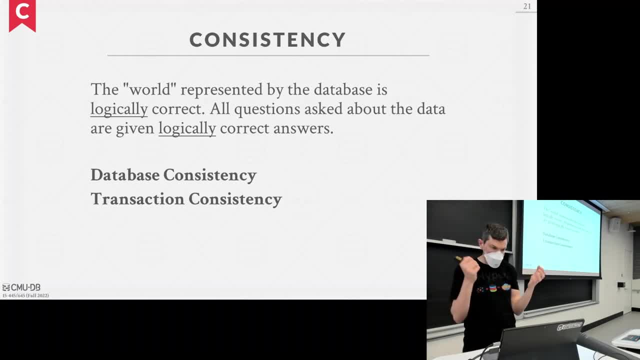 and so forth. right, and so you want whatever the thing in the real world to be like, logically correct, so that when you ask questions about it, like is this student enrolled in this class, and the person is truly enrolled in the class, it comes back with yes, true, 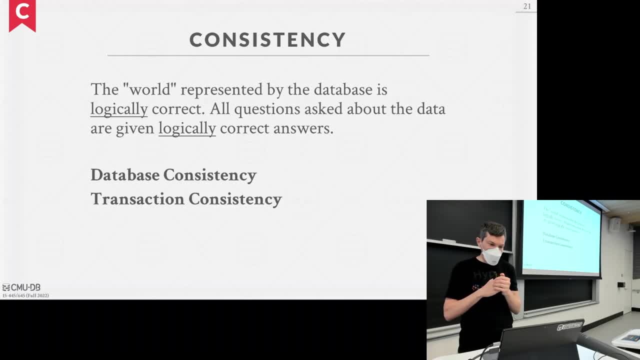 right. so that's what I sort of mean by consistency, and there's sort of two levels of this. one of them is something that we can guarantee and one of them is something that it's really left up to the application programmer because it's just too this. 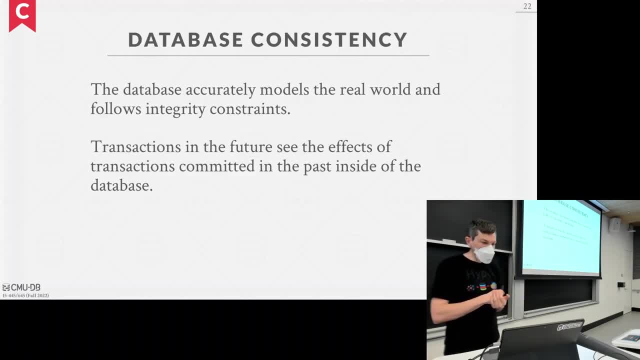 we don't. the system just doesn't under the semantics of the correctness again. so the first example I said about, like the, the modeling, the class, this is what it's called database consistency. so it just means that the database is going to accurately reflect, whatever the thing. 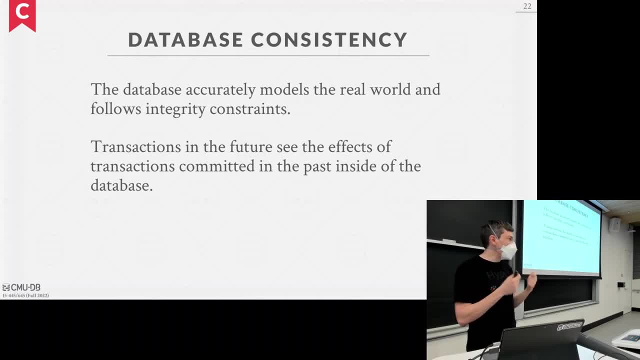 it's trying to model in the real world and it doesn't violate any integrity constraints, like a student can't be enrolled in the same class twice in the same semester, right, and so we, the data system, couldn't enforce that. if you try to do something and then any transactions. 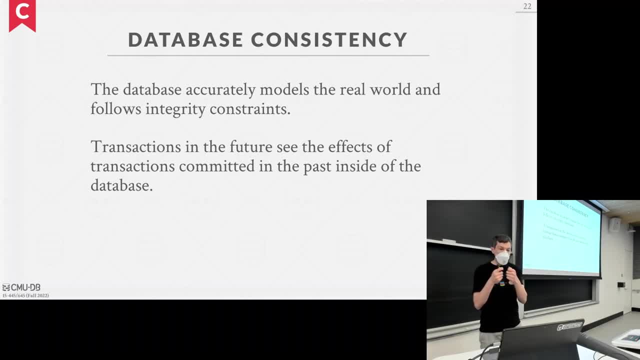 that makes a change to this database. you know any, when a transaction makes a change to the database, any future transactions will see those changes, assuming they weren't overwritten. right, but the things will persist right. so again for a single node database. maybe this doesn't make sense. 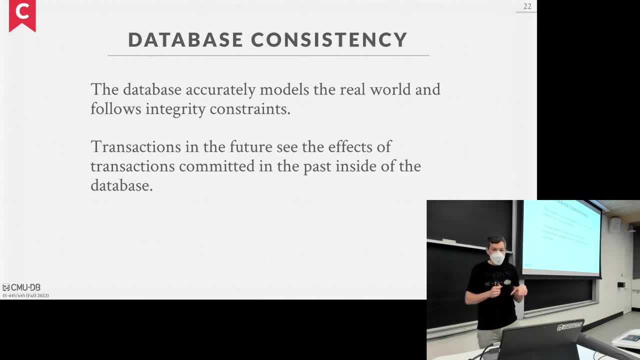 like: yeah, of course, if I insert a record I should be able to see it right. this will make more sense when we talk about distributed databases, where if I insert a record onto, say, a database is stored across multiple machines. if I'm told my transaction commits, then I should be able. 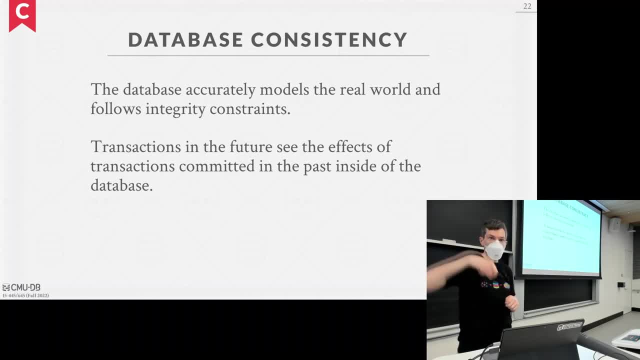 to immediately see that change on the on another node right for a single node again. it's sort of sort of weird. but again, distributed databases if they have strong consistency, they will provide that guarantee and we'll cover that how we do that, I think, after Thanksgiving: transaction consistency. 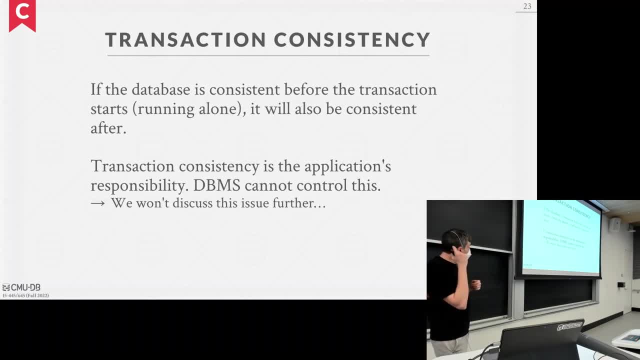 this is the one that's real fuzzy. it basically means that if the database is consistent before the transaction runs and if the transaction does consistent things to it or is consistent, then the end state of the database after the change will be consistent. right, so it's subjective. 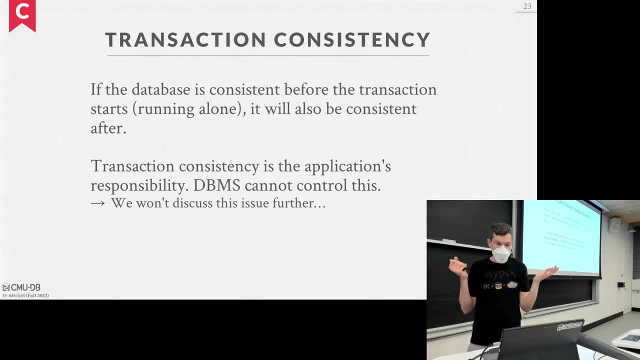 because, like the, the, the database that doesn't understand the semantics of the high level meaning of the changes that the transaction is making. again, like well, student can't be enrolled in, can't be enrolled in the same class twice. so like you can put, you can put. 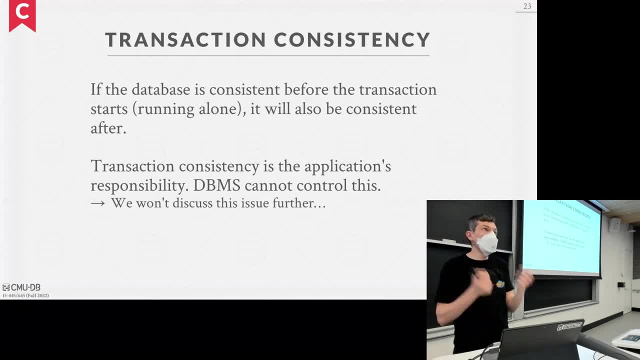 integrity traits for that, but, like a student, shouldn't be enrolled in the class if it appears on a Tuesday because of you know they have some allergy or something like that. right, that's a high level thing that you wouldn't model in a database that only the application. 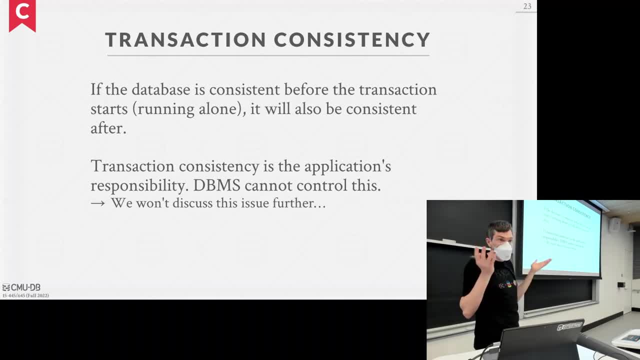 or a human actually could know, and therefore, if a transaction violates that, then the database is technically inconsistent, but we just don't know that. yes, so like an example, like if when you give a, like you have $100, someone else has $100 at the end of it. 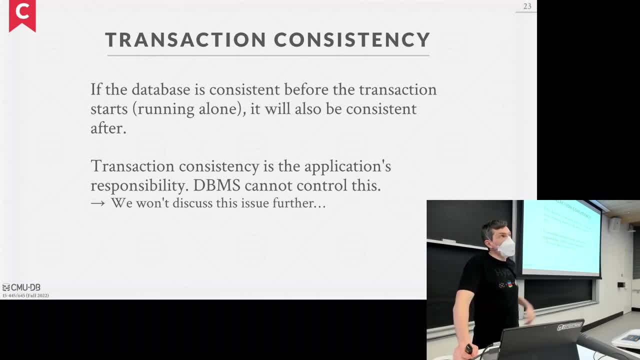 that comes under the transaction. this question is, in my example of of transferring the $100 out of my account, the notion that the when a transaction commits that $100 has to be somewhere. that would be database consistency, because there's integrity constraints we can put in place. 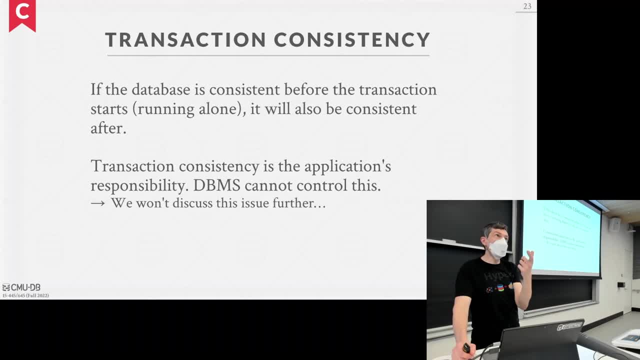 to make sure. well, actually, no, I take that back. it'd be. it'd be database consistency, because we don't. these are all tied together because you don't want to allow for the partial updates. so if the transaction commits, it has to be somewhere again. let's not get hung up. 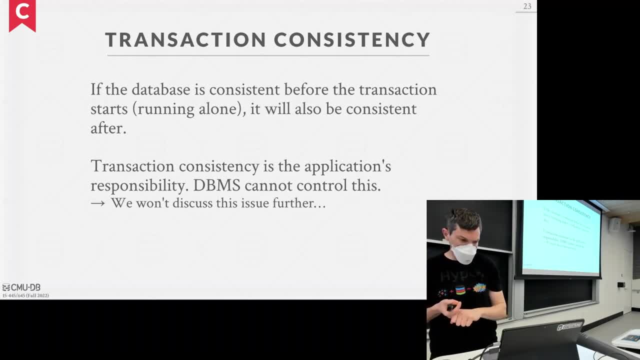 too much on consistency here again. for distributed databases it'll make more sense, but again, in general, integrity for transaction consistency. the data system doesn't control it, we can't enforce it, so it's again. this is more a theoretical thing, not something that any system would actually do. 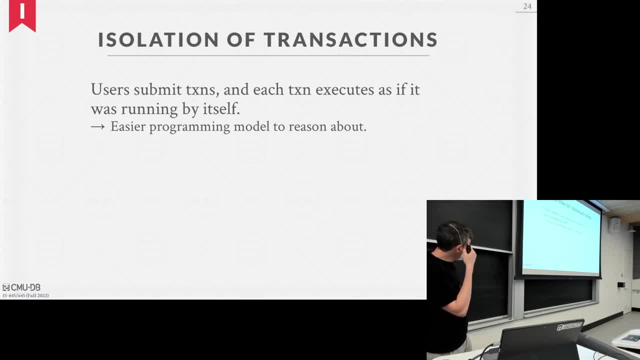 all right, so let's. we're gonna spend most of our time talking about isolation levels or isolation, so the. the thing that we want to achieve is that when an application or user submits a transaction, we want that transaction to execute under the illusion or the the idea. 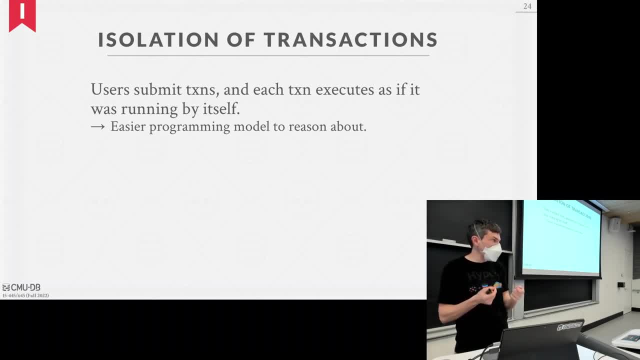 that it's running by ourself, running by itself. there's no other transaction running at the same time and therefore we won't see any updates from other transactions and we don't worry about them- sort of clobbing our- our updates, right? the reason why we want this. 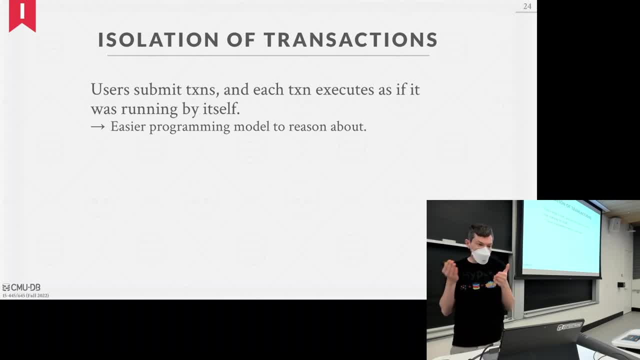 is because it's a way easier model to have, because now in your, in your application code you don't worry about. you know, should i be seeing things in my database that i i shouldn't be seeing? like if i, if i write data, i should, you know. 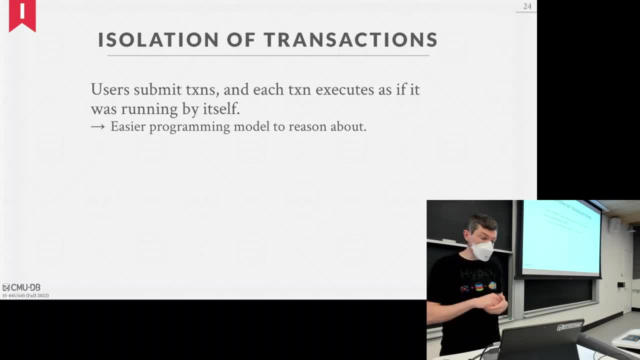 i should read my own rights. this sort of seems kind of obvious, but the the whole no sql movement was all about not doing this and you had to write a bunch of extra code to deal with eventual consistency or deal with, uh, the lack of isolation of transactions. 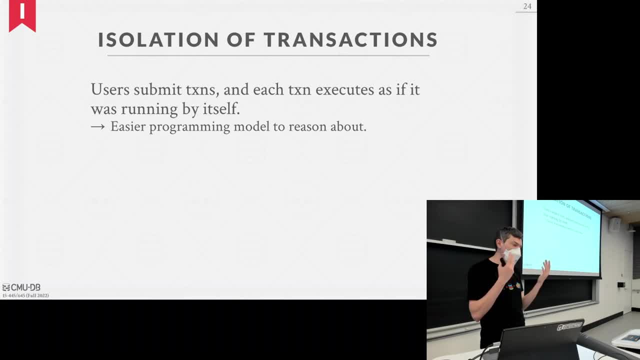 uh and, and you would run out of application code because maybe i could write something and not get back my own right. i may actually get back a series of rights- i got to figure out which one i actually want to look at- or series, a series of values. 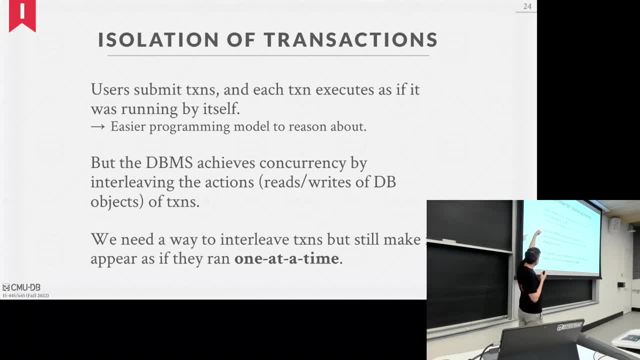 right. so the the challenge is going to be that we want to achieve this. we want to have transactions, think they're running by themselves, but, as we said, we want to interleave them. uh, the reads and writes- are transactions that running at the same time, because that's going to give us 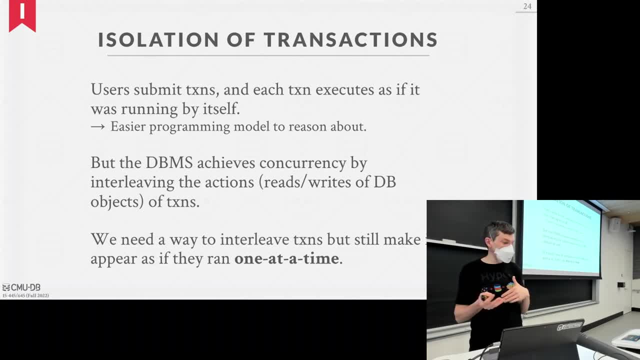 better concurrency or better parallelism, to be able to interleave our transactions in a way that they appear or they make changes to the database as if they were one at a time, running in serial order. but we were actually able to interleave them And we still wanted the database to be correct. 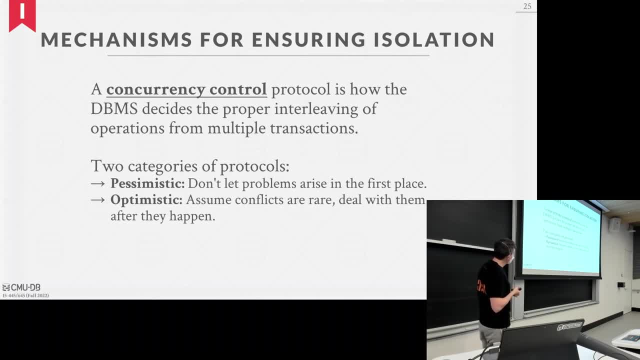 So this is what the concurrential protocol, concurrential scheme, is going to provide for us. You can think of it as a traffic cop that's going to be responsible for deciding at run time what operations from what transactions can do what things on what different database. 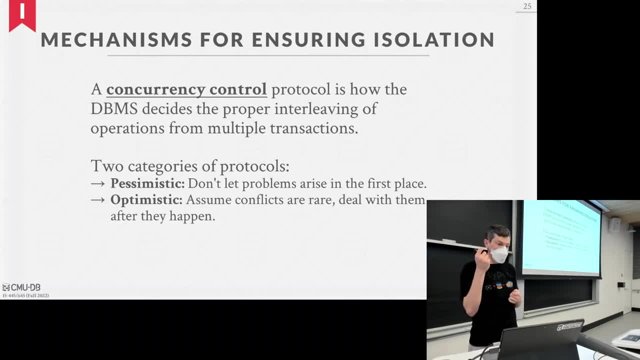 objects And it can sometimes deny the request or it can allow it and then later on say you shouldn't have done that and go ahead and abort you. So there's two categories of these protocols. He actually asked about this earlier, like why can a transaction go to commit and it isn't later decided to abort it? That's an. 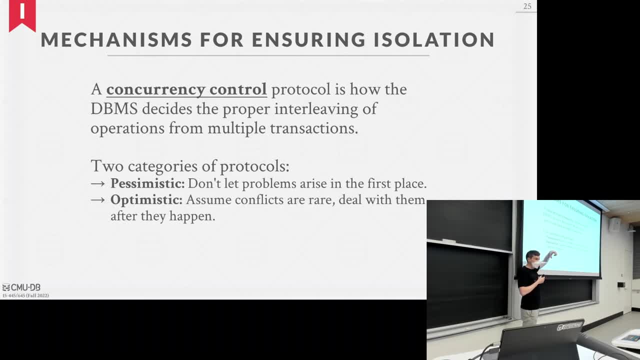 example of optimistic concurrential control, because you're going to assume there's going to be conflicts are going to be rare, So you let anybody do whatever they want and only when they go to commit you look at the things that they actually did and say, okay, that's. 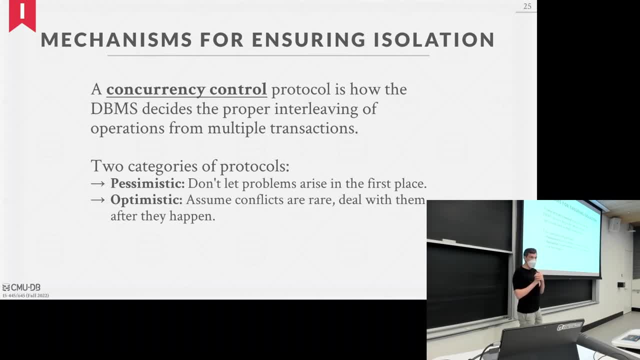 okay, You can commit or no. that wasn't okay. You have to abort. Pessimistic concurrential control would be. I assume the problems are going to. I'm assuming I have a lot of problems, So I'm going to require you to require transactions to acquire. 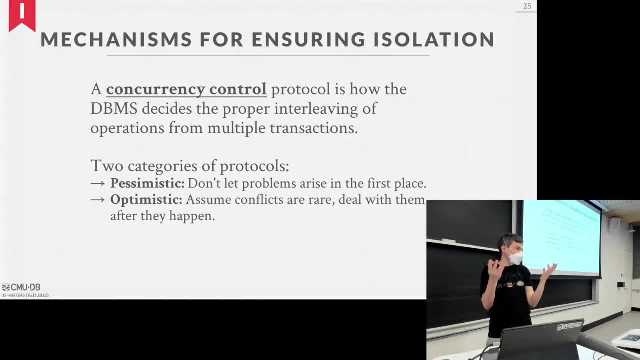 locks on objects that they want to touch before they do anything. And that way I know that if you have a lot of problems, you're going to have a lot of problems, So I'm going to require you to have a lock on something You're allowed to do, whatever it is you want. 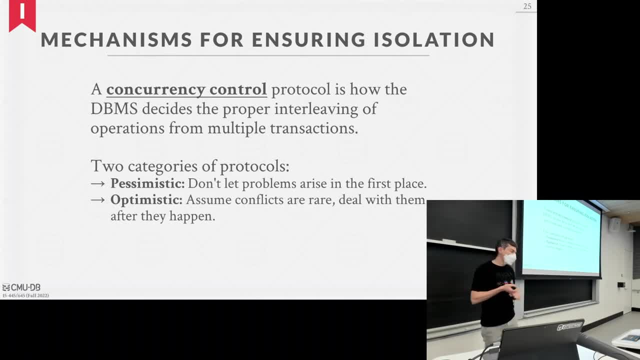 to do on it. So in some cases optimistically better, other cases pessimistically better. At the end of the day, if you have the worst contention possible, like you have a million transactions all trying to update a single tuple, these things basically are the same. 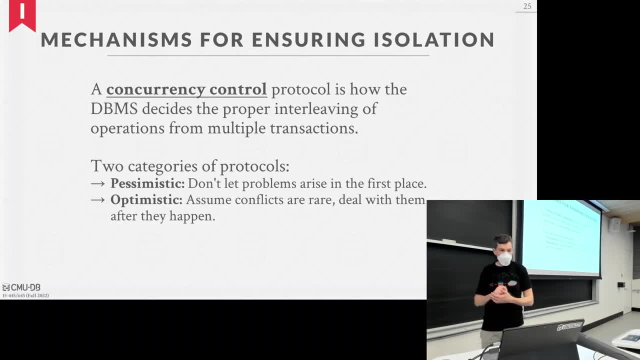 thing. It doesn't make a difference. So we probably want to mostly think about how to do this on the average case, And none of this comes to free. Just because it's optimistic doesn't mean it's magically faster than pessimistic. But at the end of the day, there's always bookkeeping. There's no free lunch in databases. 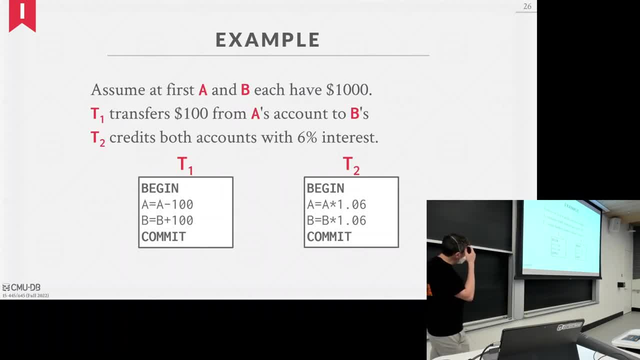 All right. So let's look at an example here. We have two transactions now And we have two accounts, A and B, And they both have $1,000.. So what we want to do here is: we want to take a- we have the first transaction- wants to take $100 out of A's account, put $100. 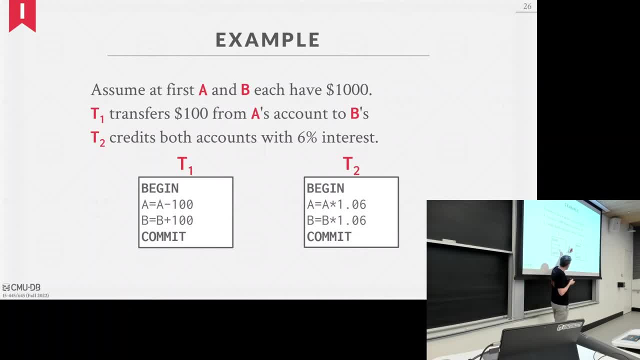 back into B's account And there's another transaction that wants to compute interest on the bank accounts and give them. everyone gets 6% Right, All right. So what are the two possible outcomes of running a t1 and t2.. Assume these things are committed or submitted to the data center. 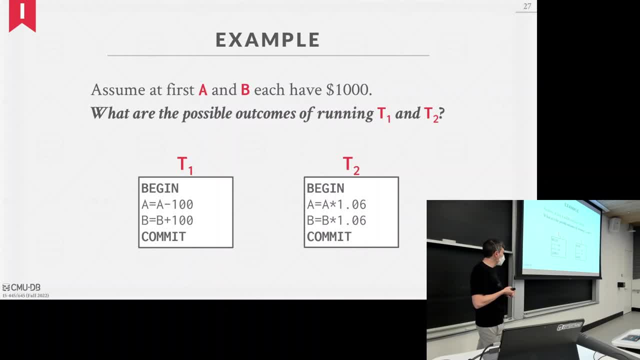 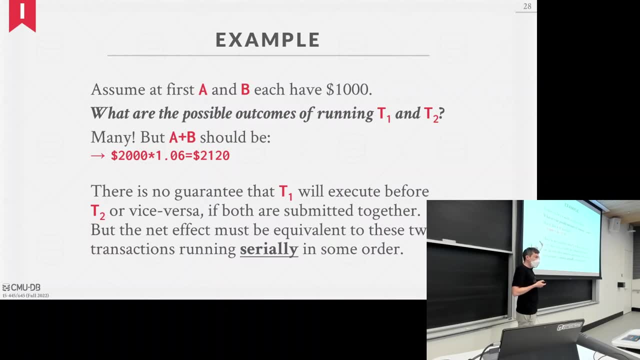 at the exact same time by two different threads or two different clients, Right. What are the possible outcomes? Well, in this case, here there was many ways to interleave these things, but at the end of the day, we need to guarantee that if we add A and B after, 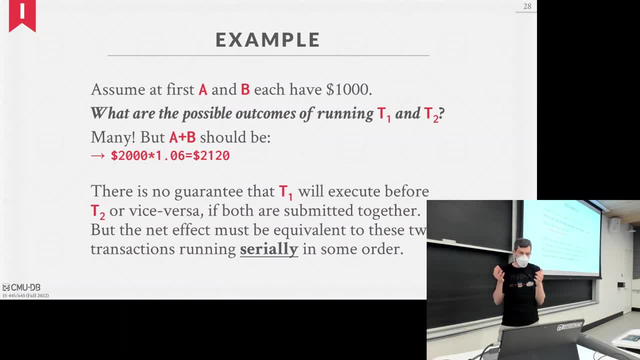 executing T1 and transaction T2.. That the only consequence is that the price is not just the price all of a sudden, but the entire price side down. So simply have a non-pay guerrilla contract. here I mean many times, but that changed. This is a similar example where you're saying: 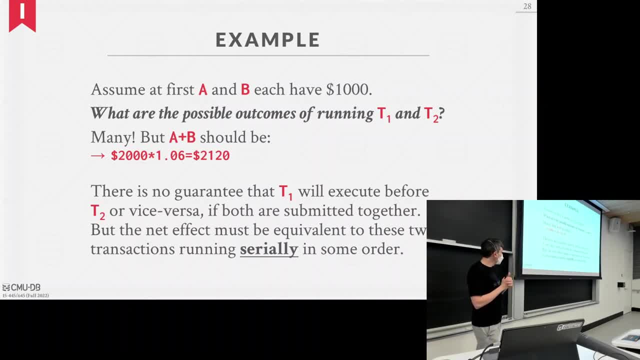 total amount that's in the bank for both accounts is 2120.. So the data system is not going to guarantee that just because T1 gets submitted before T2 or T2 gets submitted before T1, it's not going to guarantee that it's going to execute those things in exactly that order. 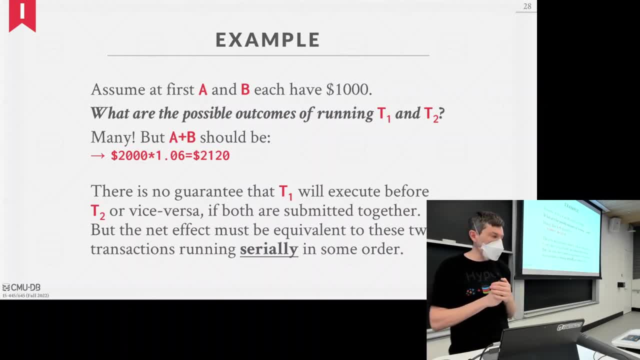 And this is going to be slightly weird when you think about maybe other parallel programming you've done where there's memory barriers, or x86 is very, very cautious to make sure you get things executed in the right order. In our world of databases we can actually 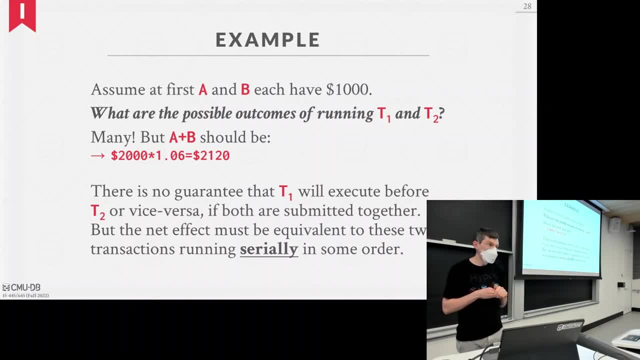 interchange these or interleave these any way we want, But at the end of the day, we just need to guarantee that, whatever the state of the database that we end up with for our interleaving is equivalent to executing the transactions in serial order. So either T1 followed by T2 or T2 followed by T1. 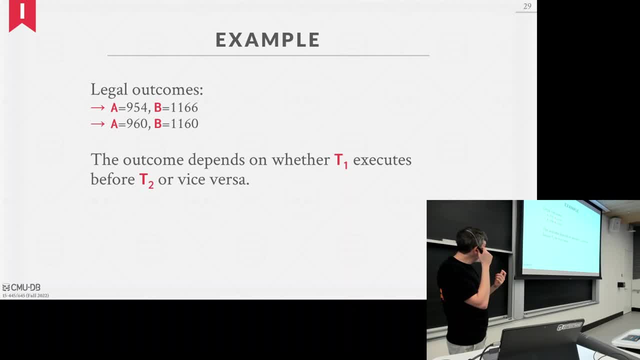 Right. so the possible outcomes we have for this: if we execute T1 first, followed by T2, we would have 954 and 166.. Or if we execute T2 followed by T1, we would have 960 or 1160.. At the end of the day, when we add them up, it's always 2120.. 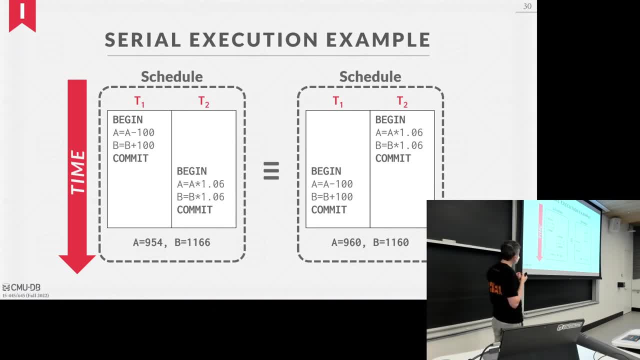 So let's see what this looks like visually. All right, so here's the two serial orderings for the two transactions. So I execute T1 first followed by T2, or execute T2 first followed by T1.. But all that matters again is the values of A and B. 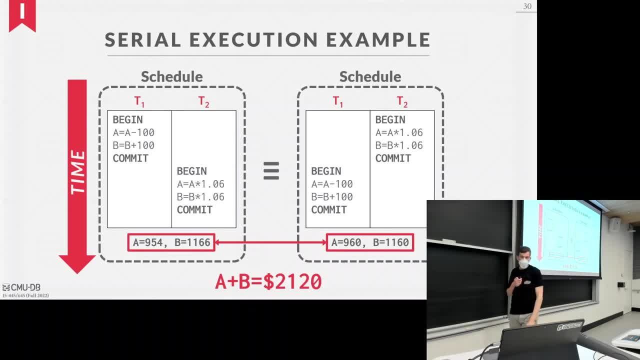 when you add them together equals 2120.. Both are correct, even though A has less money in one and B has more money in the other. But from the database system perspective these are both valid. These are both correct orderings, All right. so we talked about before why we want to interleave the transactions. Why we want to do this? because we want to avoid blocking or stalling because of slow disk and network. That was the big deal that they cared about in the 1970s. right, Because disk was super slow, You had limited memory And so you have all the time transactions that had to go stall. 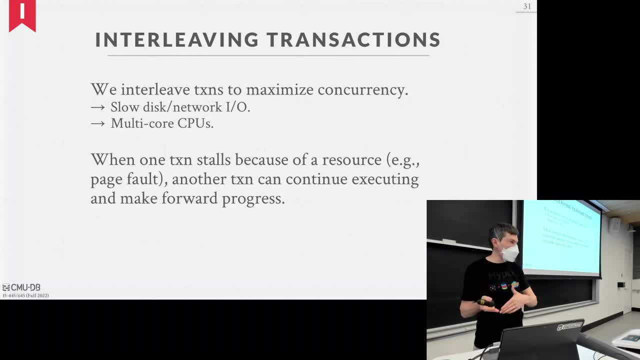 because they had to go fetch things from disk. So, even though you only had one core in your CPU, you could then pick up another transaction and run that while the other transaction was waiting for its disk. In modern systems, the disk has gotten faster, Memory has gotten larger, But 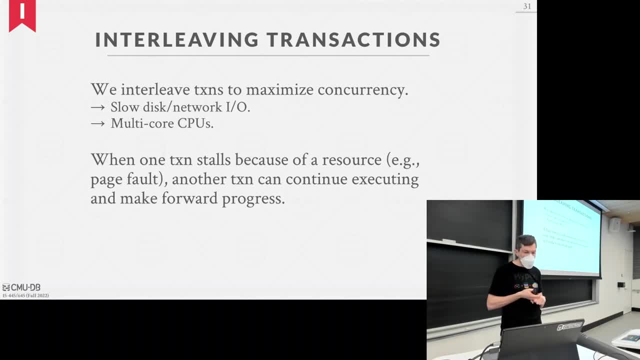 for OTP systems you want to kind of keep most, if not all, the database entirely in memory in your buffer pool. But now you have these multiple CPU cores and you want to take advantage of those. So this is why you want to start interleaving transactions as well, right? 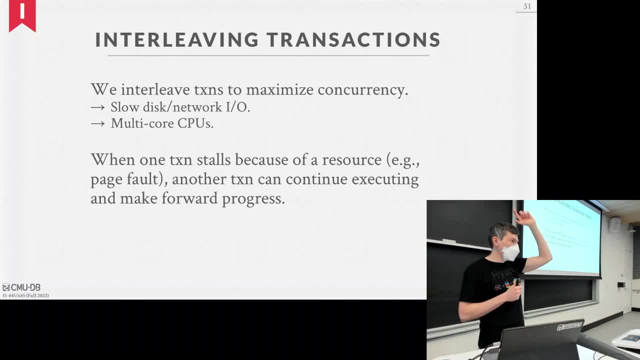 Maybe one transaction stalls because it's waiting on a latch or a lock, and then you let another transaction on another core keep running. Well, we want to make sure that we give the appearance as if they were executed in serial order. All right, so let's look at a good interleaving. 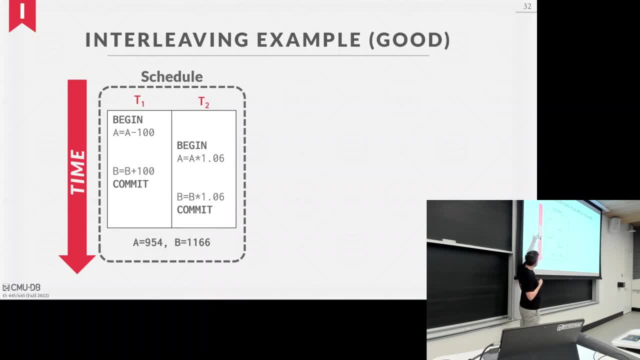 So in this case, here we're going to execute T1. first It takes $100 at A, But then there's a contact switch, for whatever reason, Maybe it stalls in disk, Maybe the OS swaps it out, Whatever, It doesn't matter. But then T2 starts running. It then computes interest on A, Then there's a. 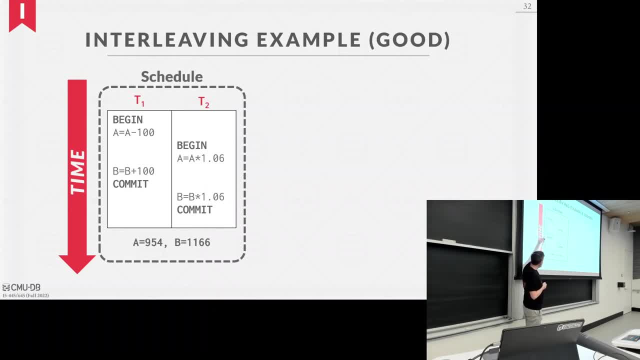 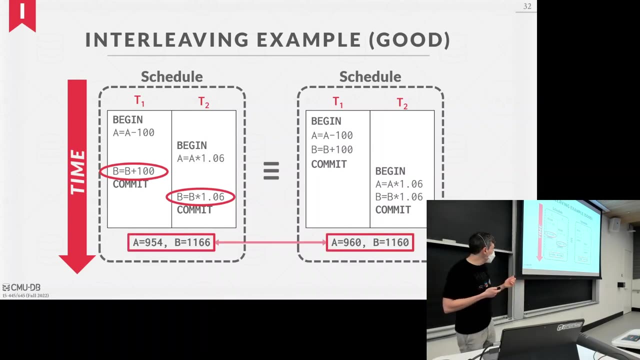 contact switch back to T1. We put the $100 back in B Contact switch back into T2. And it computes the interest on B right. This is equivalent To executing T1 followed by T2, right, And the basic idea here is that we're always 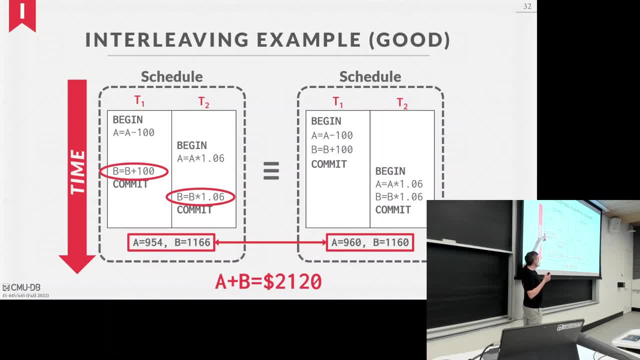 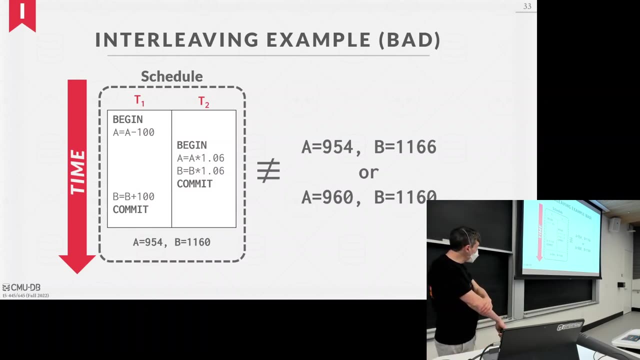 guaranteeing that we compute the interest, the deduction or addition on the account in T1 before we compute interest in T2, right Or likewise we could well. if we do something like this, right, the outcome is not equivalent to the interest on B, So we're going to do. 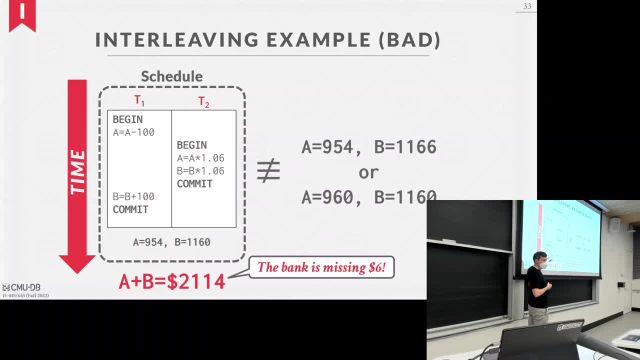 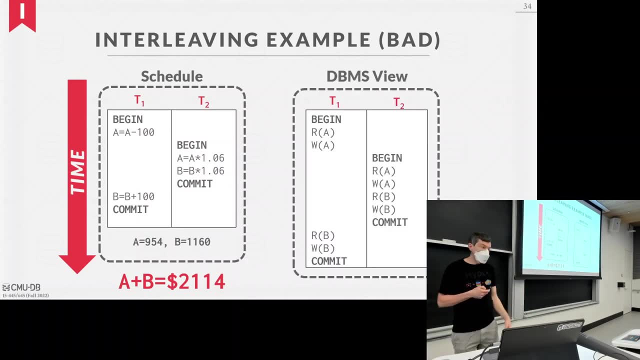 the two possible serial orderings And we end up missing $6 in our total, which is bad Right. So now the database system doesn't see again these operations like: B equals B plus 100.. So it can't do any tricks like: oh these are commutative. Let me play some game like that. 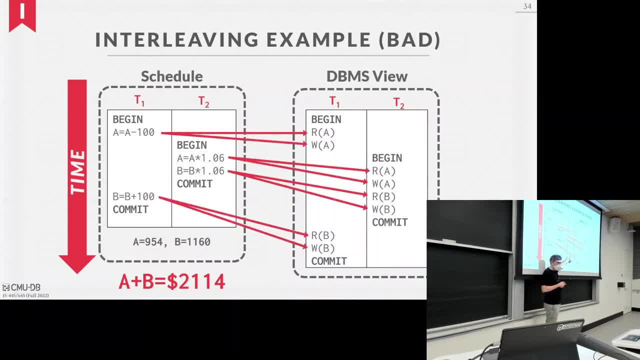 Right. All it sees is these read and write operations. So again, it doesn't understand the high-level meaning of what the. if I read a record, what's it actually going to do with it when it writes it back? We don't know. 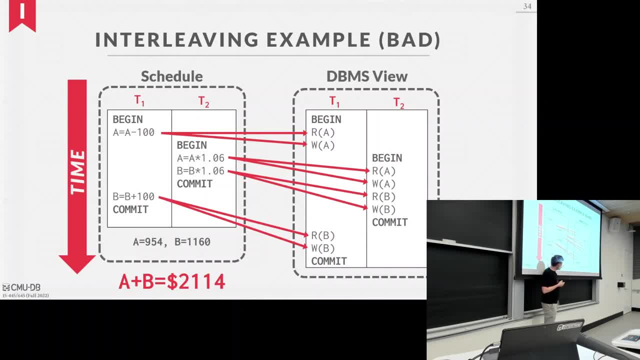 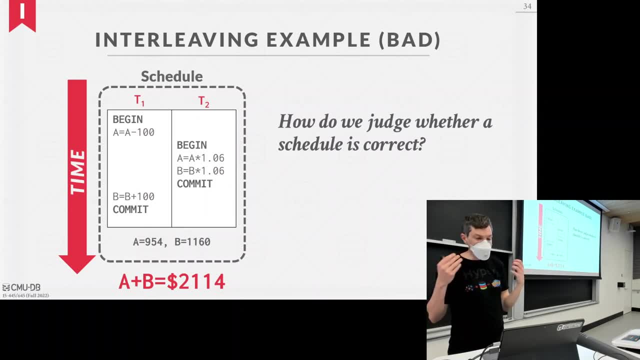 We don't know that because that's over an application code. So we only see these little things and we have to deal with this. So we need a way to actually program or we need a programmatic way to understand and reason about whether an interleaving in a schedule is actually going to be correct. 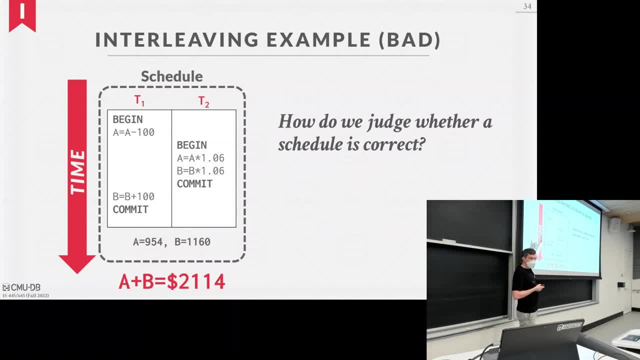 Like visually. I'm just sort of pointing at stuff and drawing circles. We can kind of see how this would be problematic. But this is for two transactions and a pretty simple schedule. I need to be able to reason about this at a large scale, So I'm going to use 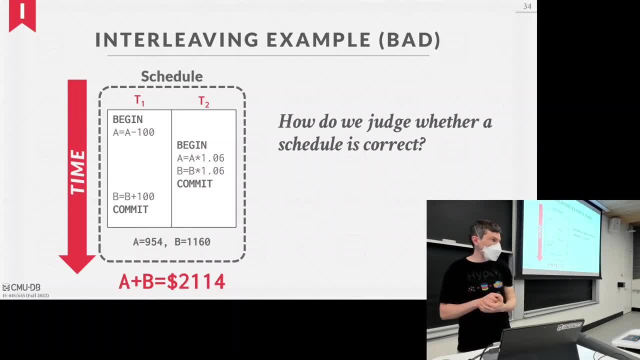 this as a way to understand and reason about whether an interleaving in a schedule is actually going to be correct, larger scale, and obviously do this in a way that's you know that a program can run or a database system can actually run. 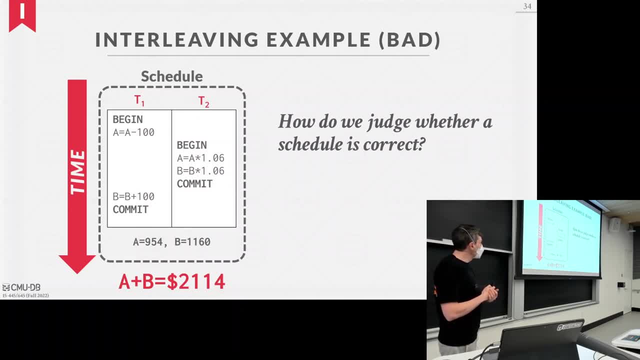 Yes, If you actually run this in Postgres, will it ever give you this bad result? The statement is. the question is: if I actually run this in Postgres or really any database system, could I end up with this result? 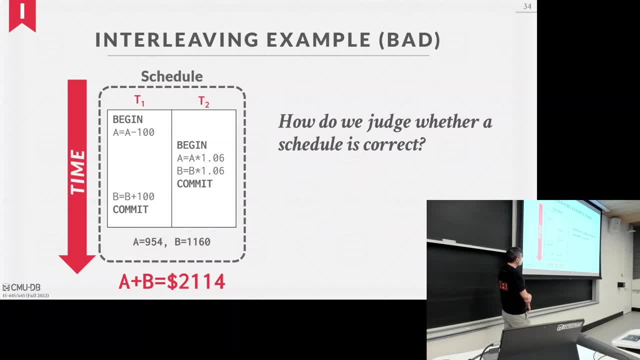 Yes, if they're not doing, if they're not running, if the curse curve protocol could potentially allow this, if you turn off locks and other things, You could yes. So basically, would transactions do this isolation checking for us? Would you say transactions? 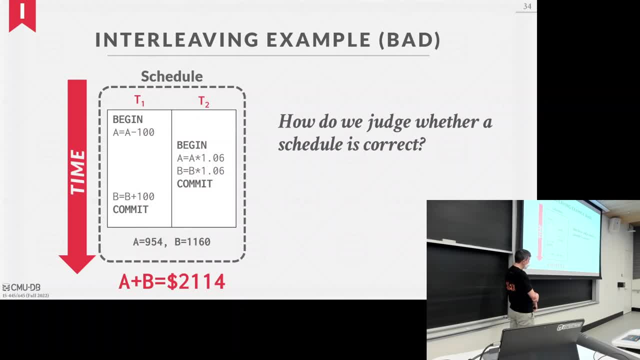 would the data system do this for you? I guess you're saying if you turn things off it doesn't do it, but if you leave them on it would do it. Yeah, but I'm telling you how to turn them on. 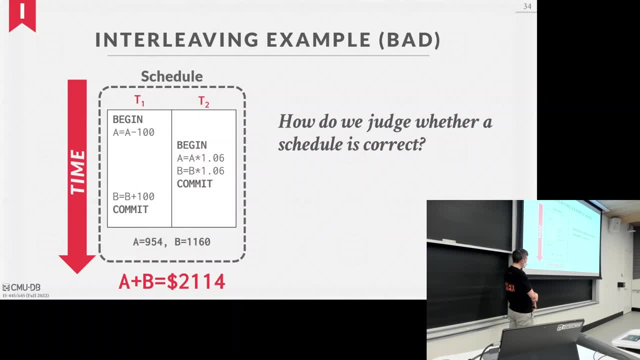 I'm telling you how to implement the thing when you turn them on. That's what this is. Yeah, Like the application code isn't going to have, you don't want people writing their own application code, doing the checks and say, oh, did this happen before this? 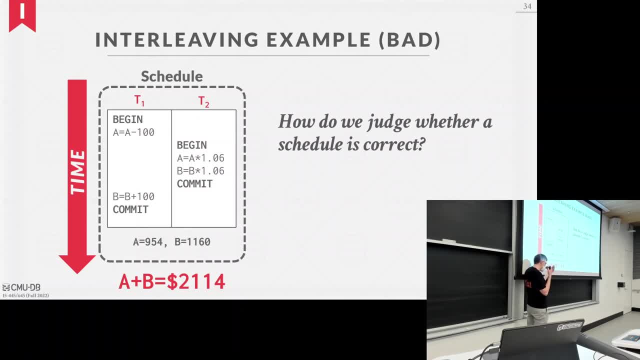 Because there's no guarantee that you're always going to submit the two transactions at the exact same time. What we're trying to discuss today is: how do we understand what does it mean to interleave things and end up with the correct state- Next class? so this would be like: 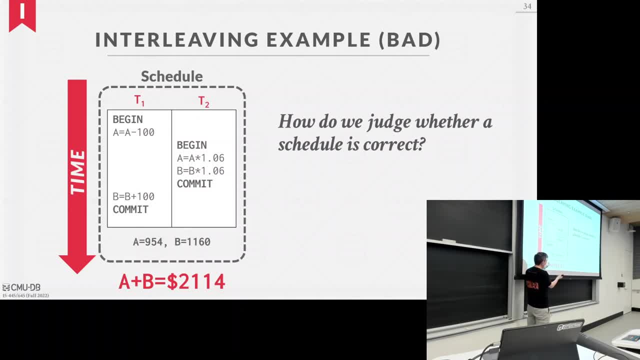 when I give you the schedule and I give you a fixed set of database objects. next class would be: if I'm getting incremental queries or incremental read-write operations, how do I guarantee that I end up with a schedule that is correct? All right, so what we're going to find? 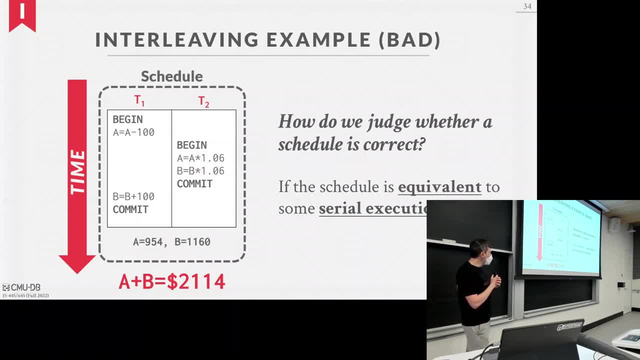 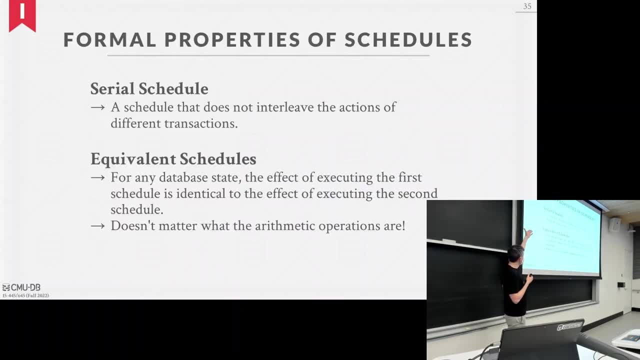 is that we're going to say that a schedule will be correct if it's equivalent to some serial execution. So we've already said sort of what a serial schedule was. There's no interleaving. We're executing the transactions one after another And we're going to say a schedule is equivalent. 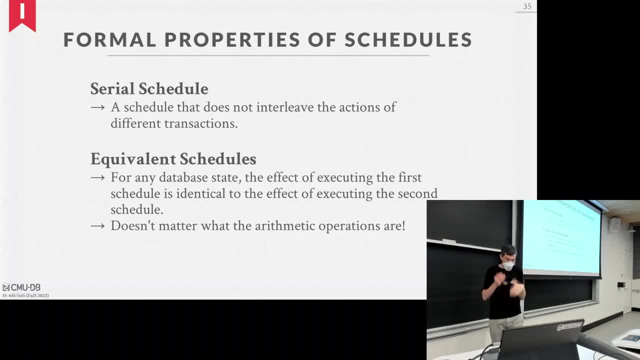 if the schedule is equivalent to some serial execution. So we're going to say a schedule is equivalent for any given database state as the input, the effect of executing the transactions in a schedule end up producing a new database state that's equivalent to the other schedule. 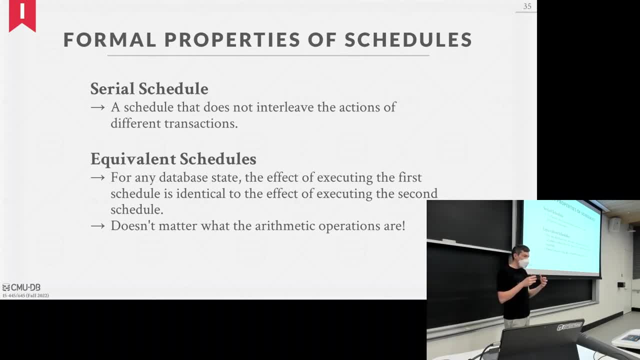 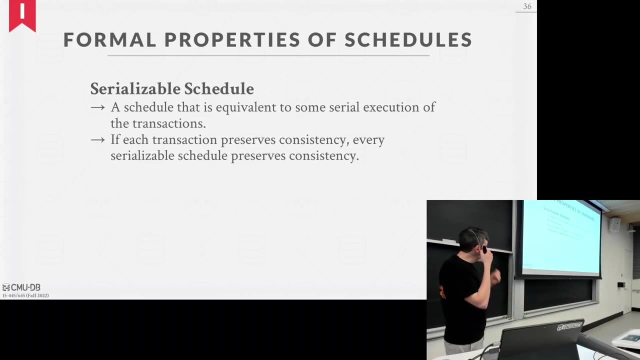 And again, these are low-level read-write operations. We don't actually care what the, is it addition, multiplication, whatever it is on these objects? It doesn't matter. We want to have the state of the objects be the same, And so the gold standard. 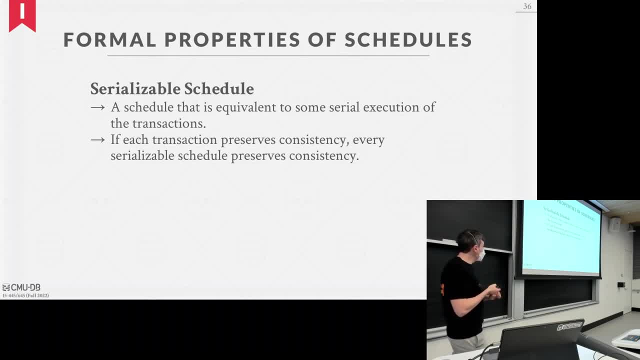 what we want to achieve is what is called a serializable schedule, And this just means that the schedule, with its interleaving, will be equivalent to a sum of serial execution of the transactions. right, And so obviously this means now if the database is consistent. 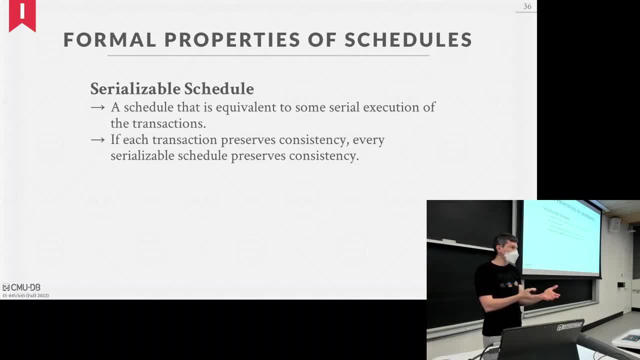 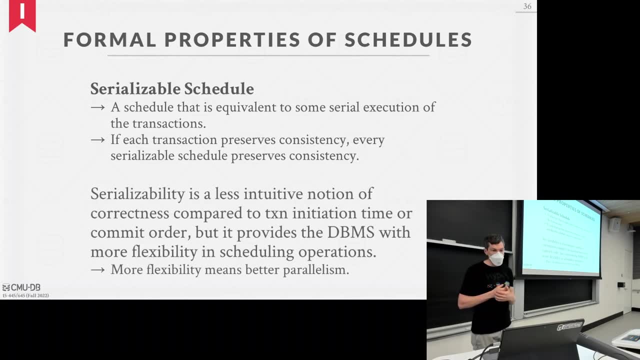 the transaction is consistent, then the serializable schedule that we would choose or use would guarantee and preserve that consistency. So, again, as I said before, this is kind of a weird concept where I could have transactions get submitted in one order, but I'll commit them and apply their changes. 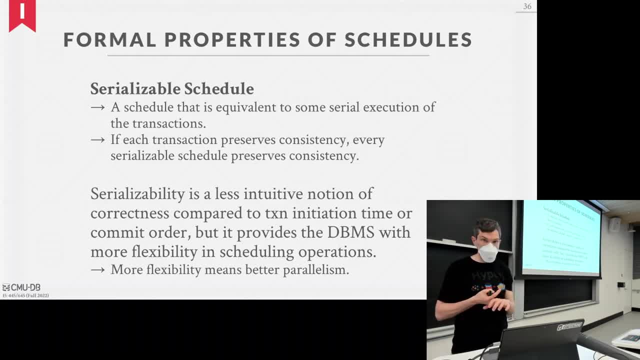 in a different order inside of my database system And that's okay. And we want that in our database system because it'll guarantee that it gives us more opportunity to come up with different interleavings to maximize the amount of parallelism we could have. 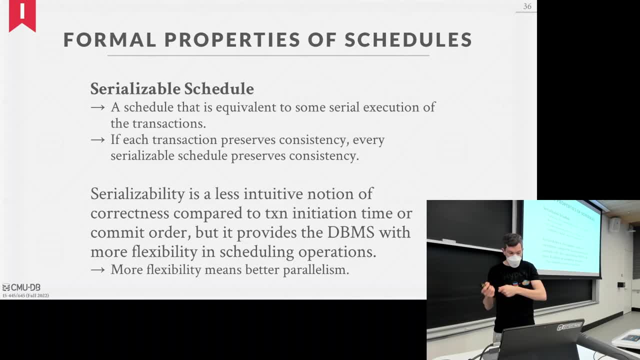 If you cared about the ordering of the commit order of transactions based on their arrival time, then you either do that in the application with your own barrier that says: okay, I submit T1, wait till it comes back, then I submit T2.. 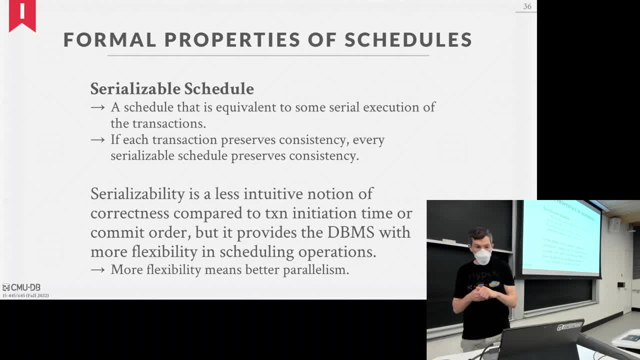 Or there are some systems which they're rare. there are some systems that will guarantee you that the commit order will be the same as the arrival order. That's called strong serializability or external consistency. There's not many systems that do this. 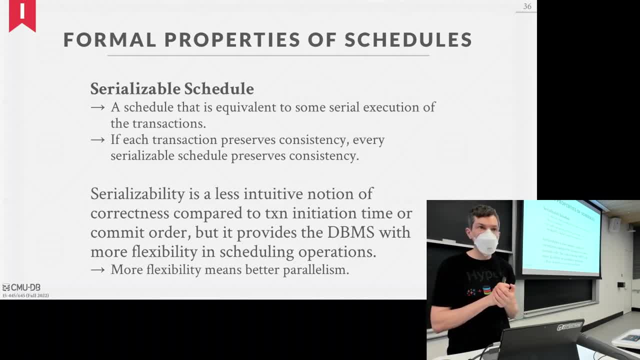 Google, Spanner and Faun are probably the two main ones. Question: Yes, I just wanted to ask at a high level: why are we calling this isolation, like even in this slide, although it's a transaction that's consistent? why are we calling this isolation? 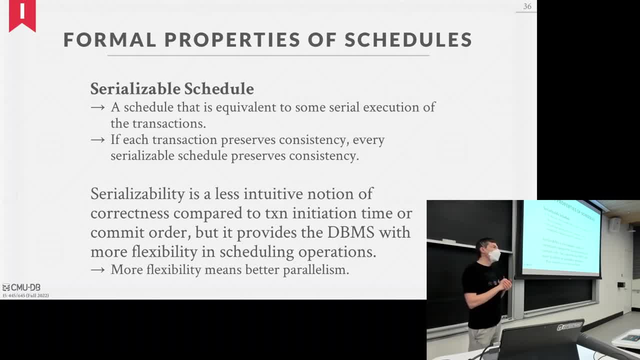 to token amount. His question is: why are we saying this is why make a big deal that this is isolation, not consistency? Because it's the- if you can, normally this sentence here. we want this, we want this, which means the state of the database. 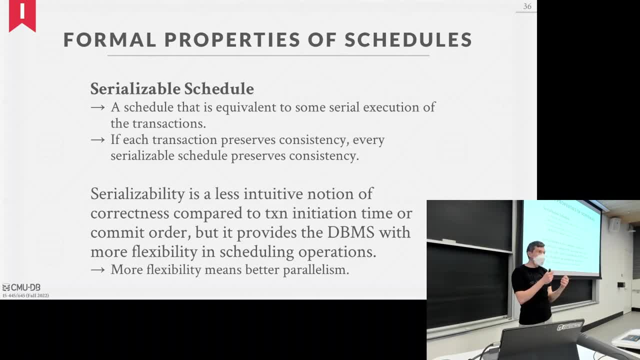 to be as if we're executing them in isolation of others, And that means that not only do we end up with a serialized, with serial ordering or cereal equipment or serial quiz, let's say sterilizable ordering or schedule that. that's part of that. 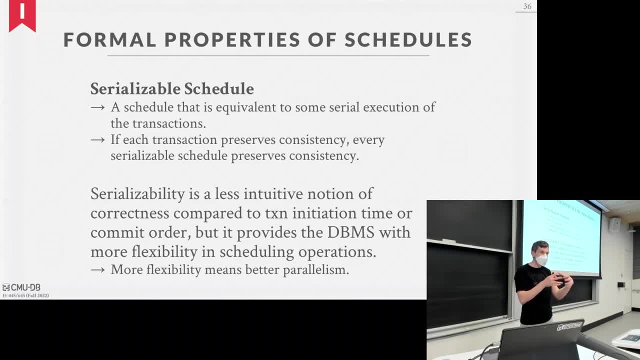 we're not be able to see any effects of any transactions or running the same time as well, So I'll guarantee the state of the database at the end is equivalent to a serial ordering And while it's part of it, while I'm running. 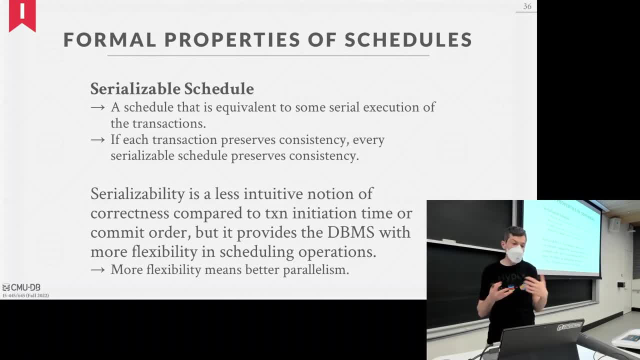 I won't see the effects of anybody else running the same time as me, Because consistency basically means that like it's part of that, like the data, if it was correct when it started, it's correct when it's afterwards, even though I interleaved things. 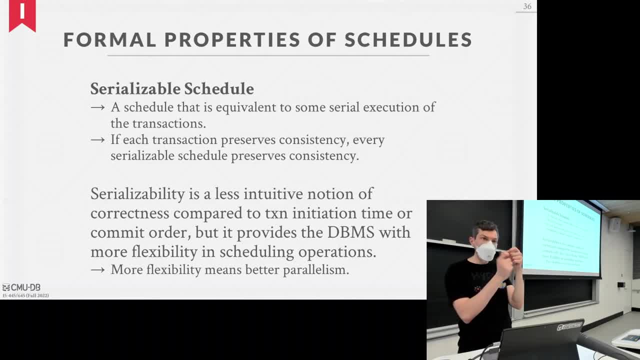 But again, as I said, you could have temporary inconsistencies, but that's okay At the end, as long as everything's consistent, that's correct, Okay. so, as I said, most systems don't guarantee that arrival order execution. Again, Spanner does this. 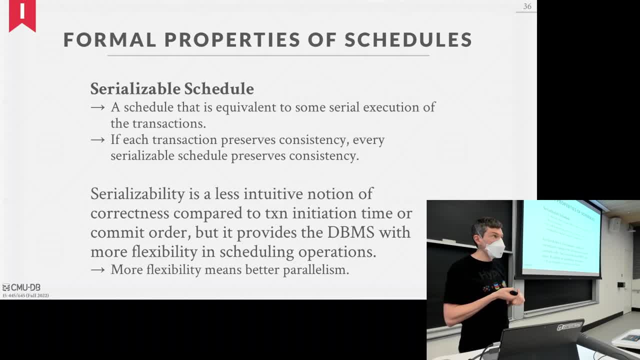 They claim their paper for Google Ads. It's a big deal and that's why they need it. I don't know if that's actually true, but, as they said, most systems don't do that. Actually, most systems may not even give you serializable execution that we're describing here. 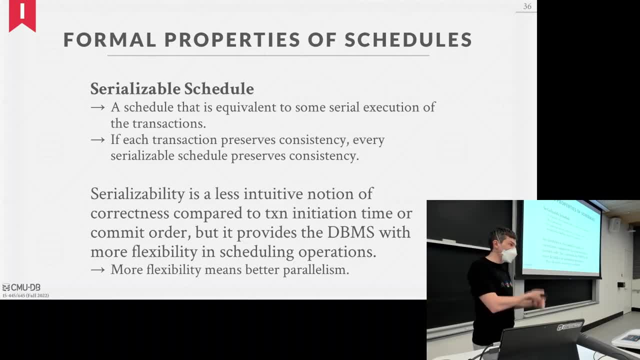 It's not all: by default in most systems, If you ask for a serializable in Oracle, they'll lie to you and actually give you something weaker. But in general, like this is the gold standard, because this is guaranteed not to have any anomalies, any problems in your application code or in your transactions. 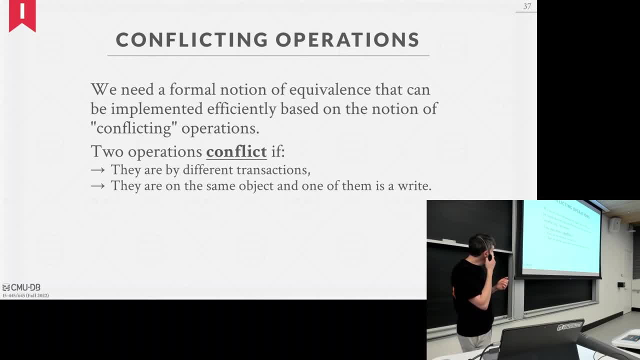 All right. so now we've got to define. what does it mean to have? you need a programmatic way to say, okay, can we have this transaction or is this schedule actually serializable? So what we're going to do is we're going to identify the conflicting operations in two schedules. 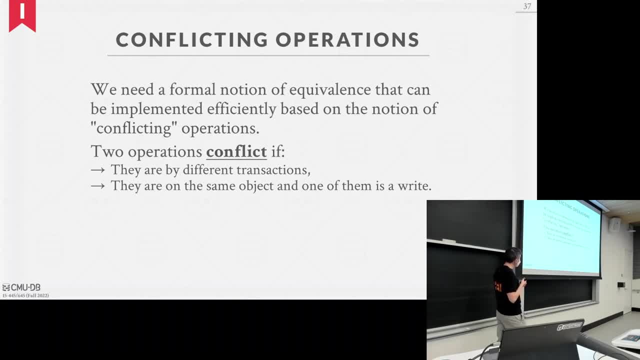 Or sorry, in one of our transactions or two of our transactions, And we're going to say that the operations are going to conflict if they occur in different transactions and they're accessing the same object and at least one of the transactions is doing a write on them. 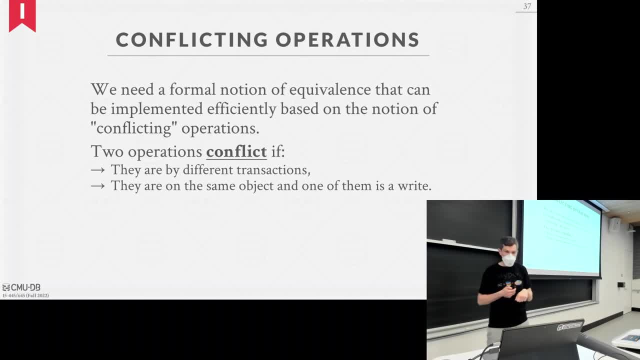 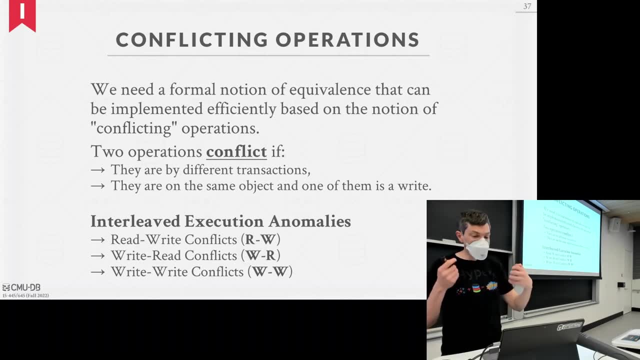 Right, you could have a read-write, write-write or a write-read And then we can look at these conflicts and identify what are some of the anomalies that could occur. that should not occur would not have occurred if it was actually a serial ordering. 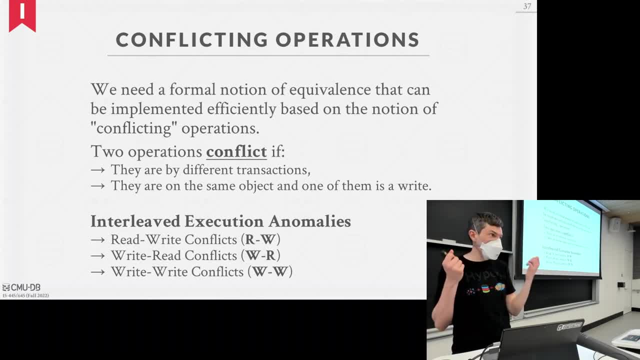 And if we can identify these anomalies, then we would know that they're not serialized, We would know that this is not a serializable ordering or, sorry, a serializable schedule. So I have the three sort of three basic anomalies: read-write, write-read and write-write conflicts. 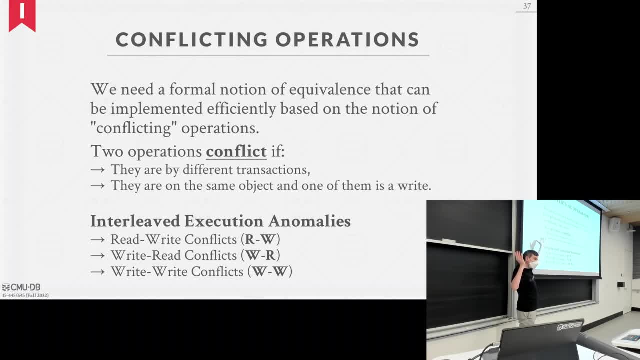 There's no read-read conflict, because obviously, who cares if you and I read the same thing? That's not a conflict. There are two additional anomalies that we'll cover next week- phantom reads and write skew- But for our purposes here we can focus on the three main ones. 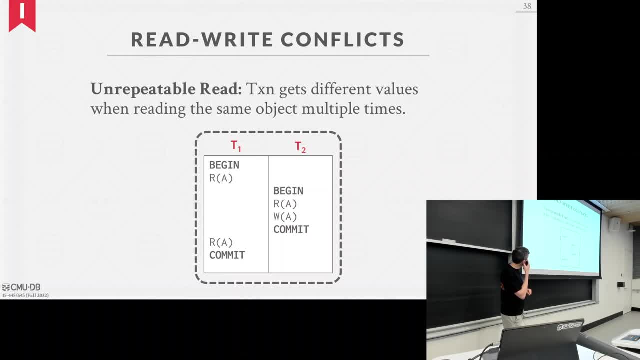 All right. so the first one is a write-read conflict, also known as unrepeatable read, And this means that a transaction tries to read an object multiple times while it's running and it gets back a different value at some later point. 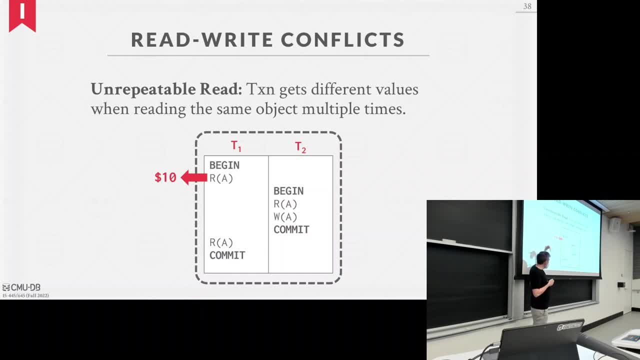 All right. so T1 starts, it reads A, gets $10.. Then there's a context switch: T2 starts running, it reads $10 as well, but then it writes back $19.. And then now, when this transaction reads A again, now it sees $19. 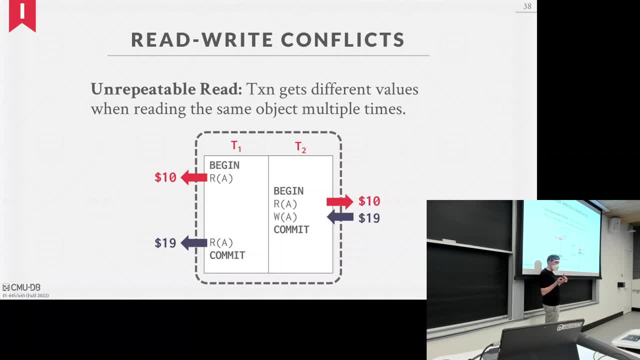 And it shouldn't right. If it was truly running in isolation of any other transaction, It would see $10 again, Right? So this is called an unrepeatable read. Again, this would violate a serial ordering. A write-read conflict, also known as a dirty read, is where one transaction reads data from another transaction that hasn't committed yet. 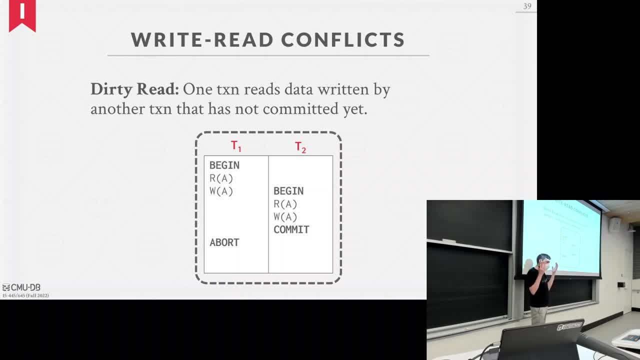 And then say that other transaction then does some action based on that dirty data that it shouldn't have seen. So we read $10 here, write back $20.. Then we read $12, then there's a context switch: T2 starts running, it reads the $12 that T1 wrote, and then there's some additional logic or something where it says, okay, well, let me add $2 to it. 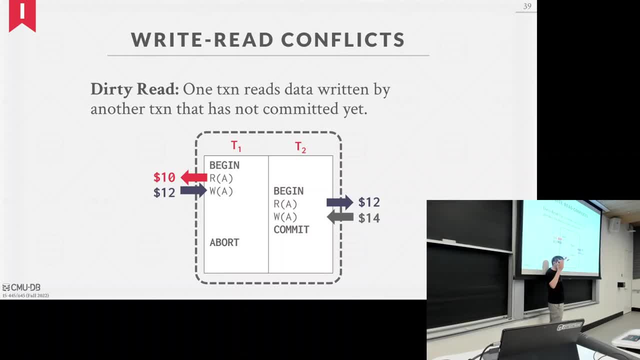 Now it's $14.. It goes and commits And, assuming, at this point here we tell the outside world: yes, your transaction has committed, T2's done, you're good. But then T1 aborts and now we've got to roll back the change that it made in A. but we've already leaked to the outside world the write that T1 made. 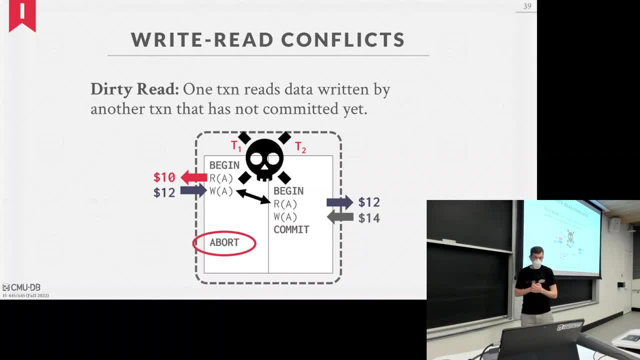 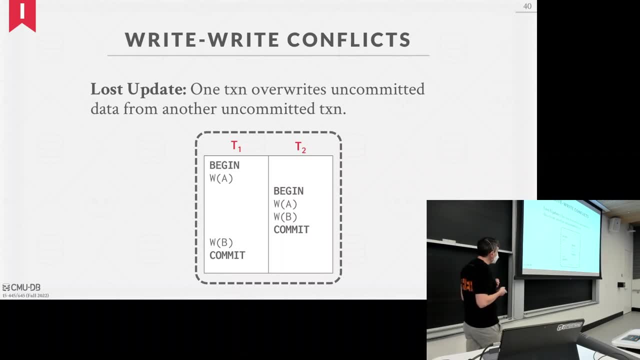 And that shouldn't have happened if it was running in serial order. So this is bad. We don't want this to happen. The last one is a write-read conflict, also known as a lost update, And this is where we have a transaction that's allowed to overwrite uncommitted data from another transaction and you can potentially end up with torn writes. 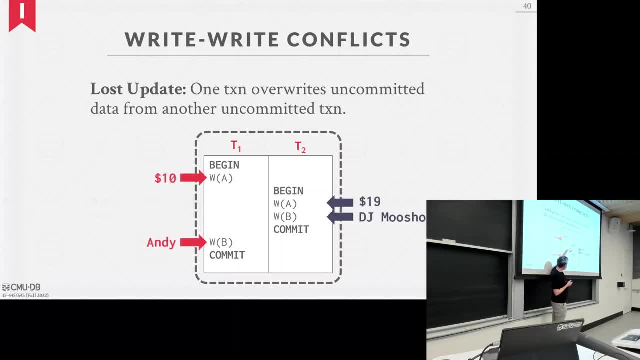 So T1 starts, does a write on A, T2 starts, overwrites on A, then writes on B and adds a DJ Mushu. And then T1 runs again And now writes Andy. So in this case here you would have: the value of A would have been written by T2, but the value of B would have been written by T1, which shouldn't happen if there was a serial ordering right. 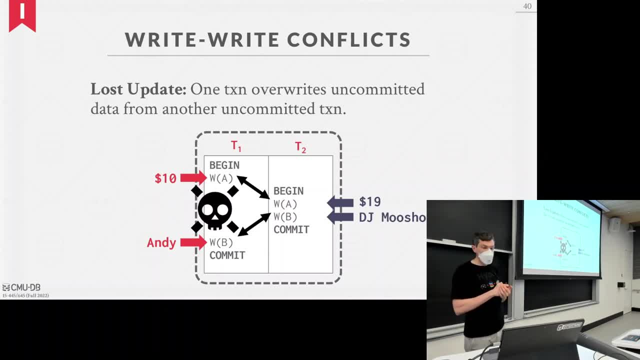 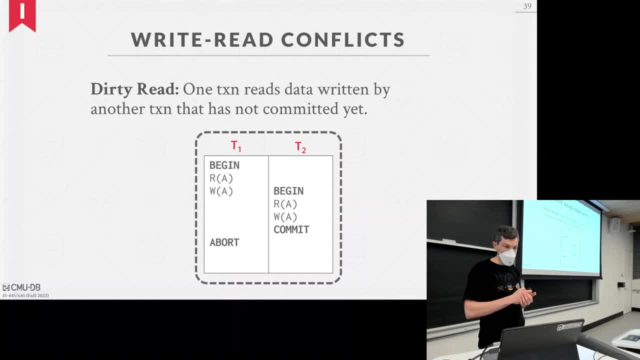 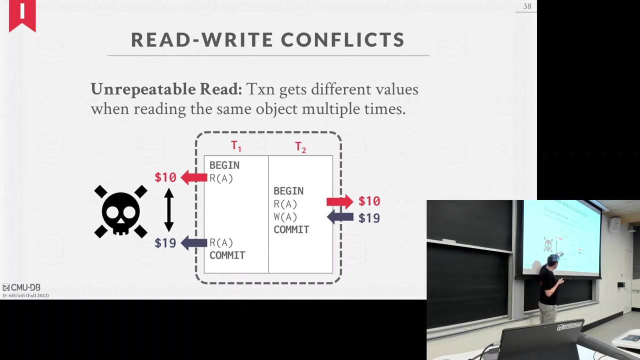 Because it would either be all the changes from T1 or all the changes in T2.. Yes, Yes, Yes, Yes. The question is: is the conflict the first read or the second read? It's the second read, right? I mean, it's a combination of the two of them, right? 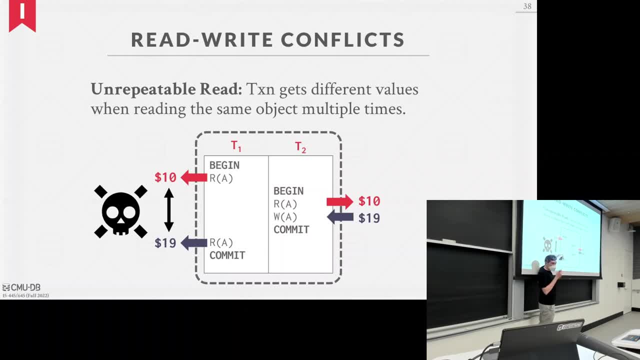 If I see $10 here, then any time I read on A again I should see $10.. Statement is: if T1 only does one read, there's no problems. Yes, Assuming that, say I read on A, Read on A here and I don't do anything else and I commit, there's not a conflict. 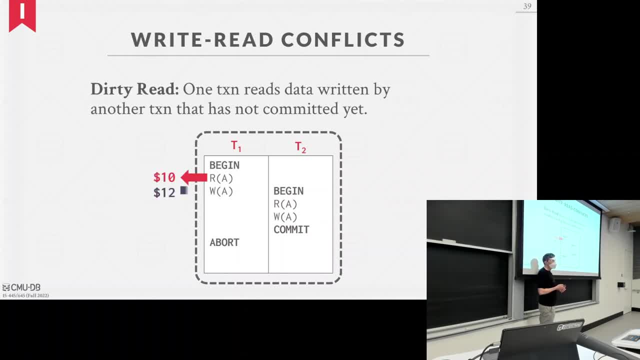 Yeah, Yes, Yes. So instead of abort I do commit here. Is that still OK? That would be OK in this example here. Well, so, Yeah, yeah, Sorry, sorry. So if this guy commits, then, since it didn't update anything else, technically the state. 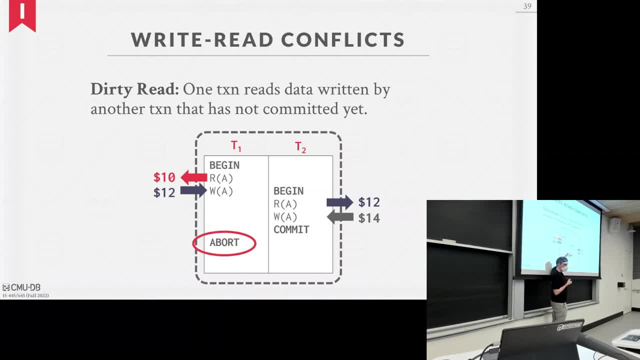 of the database is correct, because this guy overwrote anything. this guy wrote anyway, So it would be T1 followed by T2.. That would still be correct. No, I mean, I was thinking about why you would commit T1, but it just overrides a copy of 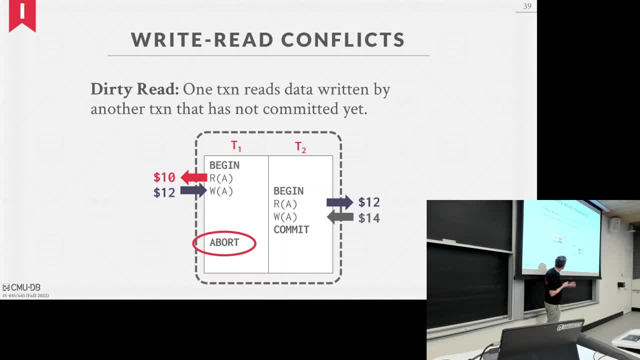 the database, and then you end up with A, B, C, D and so on and so forth. So his statement is, say this is getting queued up, and then you commit and then you overwrite it. In this case, here it would overwrite that. 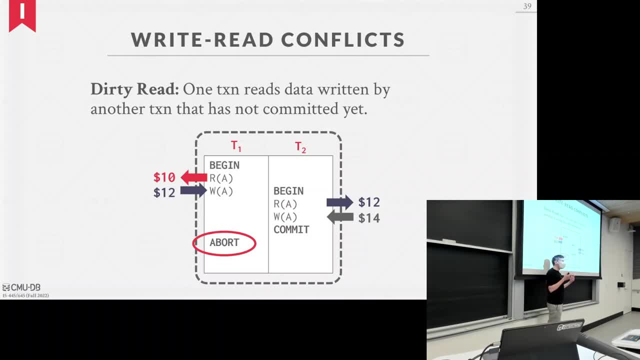 We'll get this in a second. This would be equivalent to view sterilizable where, at the end of the day, the state of the database for A is correct because it is whatever the last one that committed is. But if it was truly running in isolation, like in serial mode, this guy should not be. 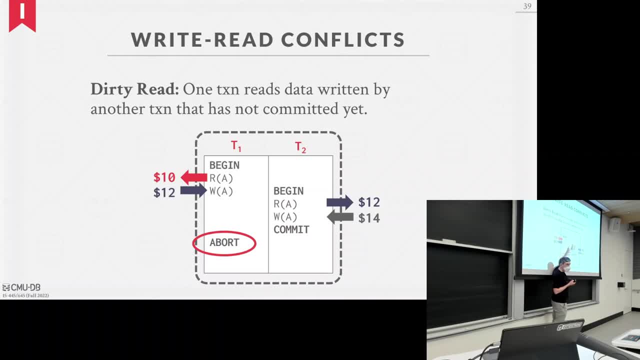 able to see that update anyway. So that's the violation that we want to prevent. There's a high-level- this sounds kind of fuzzy. there's a high-level concept of doesn't matter. That's very hard for us to enforce, so we can't. 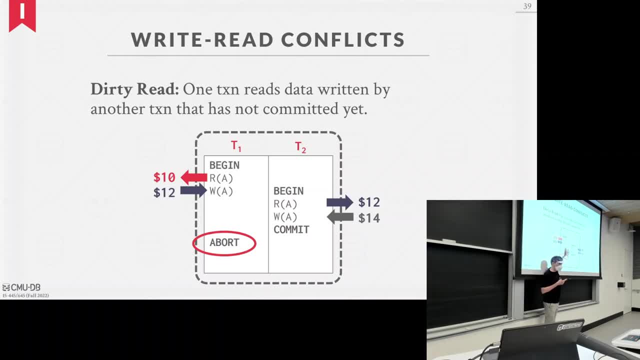 So we'll be very pessimistic- I don't want to use that word- Very strict and say again: don't use that word either. That means something else We want to be. we want to enforce that. you can't see rights from other people. 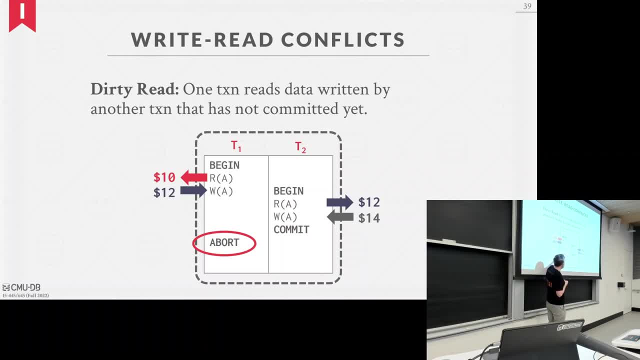 If T1 commits instead of aborting, what would the value of A be? It depends on the implementation of the kernel control. If it's because you could like, yeah, sorry, let me think about this. It depends on the implementation. 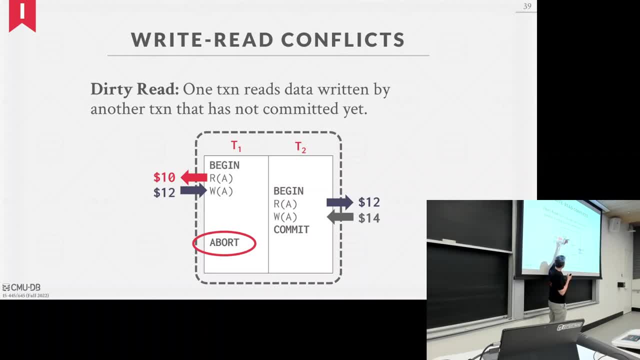 Because it could be the case that, like this thing runs in like temporary mode, not temporary mode, this is running like its own private workspace and then when it goes to commit, then it applies the changes. and so if this guy's already committed, then 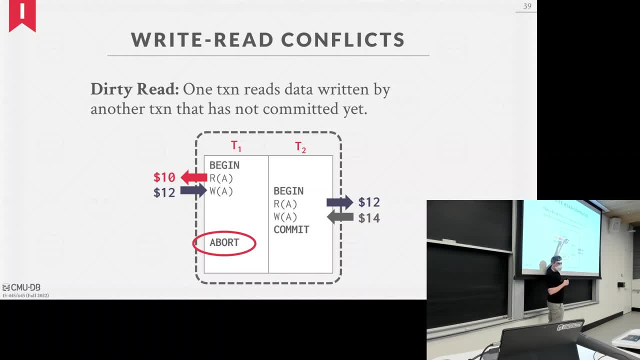 he's overriding that, even though in wall clock time he wrote first, but he wrote in a private workspace that nobody ever saw. This is why I love transactions, because it's like this concept of like, there's like. 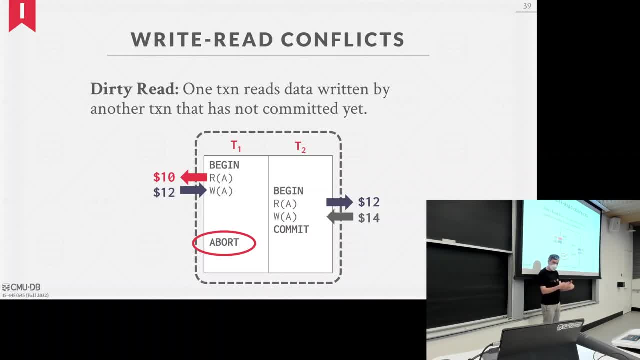 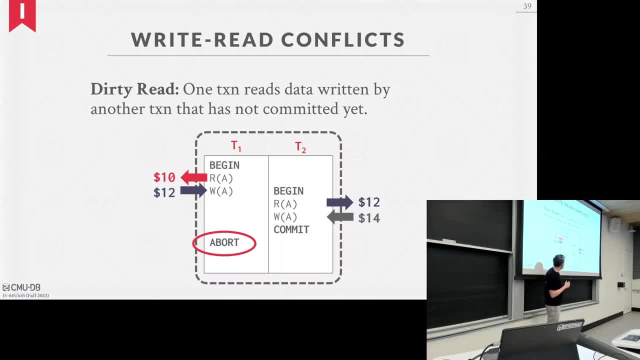 Yeah, Yeah, Yeah Yeah. If the final value is 12, it's not correct, right, In this case here: if the final value is 12, it is not correct. Or, in this case, yes, because this should have rolled back. 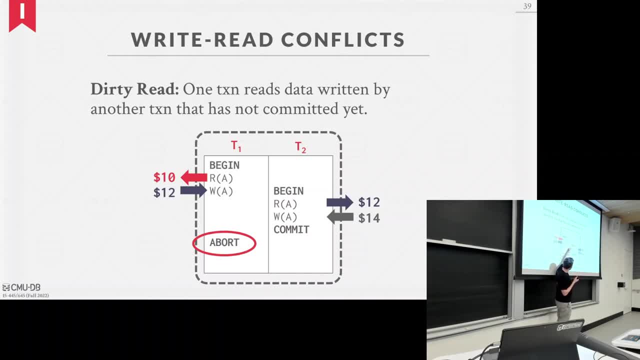 But again, think of like, think of why you don't want to allow this. because, say, I read A and then I don't know what to actually do with that A right, Maybe there's an if-then-else statement. 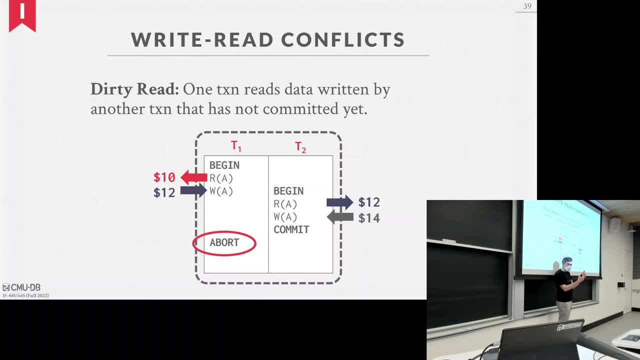 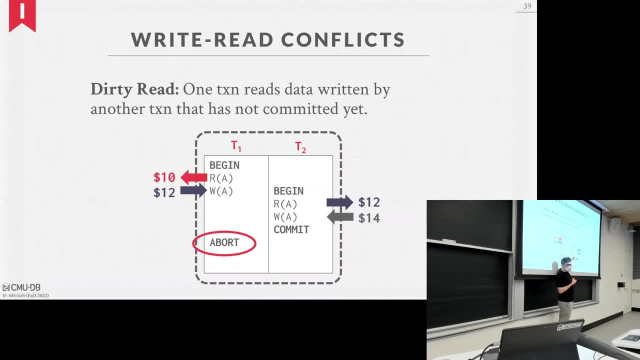 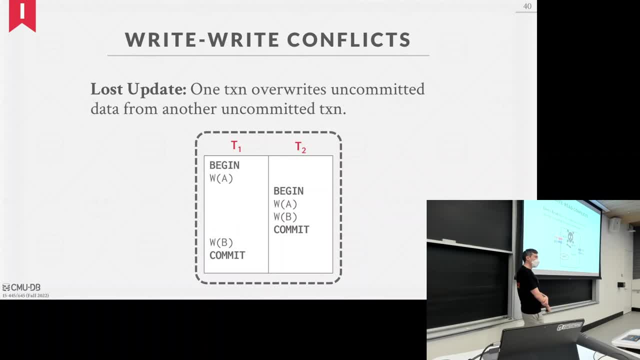 In the back. yes, The question is so in this case, here we have right-right conflict on right-B and right-B here T. If T2 is already committed, why is this then a problem? Yes, because the non-flexing may not be the same as the override, the un-flexing. 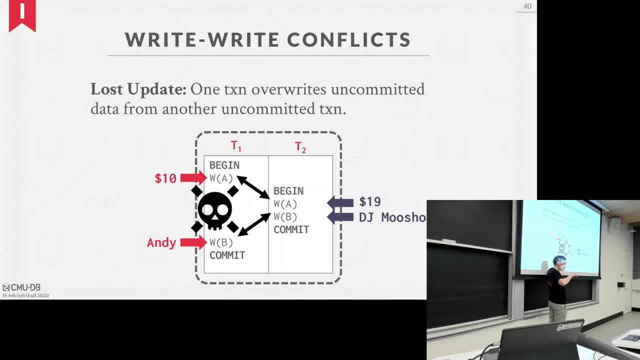 So again it has to be equivalent to a serial ordering. So it's either going to be all the values of T1 or all the values from T2.. In this case here, assuming that on commit that I applied the changes, I would see the 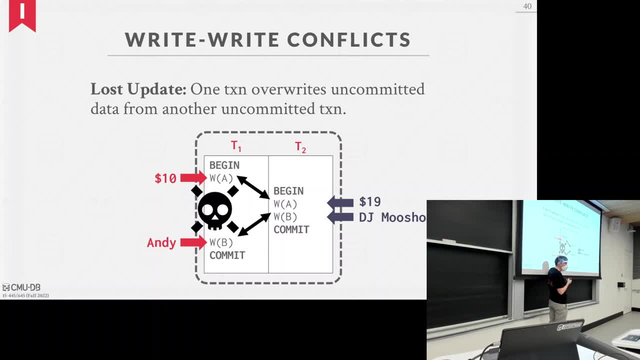 right on A from this guy, but on the right on B from this guy, and that would not have happened if I executed the serial ordering. Yes, So if you're going to be considering the application is okay, because being in a state where either T1 or, in this case I guess, T1, T2, and then T2, T1 could be different. 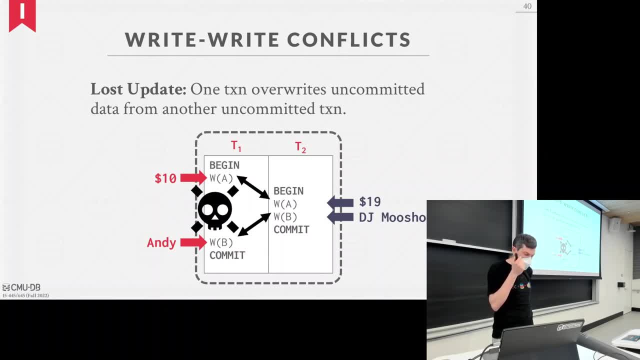 Yes. So the question is- and this is the thing I was trying to say before- the question is: does the application have to be okay with the idea that I can either be T1 followed by T2 or T2 followed by T1?? 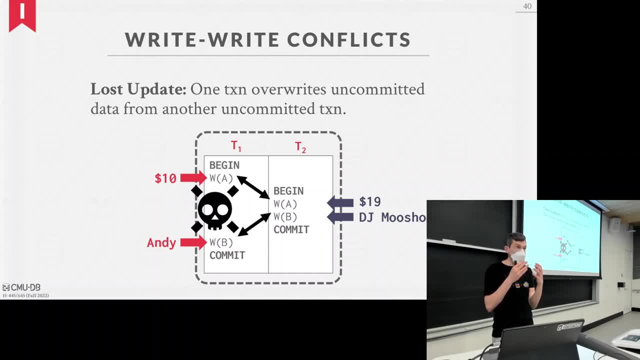 The answer is yes, And that's again. if you cared about the exact ordering- the T1 followed by T2, then you either need to use a database that supports external consistency- which we're not talking about here- or you write in your application your own barrier that says: 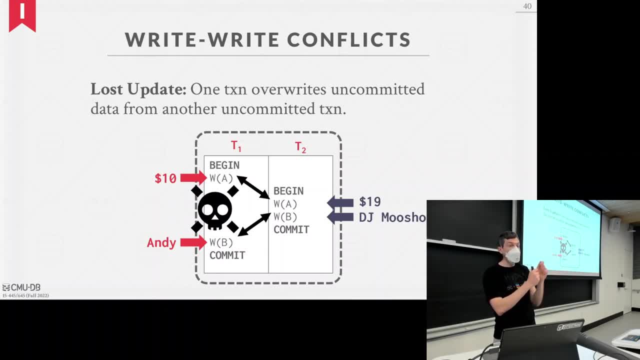 Okay, execute T1.. When I get commit then I execute T2.. Right, Right, Either in the application code or you can do some extra stuff on the server side. but that's hard And it's more work. Most people don't care. 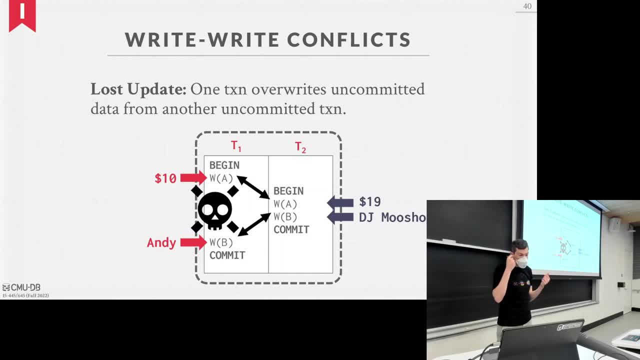 The truth is also too. I would say. I want to get through the serializable stuff because it's important to understand. this is the gold standard of what you would have in a database system, But in actuality, most systems don't actually achieve what we're talking about here. 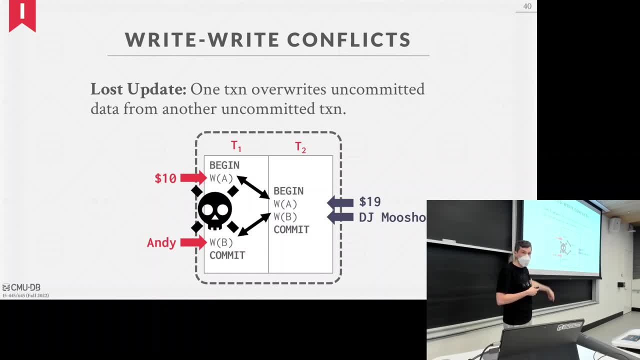 They run at a lower isolation level where you may allow some of these anomalies. Sometimes it's okay, Sometimes it's not. But it's hard because nobody knows. This is actually an open research problem. Nobody knows how bad things actually can get. 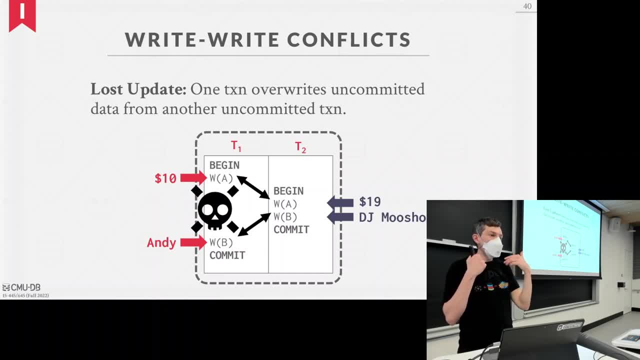 Because if you're actually doing a million transactions a second, if one of these anomalies cause a problem, would you actually know? Probably not, But I think it's important to understand what serializable is, and then we can then strengthen it or weaken it. 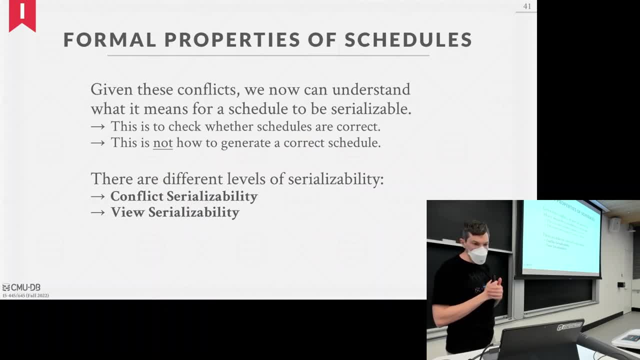 Okay, So this now gets to the comment where I thought she was going about. at the end of the day, in that write-write conflict, or in one of the conflicts, did it actually matter that the write from one transaction overwrote another? 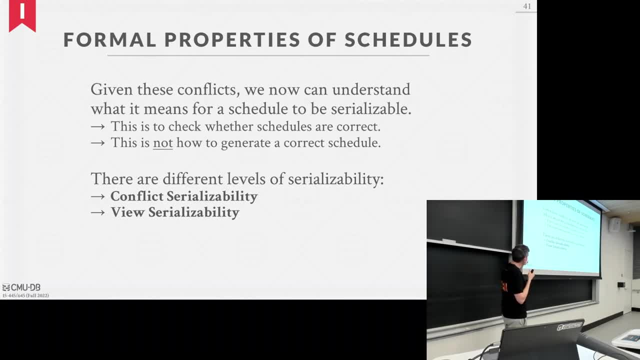 So, yeah, Yeah. So the things we're talking about going forward, these are going to be techniques or a method for us to determine whether a schedule is correct, whether it's equivalent to a serial ordering. Next class will be how we actually generate a serializable schedule at runtime, right? 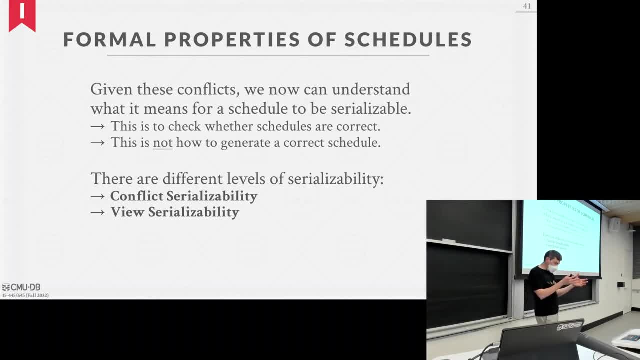 So this is like again from a pencil and paper point of view. we have the transactions ahead of time. We know the operations they want to execute. In a real system you usually don't have that. There's only one system, Fauna- that actually looks at all the transactions ahead of time. 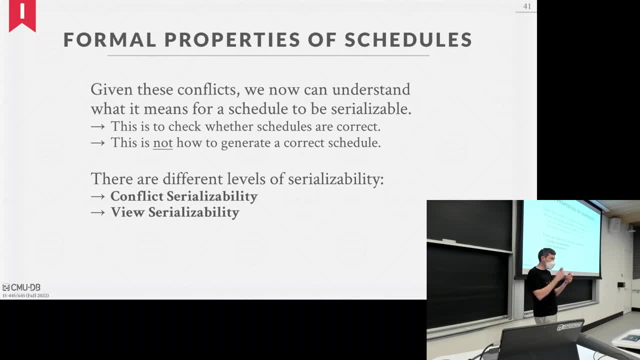 It then does the scheduling of things. Most systems it's where the application is incrementally sending queries, gets back a result, does some additional logic and then sends more queries. So the protocols we'll talk about next week are how to do this on the fly as new queries. 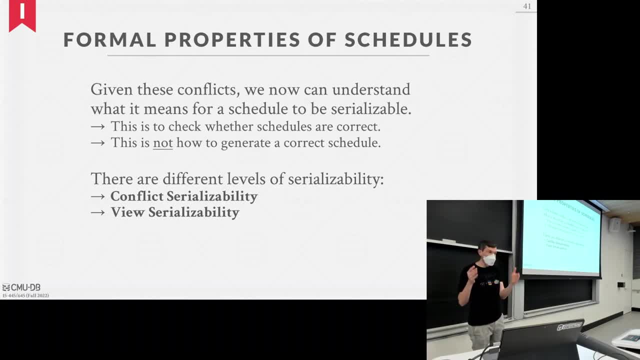 are coming in. Today's class is just about how do I look at a schedule and the operations that the transaction will want to do. I know everything ahead of time and figure out whether it's serializable or not. So there's going to be two different levels of serializability you would care about. 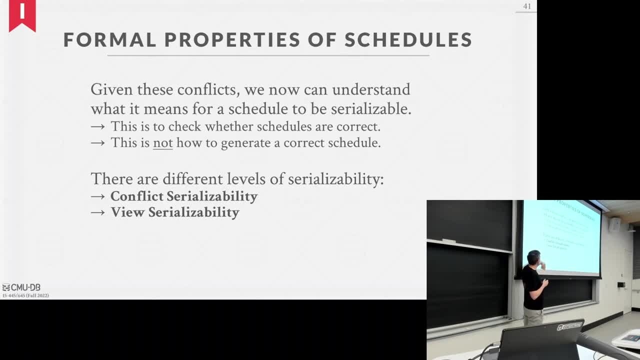 There's actually more, but that's in the theory world. We don't care about that. There's conflict. serializability and view serializability- Most systems, actually all systems. when you say I want serializable, assuming it actually, 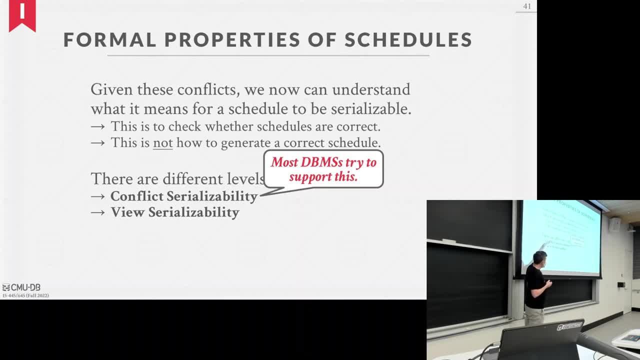 implements it correctly, Oracle doesn't, then you will get this View. serializability is sort of impossible or very difficult to actually achieve because it requires semantic understanding of what the application actually wants to do with the data, And that requires you parsing the data. 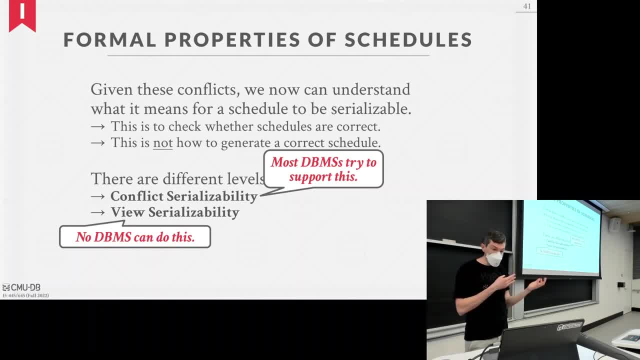 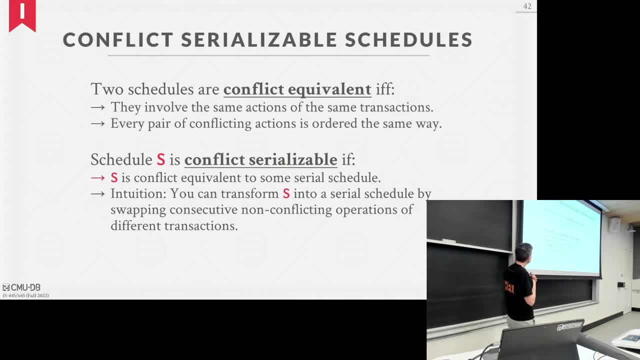 So that's why no system would actually can do this. All right, So what we're going to do now is we're going to say that two schedules are conflict equivalent if they involve the same transactions, the same operations and all the pairs of conflicting. 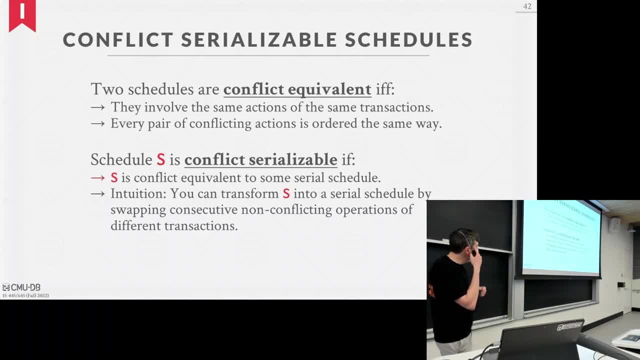 actions will be ordered in some way And then, if we can achieve this, we can achieve, we can determine whether a schedule is going to be conflict serializable if we can guarantee that it's conflict equivalent to some serial schedule. Everyone's eyes are glazing over. 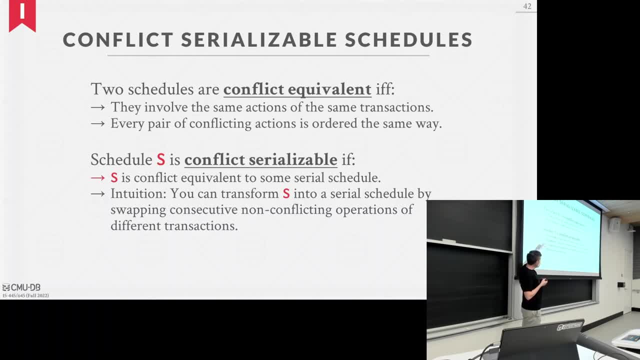 This probably doesn't make any sense right? The basic idea of how we're going to achieve this is that we're going to do this swapping technique, where we can move conflicting operations, sort of swap their order in the schedule so that we sort of push all the operations from one transaction to the top, all the operations. 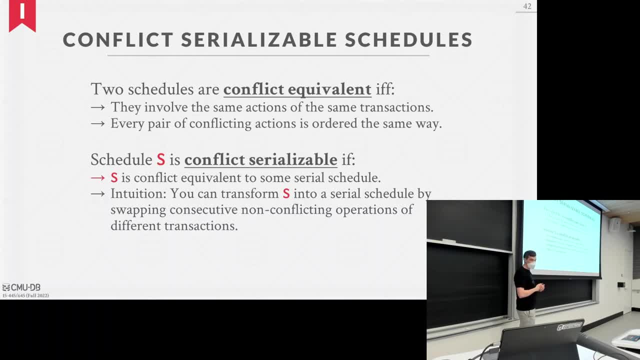 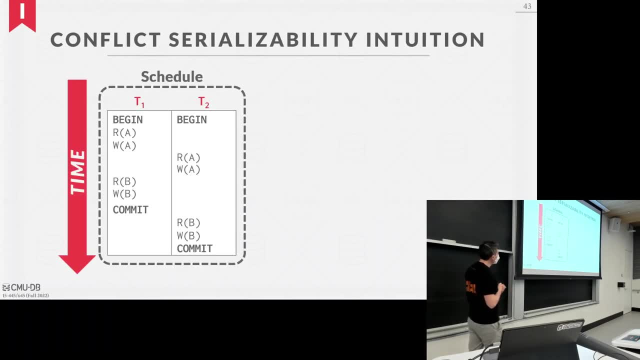 to another transaction to the bottom, and we end up with a serial ordering. And if we guarantee, if we achieve that, then we know we have something that's conflict serializable. All right, So say we have two transactions, T1 wants to. they both want to read on A, write on A, then read on B and write on B. 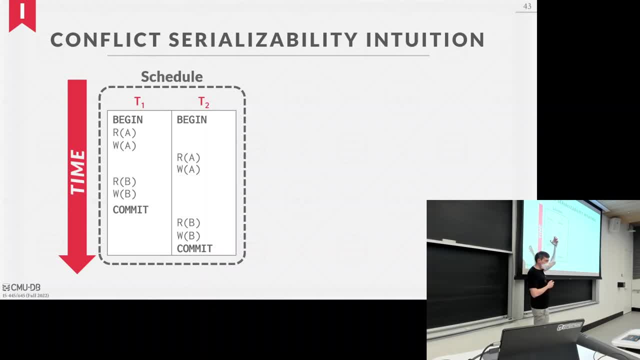 So what we want to do is we want to find conflicting, conflicting operations or, sorry, non-conflicting operations, where we can swap their order and try to push all of T1's operations at the top, push all of T2's operations at the bottom. 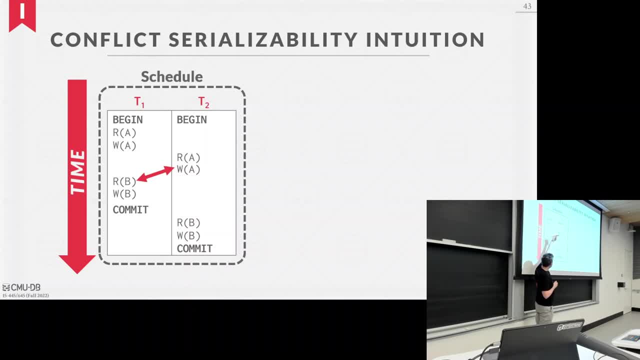 So in this case, here, this wants to do a read on B And that wants to do a write on A. They're not conflicting, so we can swap their order. Now we have a write on B. sorry. a read on A. read on B. read on A. 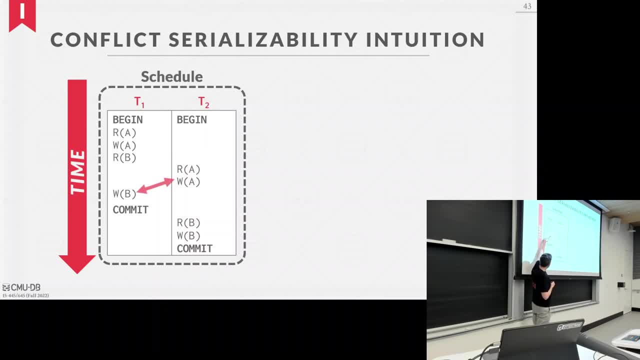 They're not conflicting because they're both reads. Swap their order. Same thing with this: write on B, That's a, write on A. We can swap that. Write on B. read on A. swap that. Yes. Isn't this just killing all of our concurrency then? Again, we're not doing this at runtime, We're just. this is just theory: pencil and paper proving that we can Determine whether this is actually conflict-sterilizable or not. A real system wouldn't actually do this. So your question is like: would this kill a parallelism? 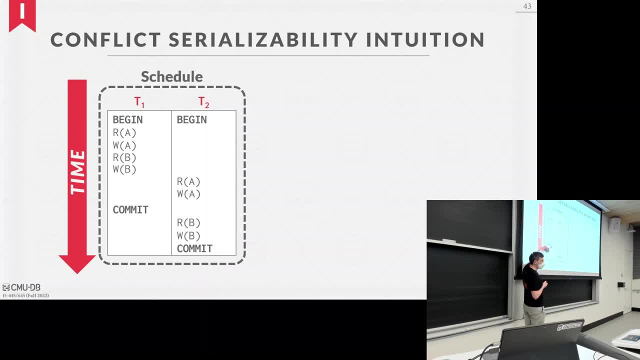 We're not. I'm not saying that I would. I'm not saying I would execute it in this order, because then it's just serial ordering. I'm trying to say, if I start here with my original schedule, this thing here is this: 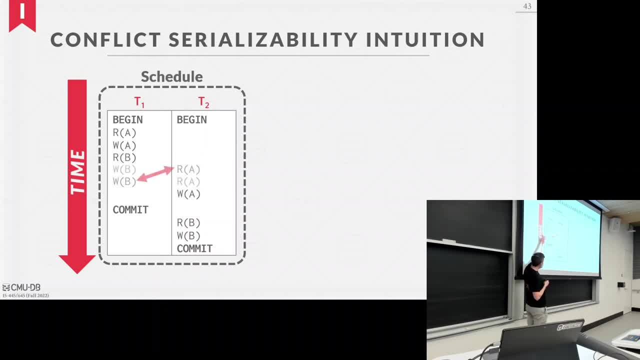 conflict-sterilizable, yes or no? And by swapping and pushing things up and down you can determine that it is equivalent to a serial ordering. What's the criteria for this To make it commit? I'm I'm sorry. I think what I was just trying to do is say, like, by the time, this: 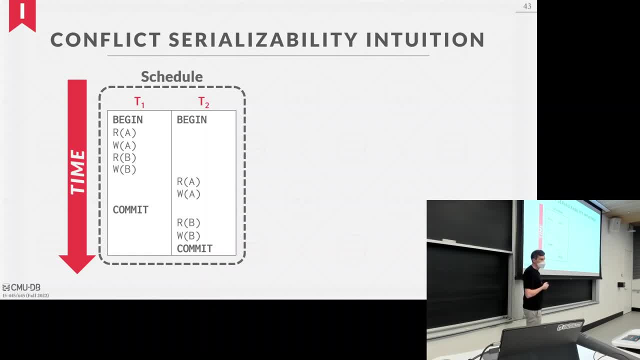 commits. I can ignore everything below that. Yes, So then, with the convert I'm trying to maximize concurrency. do you just start with it fully, like this, and then try to take everything from T to push it as far up as you can. 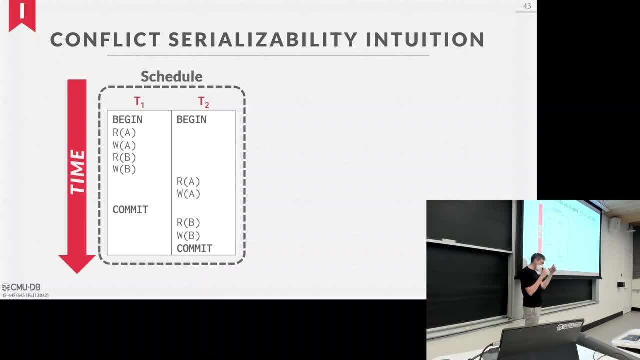 The statement is: if I, If I start with a serial ordering the way to find the most parallel schedule, would I then try to do the reverse of this? Yes, but in a real system you wouldn't do this because you wouldn't know, like you. 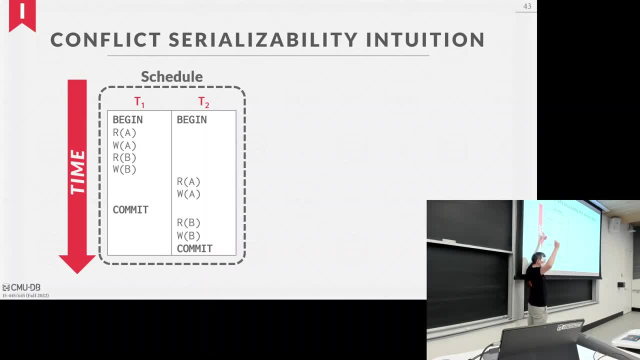 would see like the application would call begin and maybe you see the first read, but you wouldn't know what comes after that, And by the time you get to the bottom here you've already executed the other ones. Two-phase locking will fix this for us on Tuesday next week. 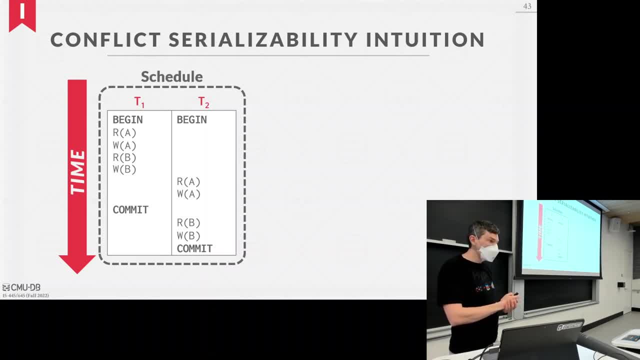 That seems to active transaction right. Some databases don't support active transaction. You have to send the entire transaction from beginning to end to the database. So the statement is: some systems require you to send all the transactions from beginning to end to the database ahead of time. 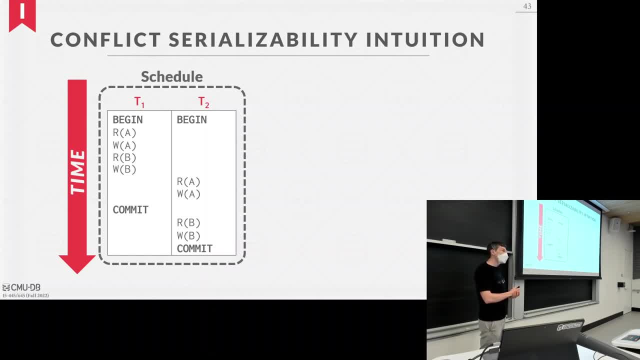 Yeah, so DynamoDB does that, Fauna does that, They, Yeah. so in that case, yeah, they're. basically they wouldn't use this algorithm because this is obviously inefficient but, like you, would figure out the interleaving within a batch. 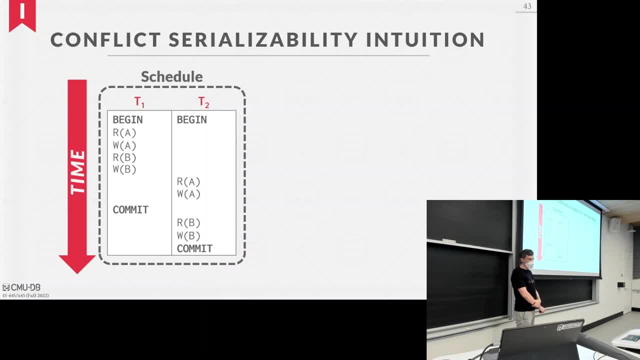 and then submit them all at once. Most systems don't do that. Most applications aren't written that way. Yes, What if, instead of T1 committing at the end, it aborts? Would you still consider this appropriate to serialize it more? 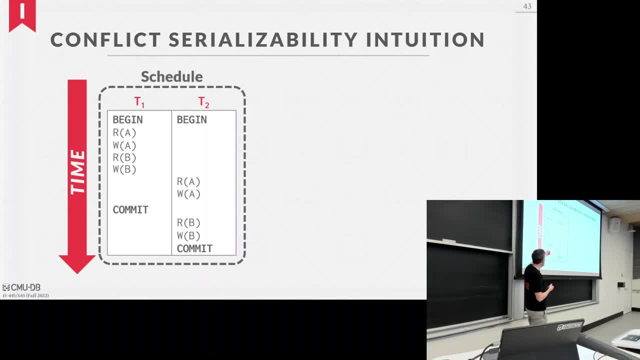 So his question is: instead of T1 committing it aborts, Would this still be considered serializable? Going back here, We can ignore aborts. for this It depends. It depends on how it's implemented. right Like this is just getting just pencil and paper. 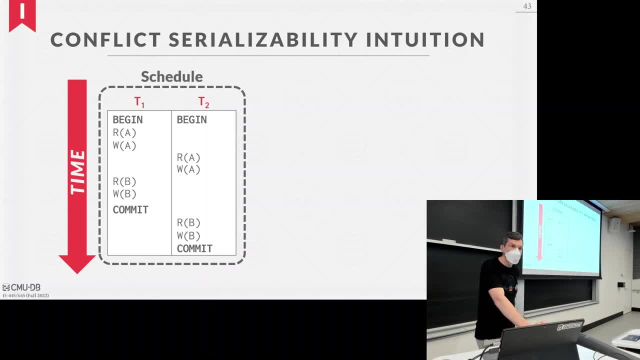 Yes, Are we assuming here that whatever like A is in T1, T should be available to T2?? Again, that's the implementation detail. We can ignore that for now. All right, so this is equivalent to this. Here's one that isn't right. 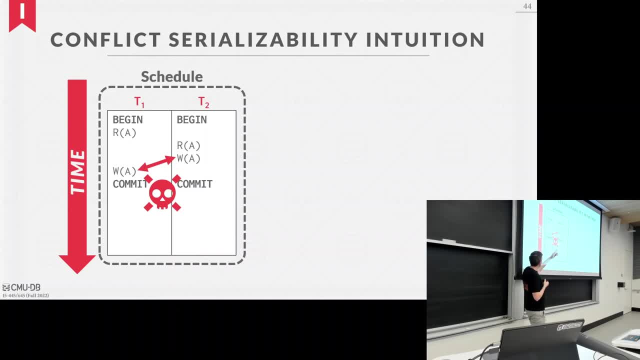 If we try to swap the write on A, the write on A, here we cannot swap with this right Because they're both writes. so therefore this is not equivalent to a serial order right. So this swapping thing it'll work. 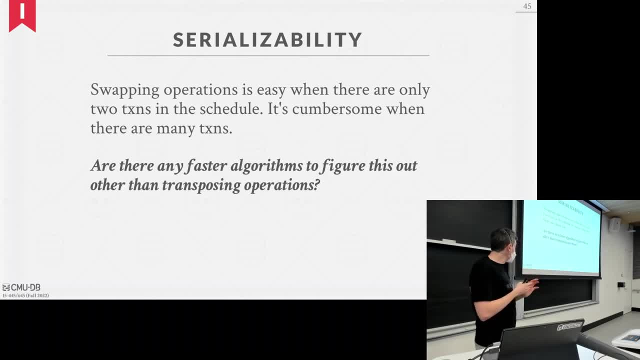 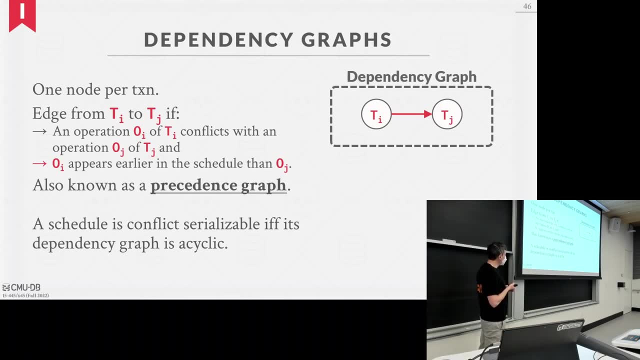 It's easy to do for two transactions, but it's cumbersome to do when there's many transactions, And so a faster way approach to do this is to use what is called a dependency graph. I think Wikipedia might call this a dependency- sorry, precedence- graph. 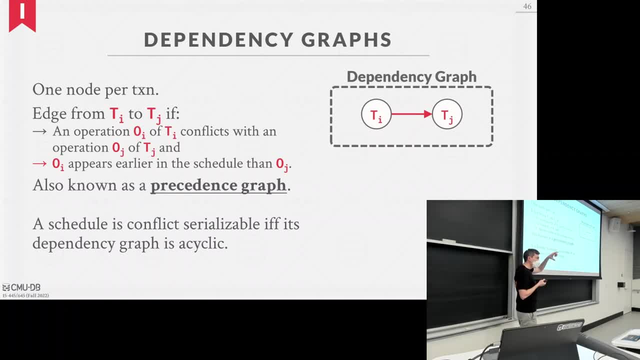 The basic idea in our graph is that we're going to have one node per transaction. that's in our schedule- And then we'll have an edge from transaction T1 to transaction TJ If there's an operation in the first transaction that conflicts with another operation in the other transaction. 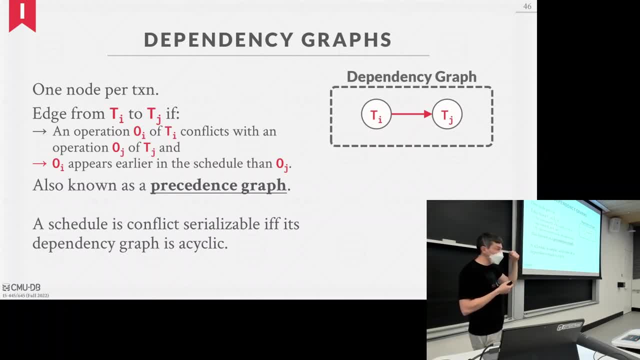 and that first operation in the first transaction appears earlier in the schedule than the operation in the other transaction, you would have a directed edge from TI to TJ, And so we would look at the entire schedule, build out this dependency graph and if there's no cycle, 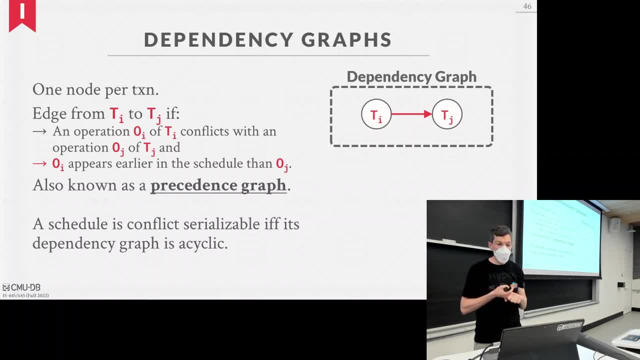 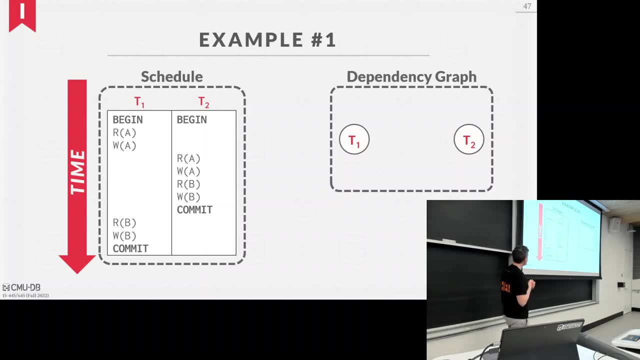 in the graph, then we know that the schedule is conflict-sterilizable. All right, so we're going back to our example here. So write on A, read on A, write on A and read on B, and write on B. 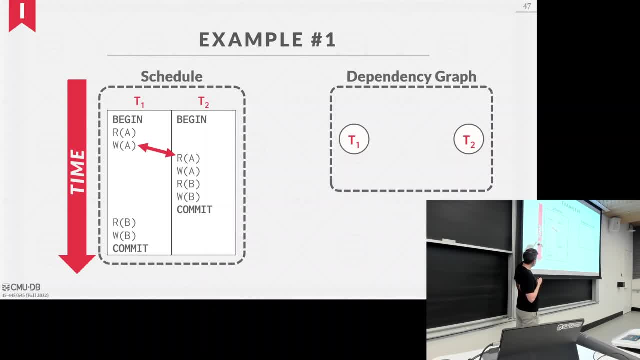 In this case, here we have a conflict between write A and read A, So we have an edge from T1 to T2.. Then if here we have a conflict on write B to read B, so we would have an edge from T2 back to T1.. 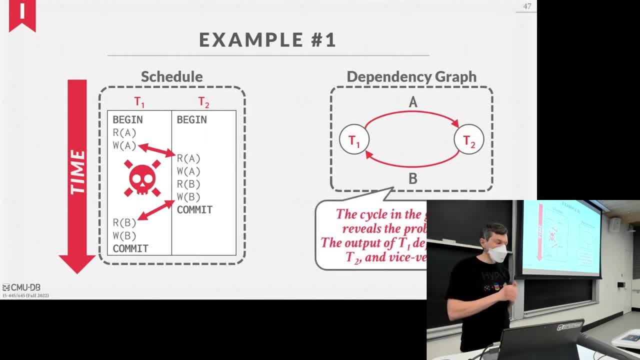 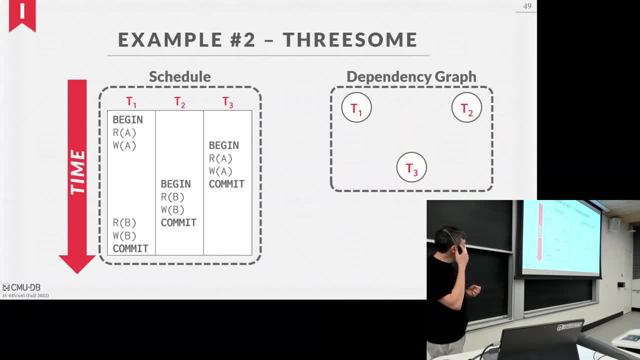 We have a cycle. Therefore, this is- This is not conflict-sterilizable right. Let's look at a more complicated example here. Now we have three transactions, So we're going to do a read on A in T1,. 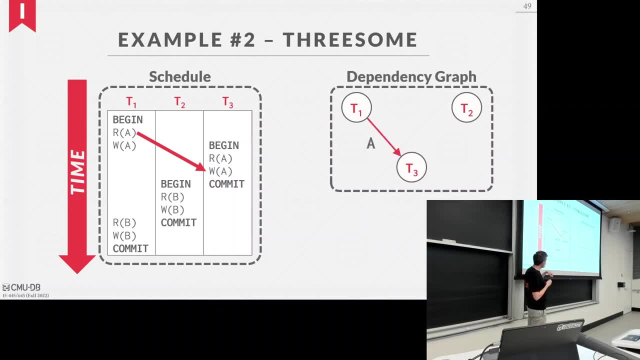 and that'll conflict with the write on A in T3.. So we have an edge from T1 to T3.. We have another write on A to a read on A in T3, but since we already have an edge from T1 to T3 in our dependency graph, 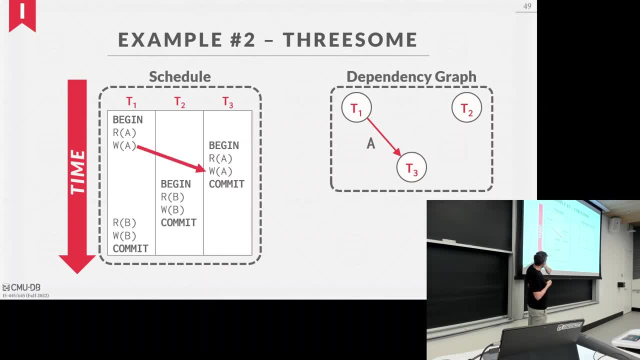 we don't need to draw it again. Same thing with the write-write conflict here. So we don't need to draw that again. And then on this side here, the only conflict we would have is the write on B to read on B. 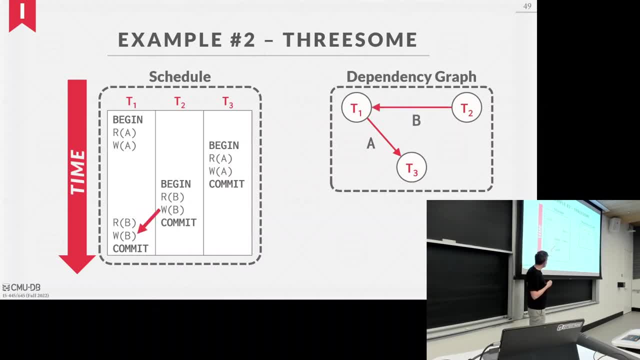 We'd have an edge from T2 to T1, and then write B and T2 and write to B on T1.. Again, we already have an edge there. so it is We don't draw an additional edge Right. so is this equivalent to a serial execution? 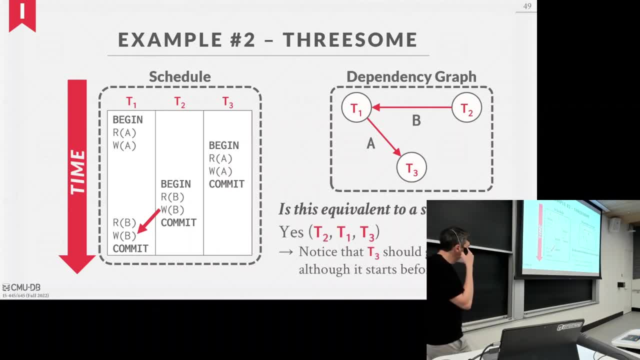 Well, by definition, yes, because since there's no cycle in the graph, it is, And it would be, T2, followed by T1, followed by T3.. Right again, this idea that we can reorder the commit ordering of transactions to be different than their arrival order. 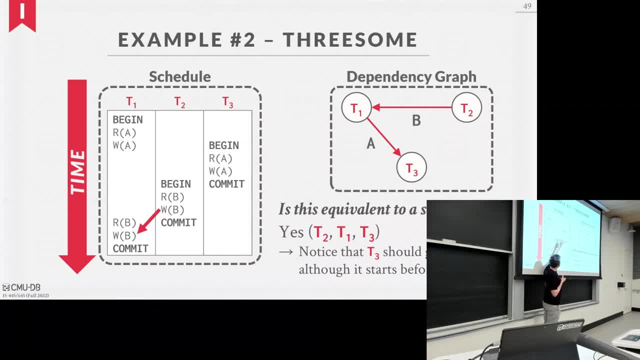 In this case here T3 called begin before T1, assuming this is wall clock time. But in our serial order we're going to say that T3 will get committed after T2, even though it started before it, And that's still okay. 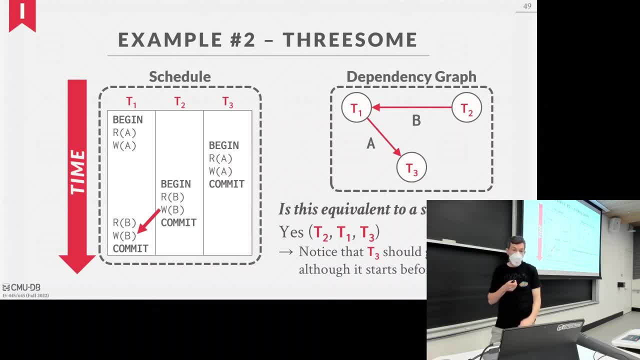 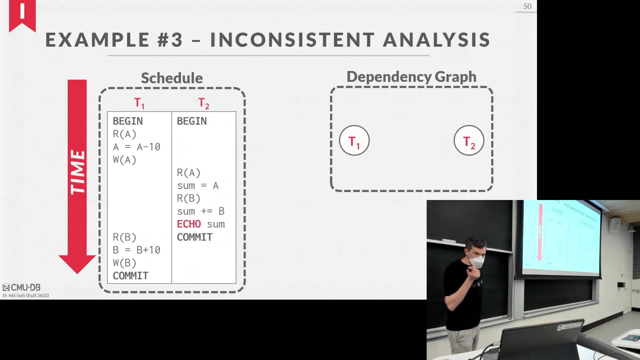 That's still equivalent to a serial ordering. Yes, The state of the database will be equivalent to where T3 committed after T2.. And that's okay, All right. so in the sake of time, I'm going to skip view sterilizability. 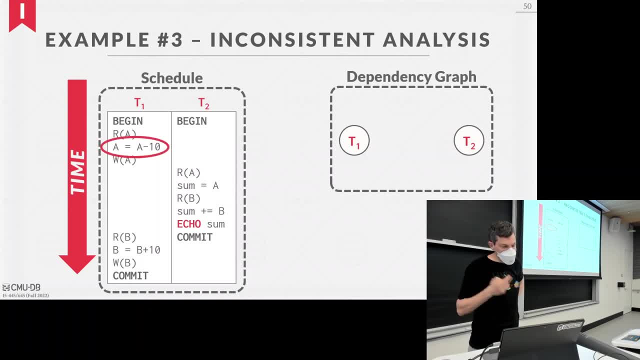 Again, no application, actually No database is actually supported. No database is actually supported. I just quickly want to show you. the basic idea here is that if I try to compute something like I add to, I want to read A, read B and then add them together and print it out. 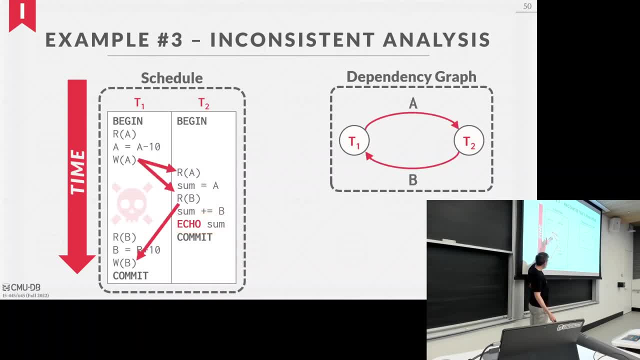 If I do my dependency graph stuff, then I will have cycles And this will say that this is not conflict sterilizable. But if I just change the code, where I don't actually care about the sum, the exact value. all I want to know is the number of accounts that have a. 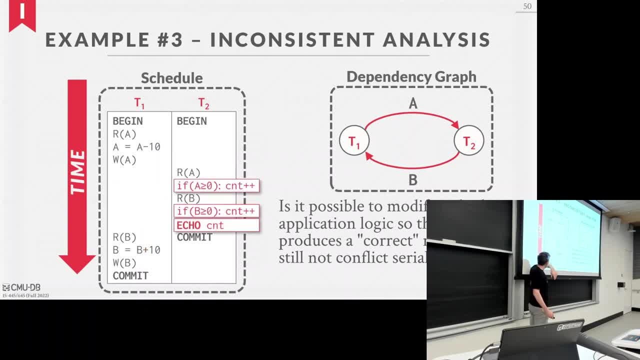 that have more than zero dollars in their bank account. So if I just rewrite the application to this, then, assuming that these values are above zero, then I can produce actually the correct result. But again, this is hard. How would the application know that this is actually what you're trying to do? 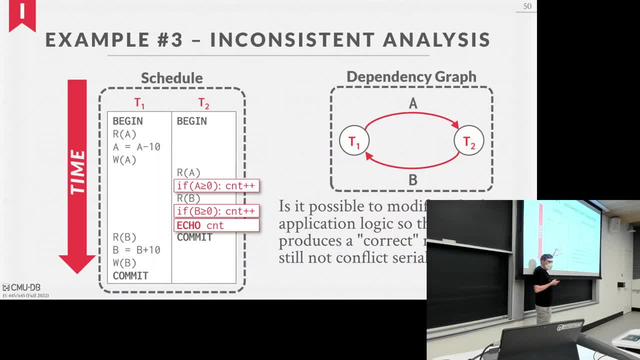 and that this count doesn't really matter. I mean, you can do maybe deeper static analysis and understand what's going on, but now you've got to support every possible programming language that someone writes an application in right, And that'd be super hard. 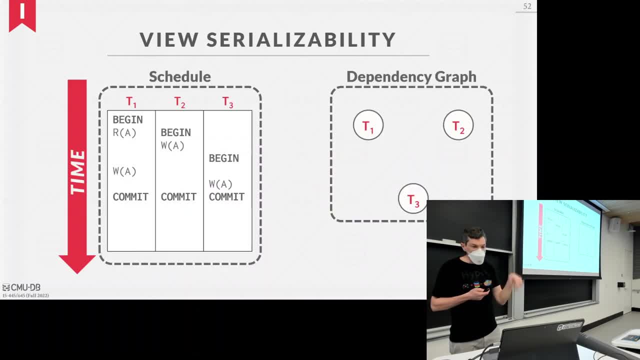 So this is what view sterilizable means, right? Or the other example that I think someone brought up before: like if I do a blind write, like if I T2 writes A and T3 writes A without actually ever reading it, then even though there's a cycle in my dependency graph, 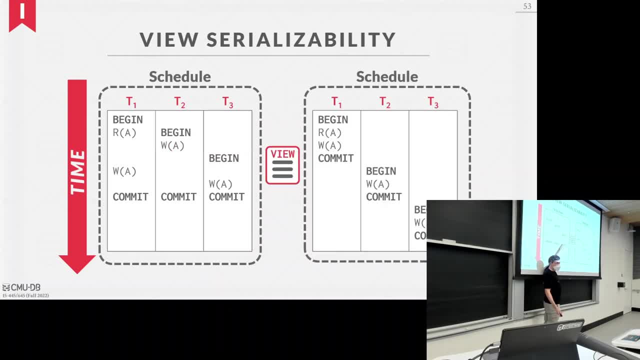 at the end of the day, all I care about is that this guy wrote it last, And that's okay. So the main thing I'm just pointing out is there's a looser notion of sterilizability that you can get through view sterilizability. 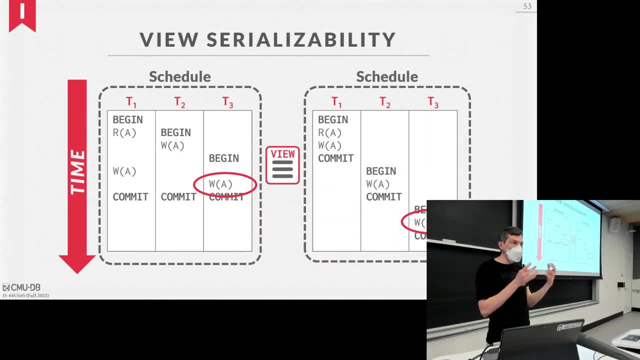 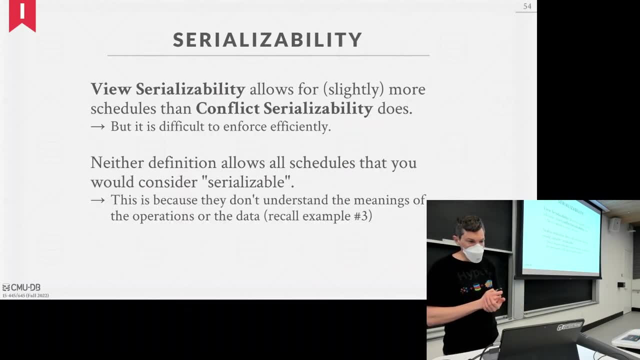 but it requires you to understand: are certain things okay in the application? Is the program actually going to care? And that's really hard to do, So nobody does it. Okay, Right, so pretty much, if you answer sterilizability, this is what you get. 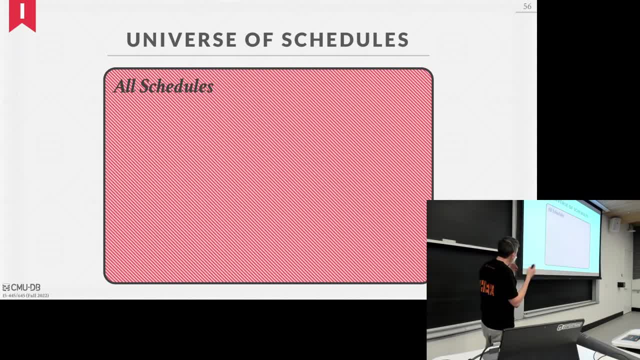 So the way to think about what possible schedules could exist is through this. There's sort of this nested structure here. So say that this region here is all possible schedules. No notion of correctness, no notion of serial ordering or sterilizable. It's anything you possibly could do, right. 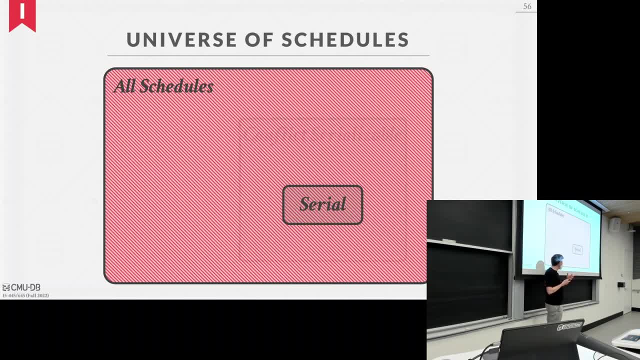 And then in the middle is going to be serial ordering- Oh sorry. And then after that would be conflict sterilizable and then after that would be view sterilizable. So any schedule that is serial is also conflict sterilizable and view sterilizable. 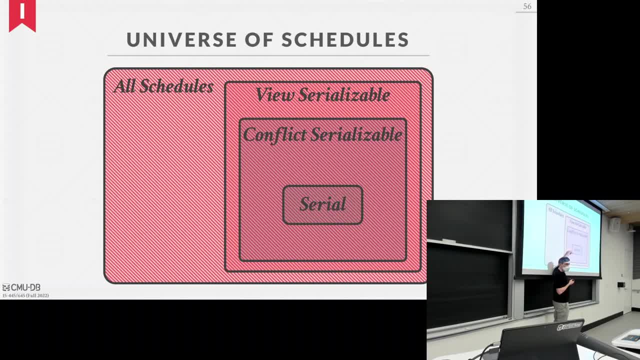 but not every view. sterilizable schedule or conflict sterilizable schedule is serial Right. so most systems again are going to be hanging out in this middle part here, because it's efficient to execute it, You can efficiently implement it, You can efficiently guarantee that there's property. 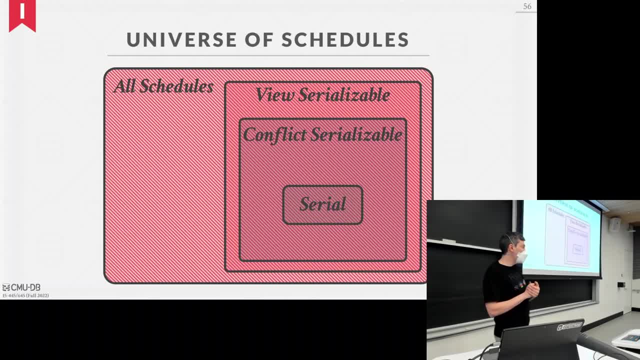 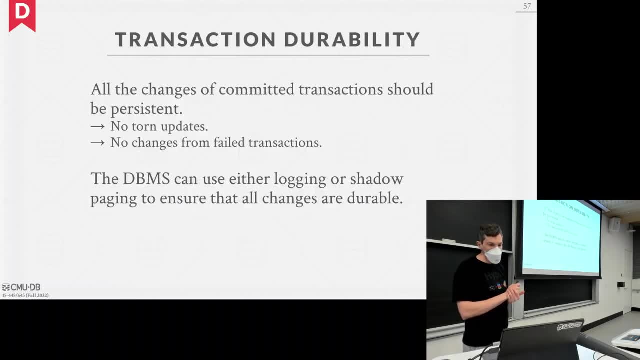 And there's enough opportunities for parallelism that you can get better performance than you would in otherwise in serial ordering. All right, so quickly I won't say much about transaction durability. We've already talked about a bunch of things: The logging and the shadow paging. 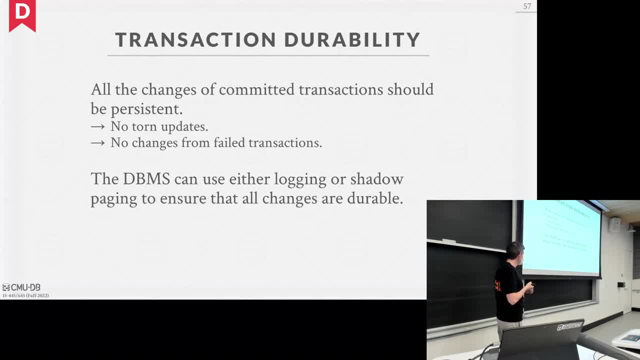 We'll go into more details how this all works in two weeks. I realize I keep saying we'll cover this in the future, but there's a lot to cover here and I can't sort of. You guys can ask your questions about. 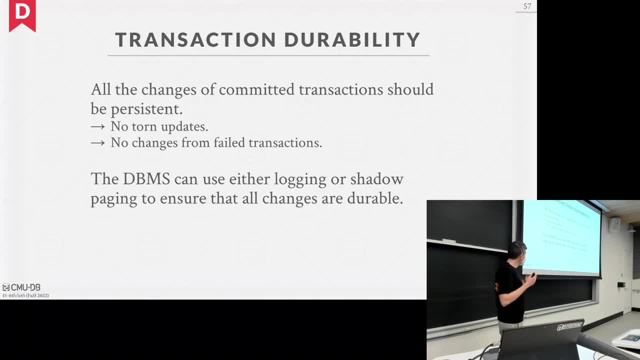 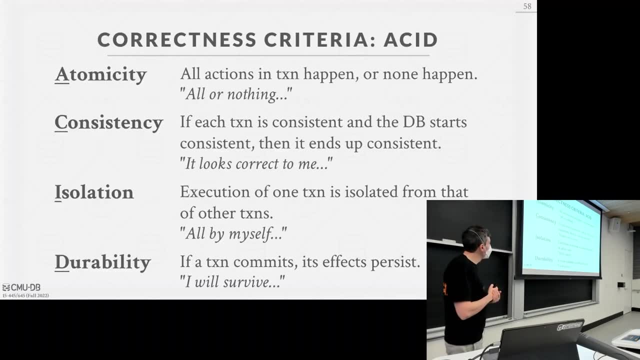 hey, what about this? And there's answers to those things that are in the future lectures. So I just want to say we will cover this in the future, All right. and then we've discussed all the asset stuff before. So In my opinion, the concurrency troll. and the recovery mechanisms in a data system are some of the most important features, along with the query optimizer. This is really hard to do and get correct and make sure you don't lose data. don't have transactions do things they shouldn't be doing. You want transactions. It makes it easier for the programmer to write code and not worry about weird issues. There's always some. I think it was a Bitcoin exchange that went down recently because some guy bled them all the money because they weren't doing transactions correctly. 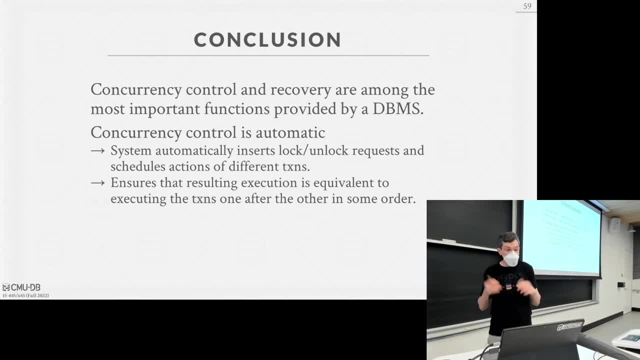 So you want a data system that does transactions. You don't have to worry about these anomalies, because the data system will guarantee it for you, And so we'll see, next class, how we're going to use concurrency troll to automatically guarantee that we can take any arbitrary set of queries. 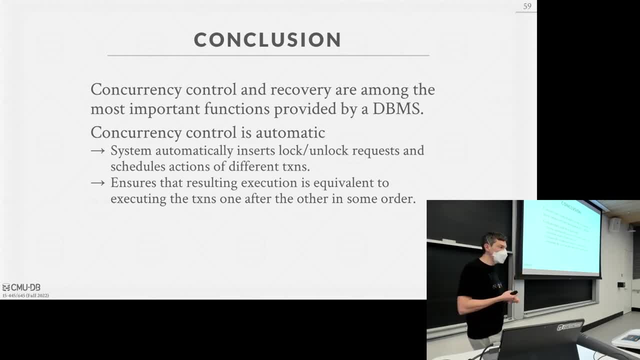 that are showing up from our application and still guarantee that we achieve serializability. And then we'll talk about weaker isolation levels, where we can start relaxing some of these guarantees and allow some anomalies to occur, Because that's going to potentially give us better performance. 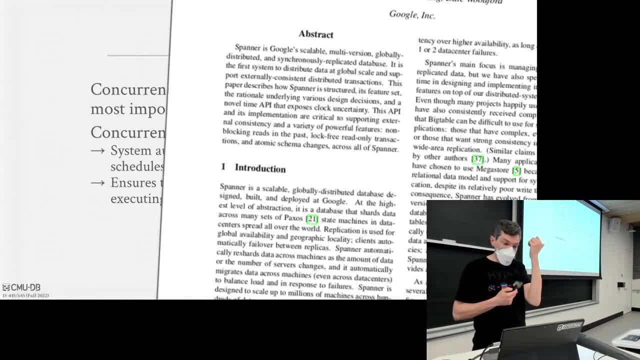 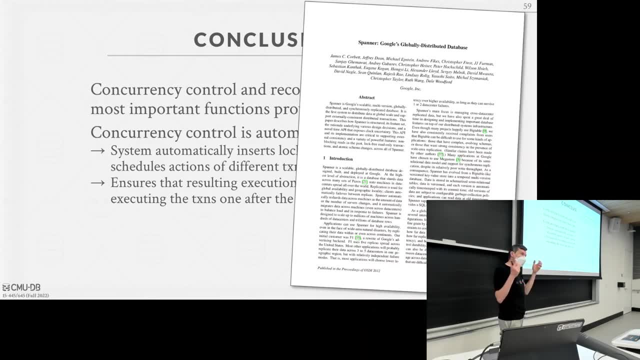 So don't take my opinion that I think transactions are super important. There's this paper from Google about Spanner. over 10 years ago in OCI, Google was at sort of the forefront, or they were sort of the vanguard, of the NoSQL movement. 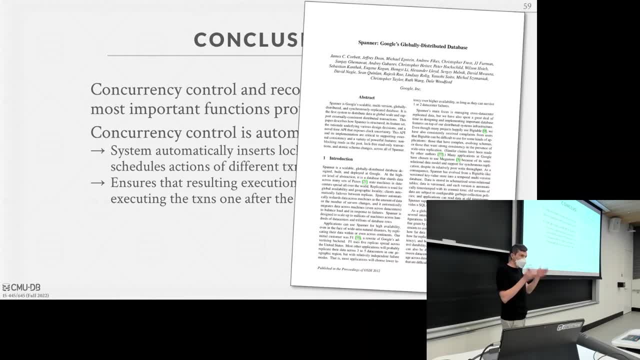 because they built all these systems that didn't do transactions, because they cared about performance and scalability, And everybody copied them because Google was making a lot of money. They're smart, let's do what they did. And then Google realized: oh for transactions actually. 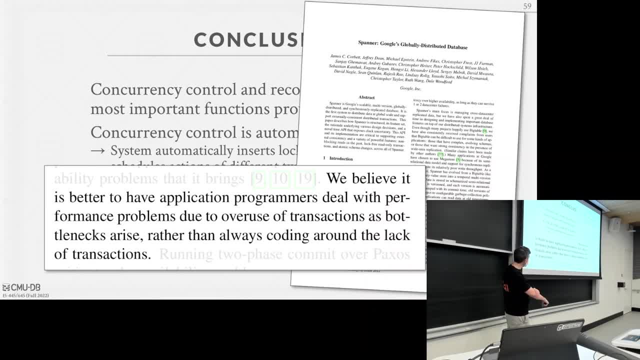 a good idea. So there's this line in the paper that says we believe it is better to have application programmers deal with performance problems due to overused transactions as bottlenecks arise, rather than coding around the lack of transactions, Because the lack of transactions is the comment I said before. 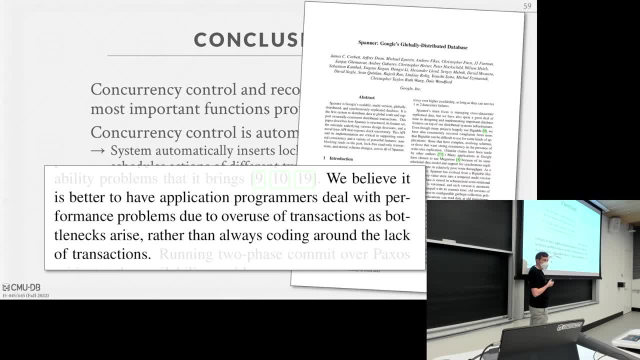 in these NoSQL systems where you have to write your own application code to deal with all those anomalies that I talked about. So if you don't, the average programmer is probably not gonna be able to reason about these things. Let the data system do it for you. 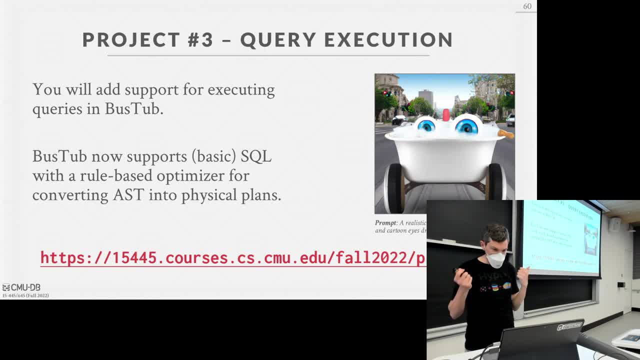 Okay, I want to quickly talk about project three. So project three is out. You're gonna be implementing query execution support in Busstub. Busstub now supports basic SQL And we have a rule-based optimizer that can take a SQL query, convert it to an AST. 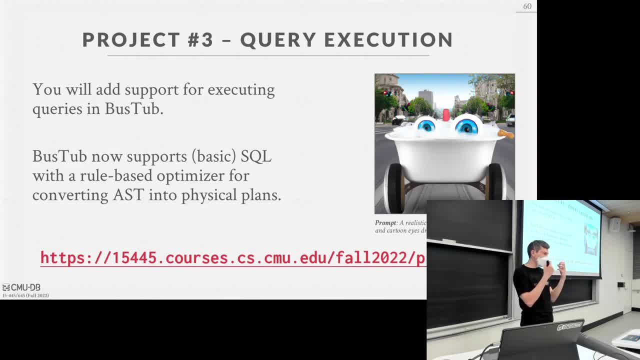 and then convert that AST into a physical plan And then your job is to build the query executors or the operator executors that can execute those query plan nodes, right, So everything is posted on the project website And pull the latest version from GitHub. 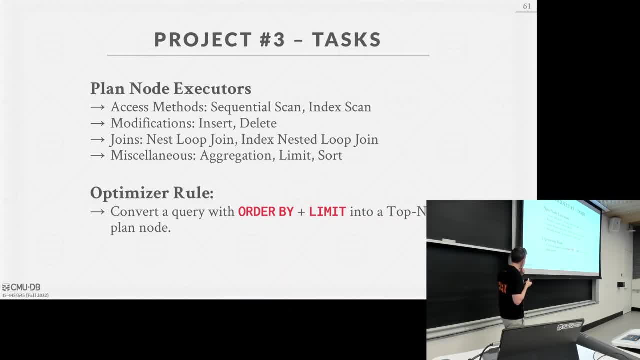 So there's two major tasks. Most of the work we spent on doing plan node executors. So you do sequential scan, index scan. We're only doing inserts and deletes, You don't have to worry about updates. And then you do a basic nested loop: join. 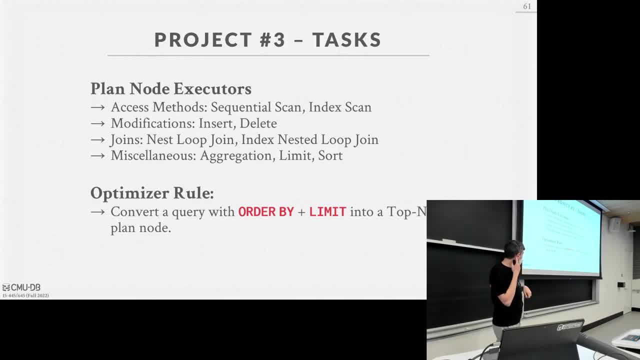 and an index nested loop, join Then aggregations, limits and sorts. So for those that struggled on project two, checkpoint two: when having concurrent index, if you think your thing has bugs, just put a latch on top of the entire data structure. 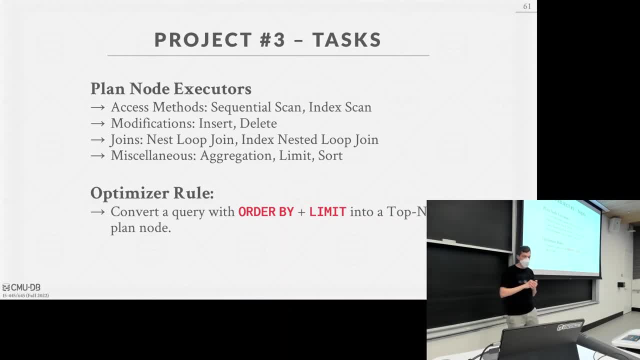 And that'll be okay. for project three, okay, What? Well, we'll do that in a second right, And then we have a rule-based optimizer. There'll be one task at the end: We have to convert the order by and limit clause into a top end right. 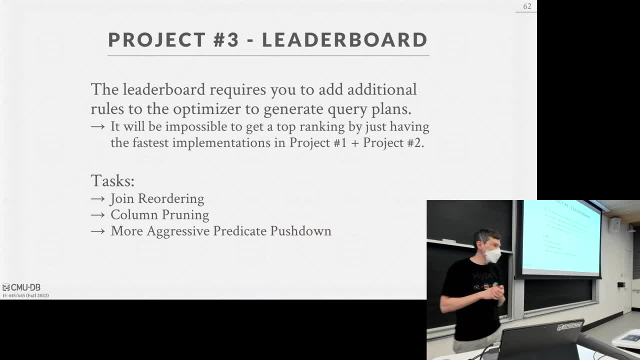 Which is more efficient. So now the question is: will that be efficient? No, But for the leaderboard. what we're going to do, rather than relying you having whoever had the fastest project one and project two, crush it also for project three on the leaderboard. 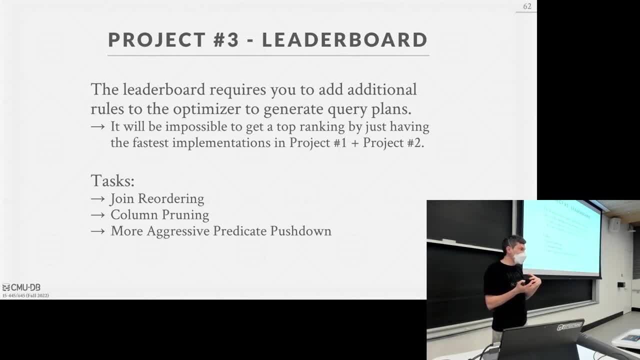 we're actually giving additional tasks now that would not necessarily rely on you having the fastest implementation for your buffer pool manager and your index Right. The basic idea is that you have to implement new optimizer rules to get better query plans, Because for certain queries, the optimizer we have now will produce. 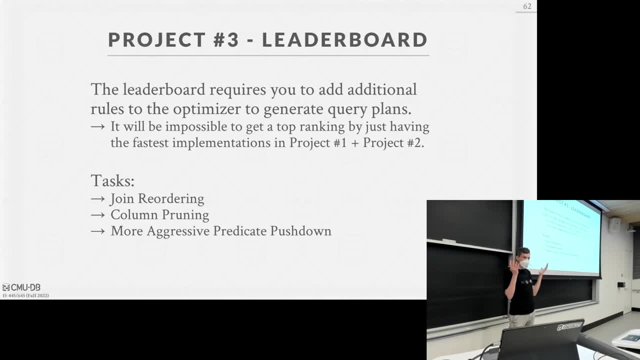 it's horribly inefficient query plans And no matter how fast your B plus three is, you would lose out. So this is the idea here: to make it so that like it's not the same people always getting top ranking for the subsequent projects. 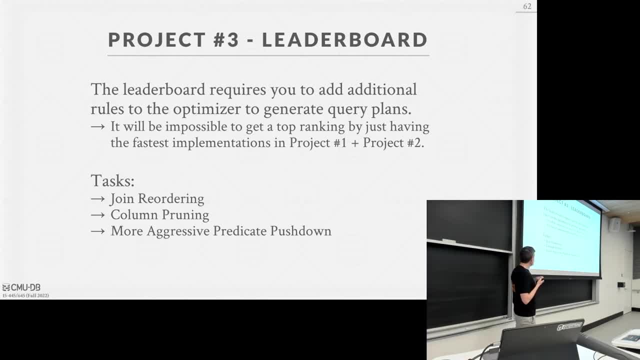 You can actually do some extra stuff and still beat them. So the task you have to do for this, or implement optimizer rules to do joint reordering, column pruning and then a more aggressive predicate: push down, Yes. If I don't do this, will that interfere with project four? 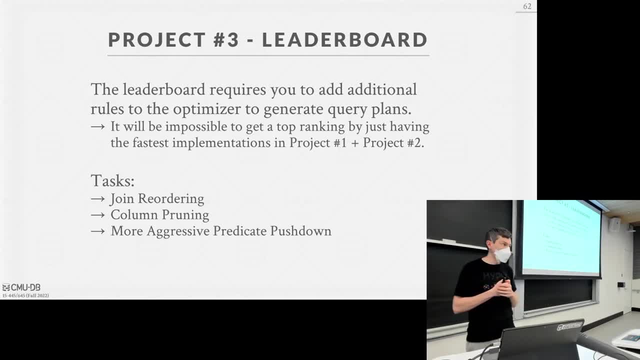 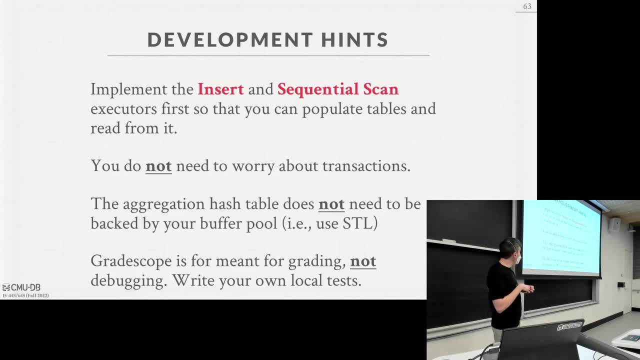 His question is: if I don't do this, will that interfere with project four? No, Yes, This is optional. Yes, All right. So my advice to you guys: start with insert sequential scan. do that first So you can implement, actually read data. 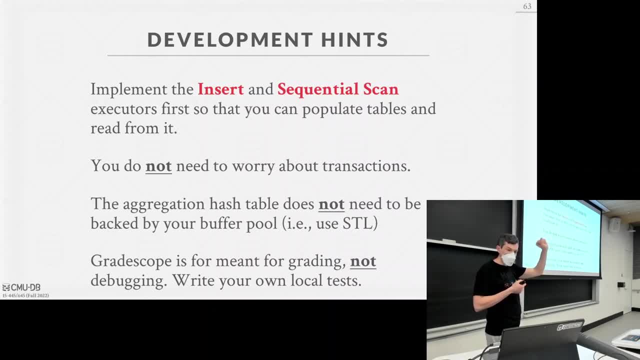 There is a mock table that he has a mock sequential scan. But Chi did this, He's fantastic. So there are internal tables that you can then run queries on and maybe test other parts of your database, like your sort calls and so forth. 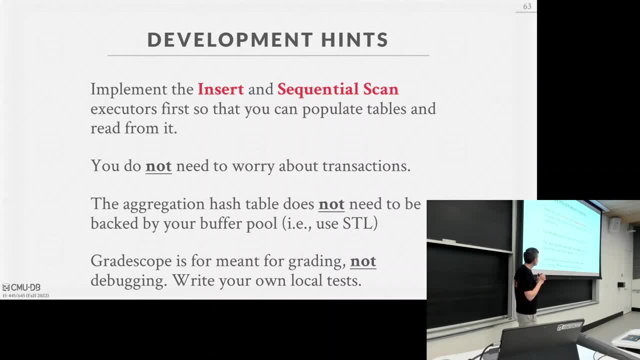 But I recommend you start with insert and sequential scan. All right, You do not need to worry about transactions just yet. All the things we talked about today. don't worry about that. The aggregation and sorting do not need to be backed by the buffer pool. 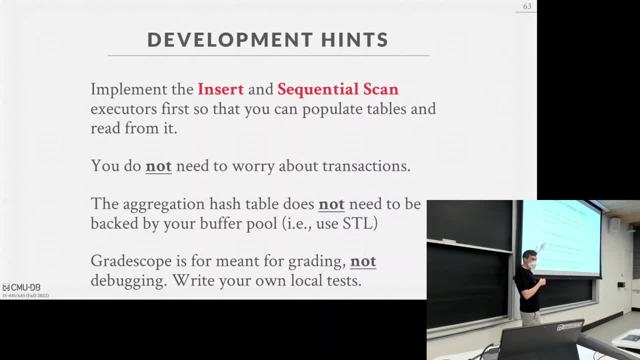 You don't need an external merge sort. You don't need to have your hash table to spell a disk, Assume that everything fits in memory and you can use the standard template library functions for these things. And again, of course, Gradescope is not meant for grading. 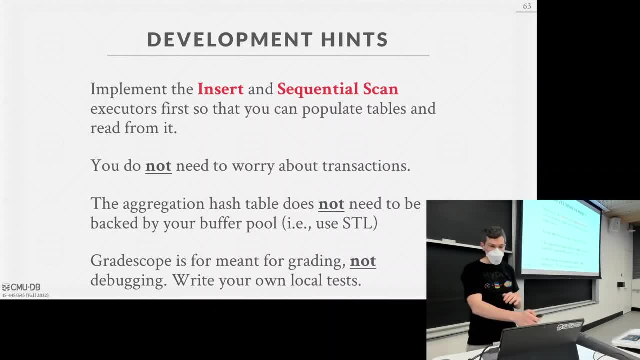 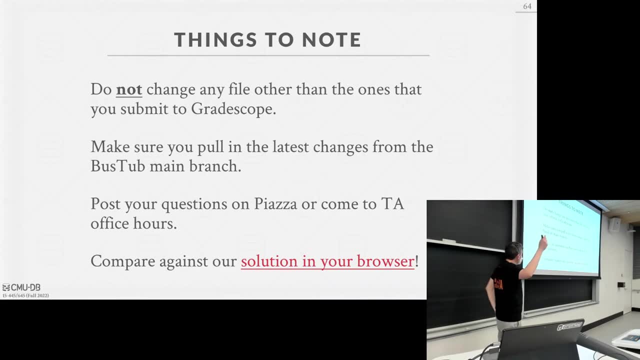 Or, sorry, not meant for debugging. Write your own little test. All right, So you're not changing the files that you did, the ones you submitted on Gradescope. Make sure you pull the latest changes from us, Of course. post on Piazza and come to office hours. 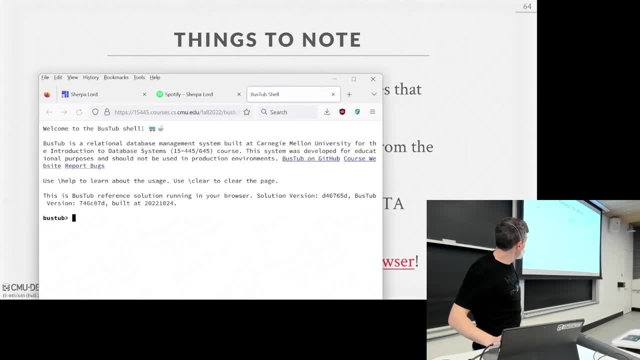 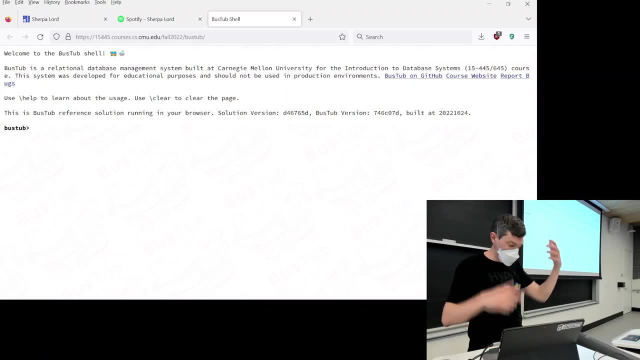 But the one thing we have this time for you guys which is super, super exciting is there is now a browser version of Busstub. He used Emscript to convert the C++ code into JavaScript- JavaScript- So you can run queries. 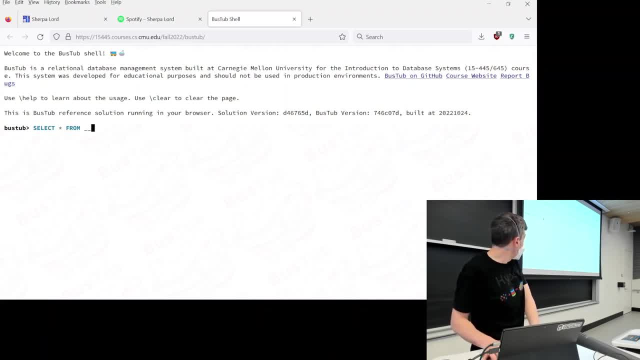 I'm going to forget. Is Project 3 already done on it? This is Project 3 is already done on it, Including the optimized stuff That I don't know. But you can create tables, Did I? No, Did she? 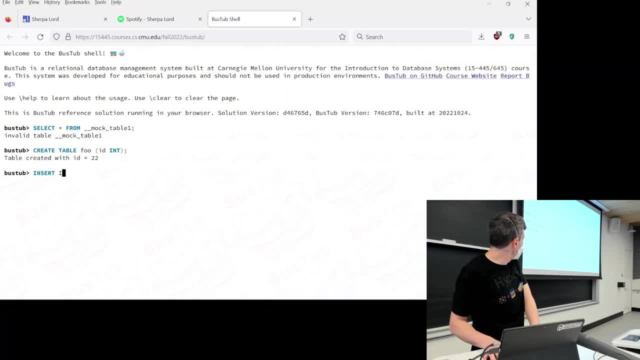 Yes, Mm-hmm. Insert into Sorry, Why would you do that? question of why is it called Busstub? The question is: why is it called Busstub? Yes, So you get a row select star from foo and you get it back.